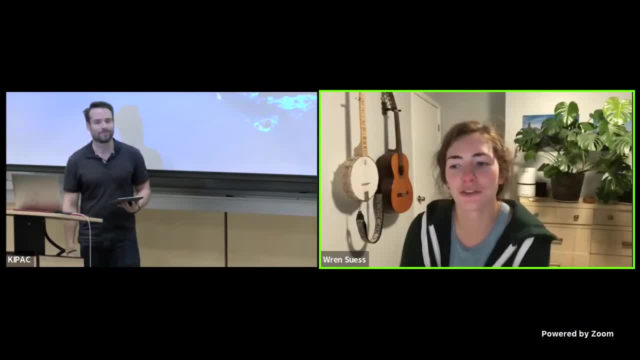 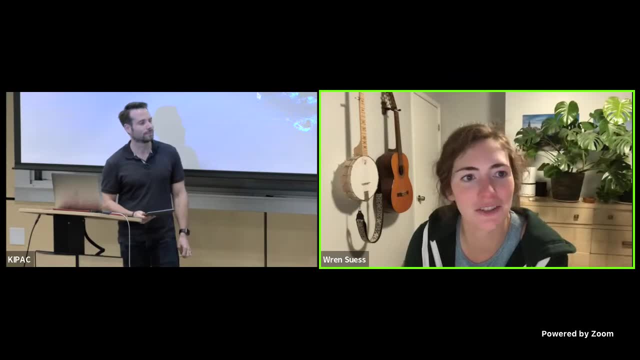 Hi everyone. I'm Ren Seas. I'm a joint fellow at KIPAC and UC Santa Cruz. I study the formation and evolution of distant galaxies using JWST. I gave the last lecture, so I'm very excited to hear about cosmology tonight from Simon. Thank you, And Jelle. 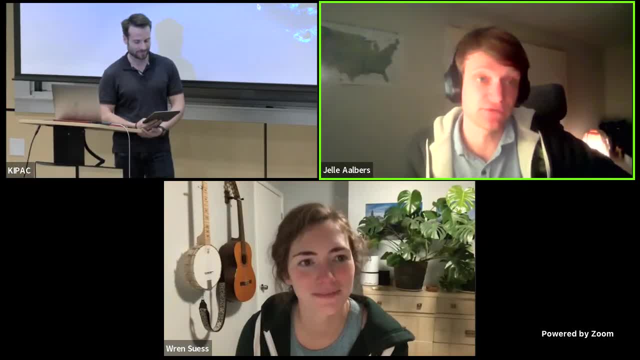 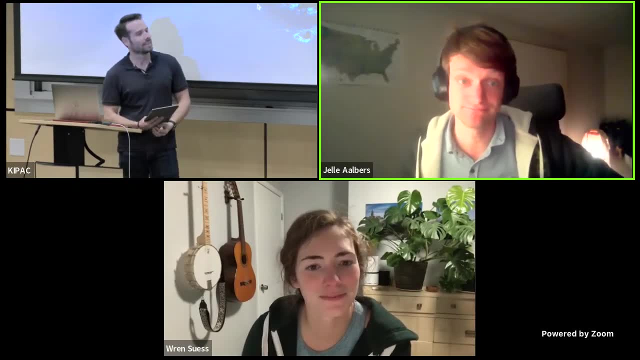 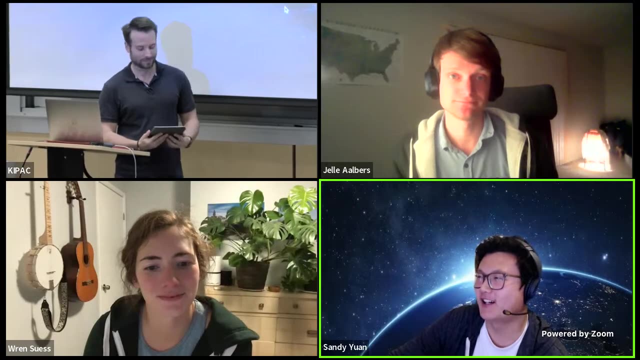 Hey all, I'm Jelle. I'm a colleague of Simon, also a postdoc at Stanford, and I work on trying to find dark matter with telescopes in space and deep underground. Excellent And Sandy. Hi everyone, I'm a research fellow here. I work on large-scale structure, the cosmic structure of the universe. 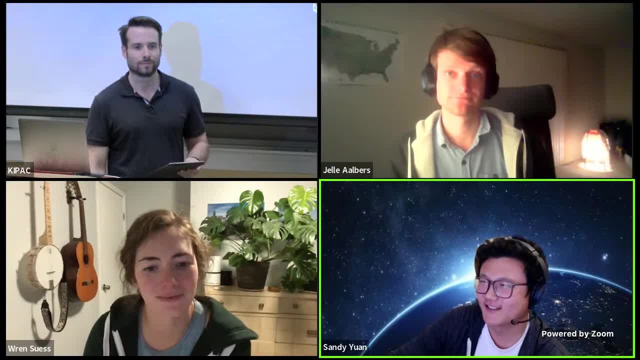 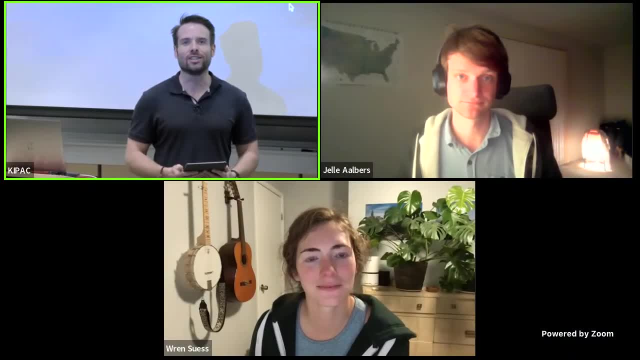 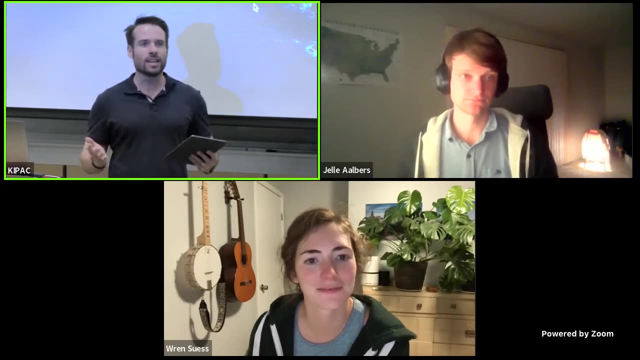 and the galaxy evolution using large simulations- Excellent. Well, thank you so much, And for those of you on YouTube, we welcome you to engage in tonight's talk via the chat window on the right hand side of your screen. In that chat window, you can post any questions you might have about. 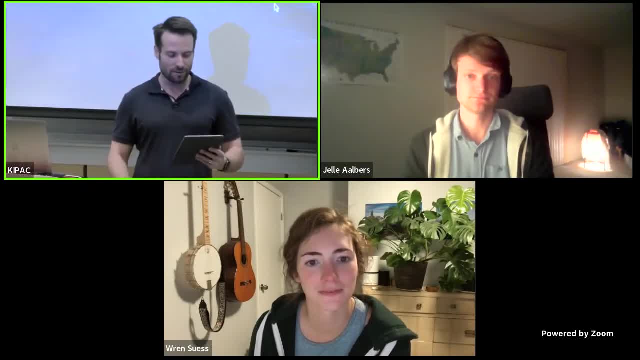 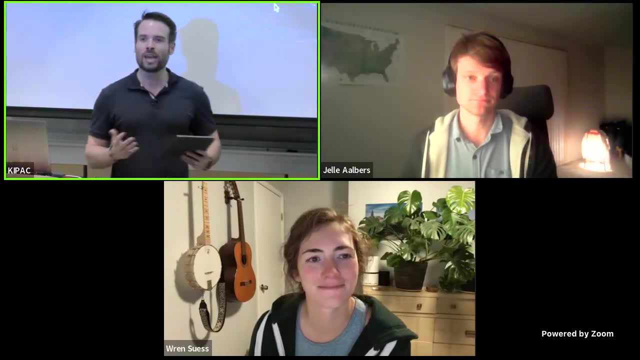 what you hear tonight, or start a discussion with some of your fellow viewers, Though we do please ask that you be respectful to others, And our expert chat moderators here will be able to help answer some of your questions as they come up, But those of you in the room fear not. 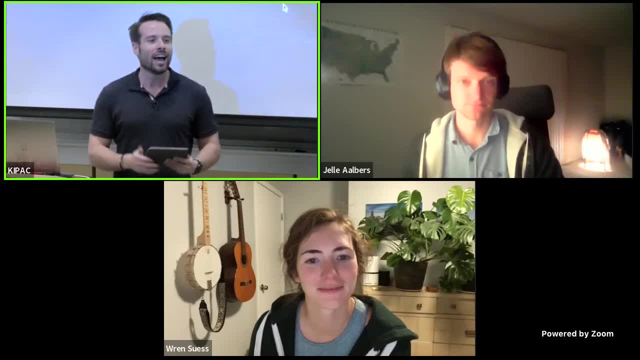 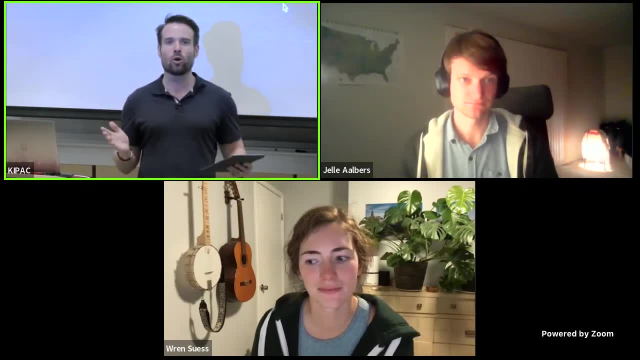 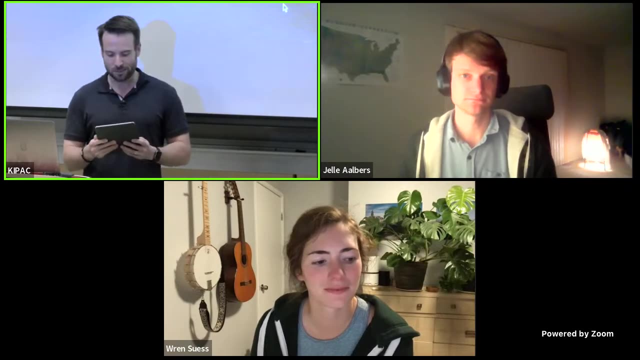 you will have an opportunity to ask questions as well. After the talk concludes, we will have a live Q&A with Simon up on the stage, when we'll be able to put some of your questions and some of the questions from the online audience straight to him. So, without further ado, let me introduce. 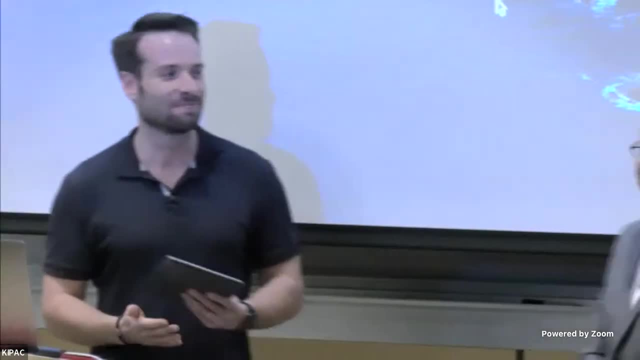 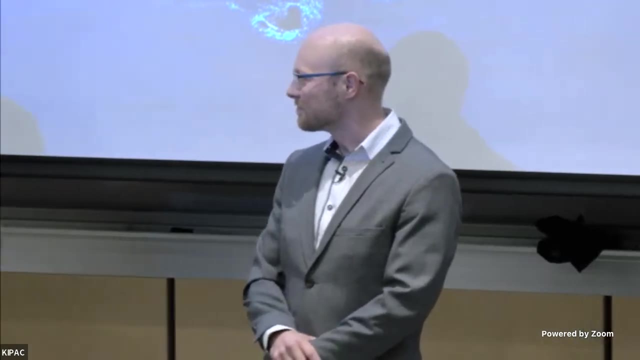 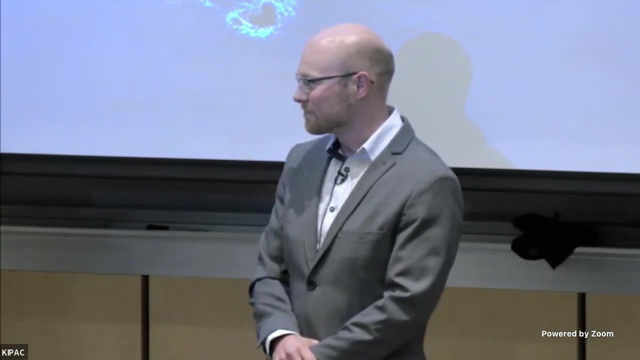 tonight's speaker, Dr Simon Birra. Now Simon is a Kavli Postdoctoral Fellow here at KIPAC and his research is all about probing the fundamental physics of our universe on the largest cosmological scales, in particular using the phenomenon of gravitational. 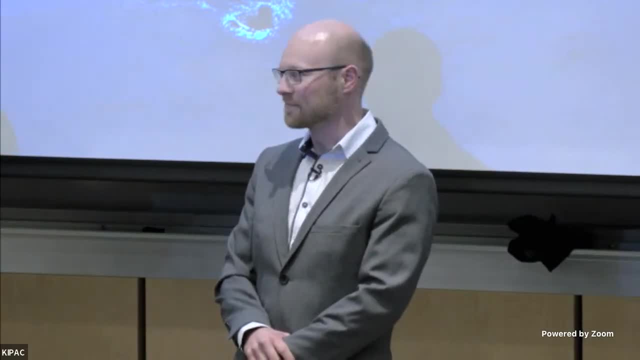 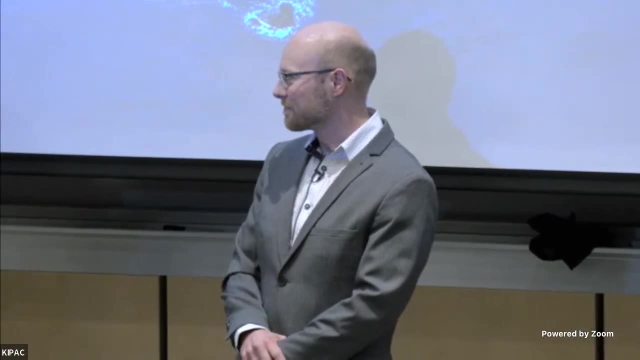 lensing, looking at how material in our universe, in particular the structure of dark matter in the universe, can be used to measure the size of the universe. And he's going to be talking about, in our universe, Ben's light. as that light travels towards us, Simon is involved, actually. 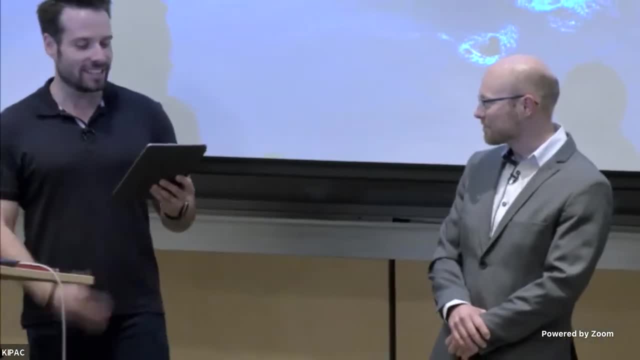 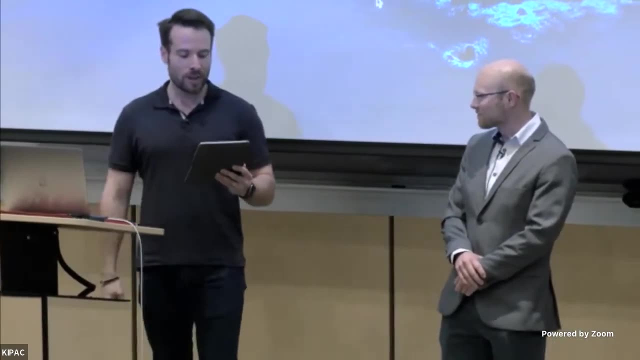 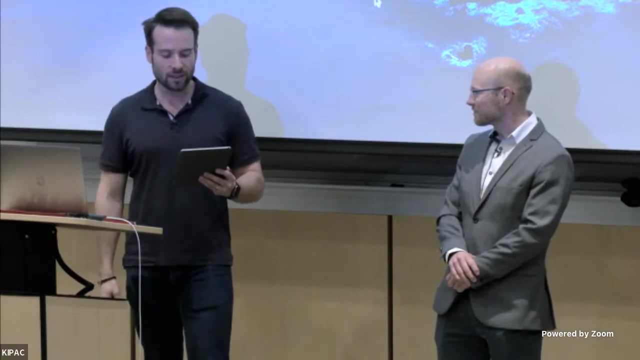 in several JWST programs. So we're really delighted to have him here tonight to tell you firsthand all about the amazing new science that he's been doing. He received his PhD and his undergraduate education from ETH in Zurich, Switzerland, And before coming to Stanford. 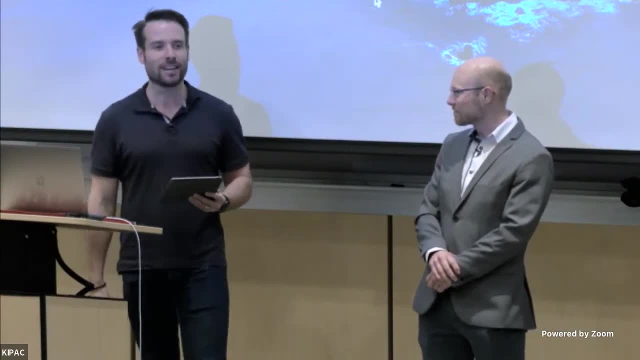 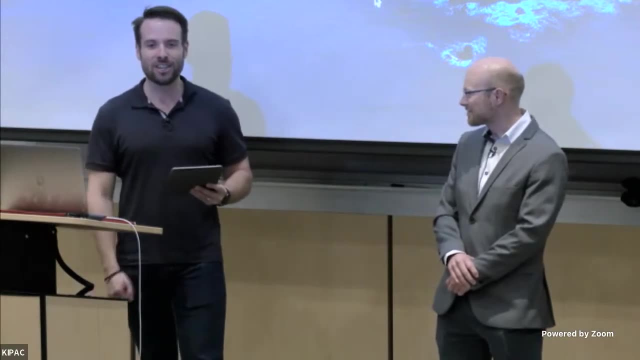 he was a postdoctoral scholar at the University of California, Los Angeles, And I'm sorry to say that Simon's actually going to be leaving us very shortly. He's moving to a new position as an assistant professor at Stony Brook University in New York. 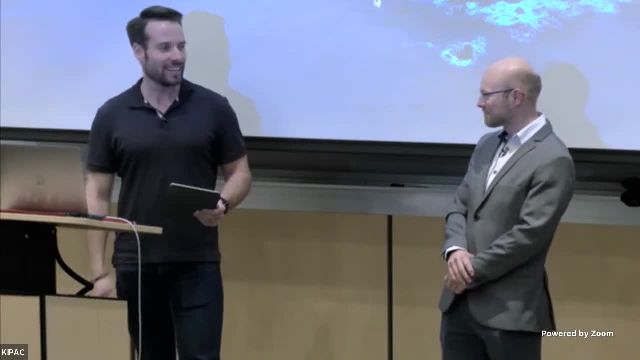 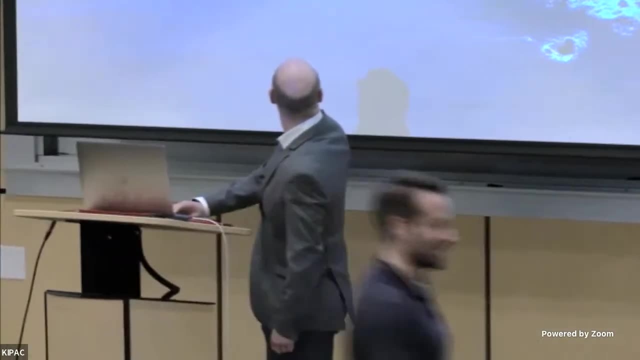 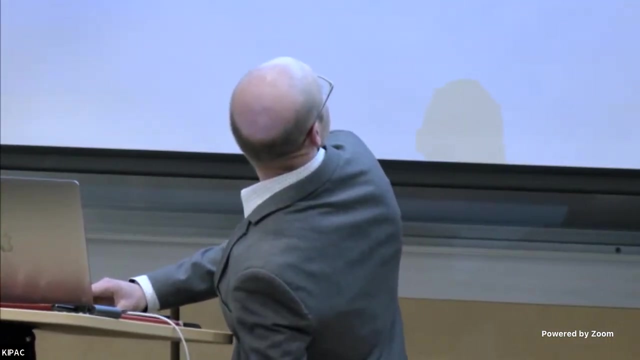 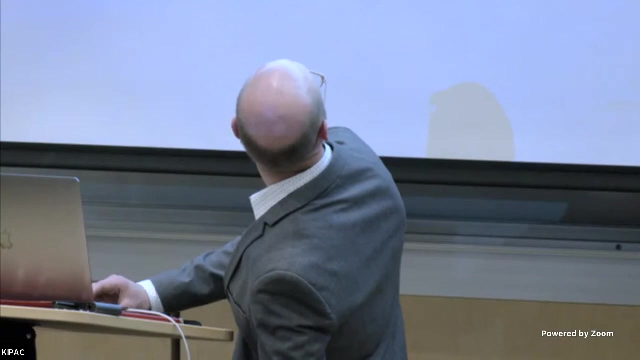 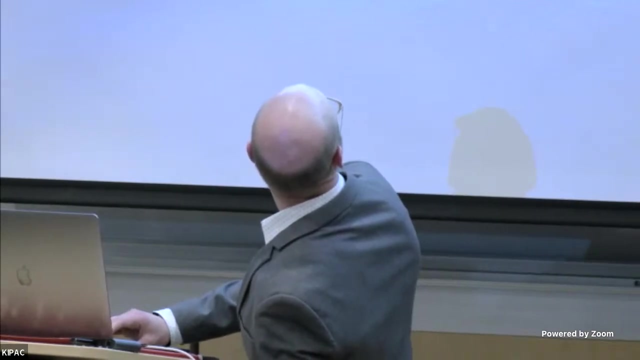 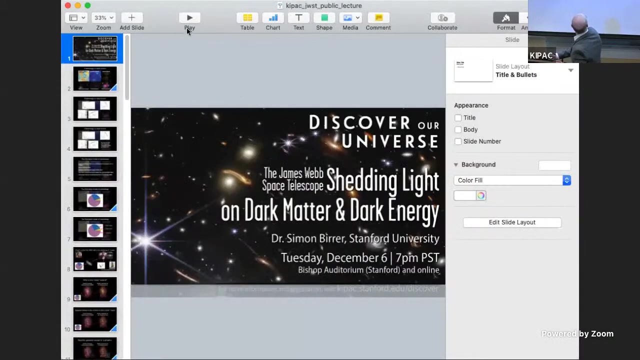 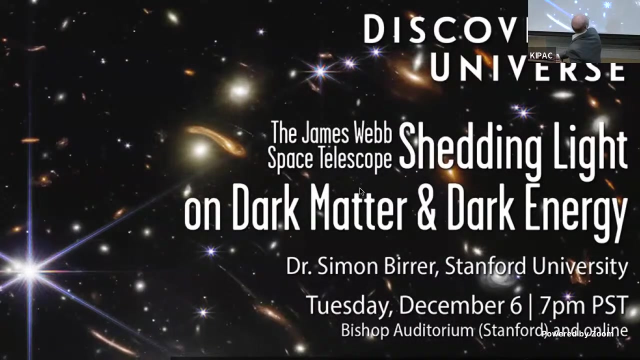 But it's a real pleasure that we could get him to speak to you tonight before he leaves. So, without further ado, Simon, take it away. Thank you so much. Oh, wonderful, Wonderful. Thank you. Thank you, Wonderful, It's a great pleasure to be here. Welcome everyone. Today I would like to talk about 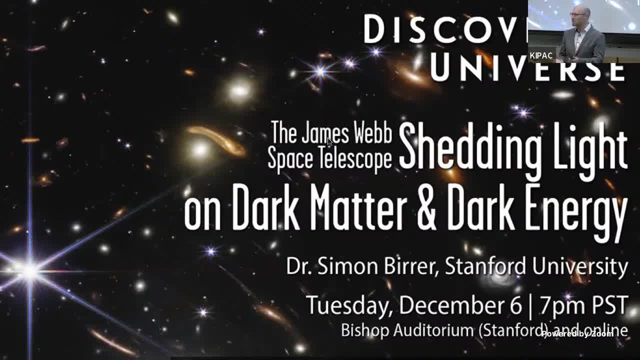 the history of the universe, what it's made of and, most importantly, what we don't know of it. And I can already tell you: it's a lot that we don't know, And that's why, in particular, we are so excited to having a new tool in space, the JWST, that hopefully 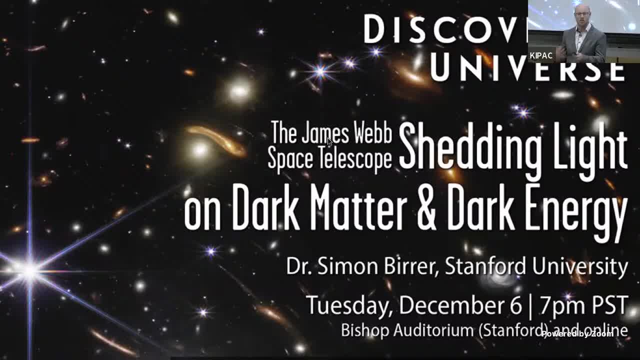 and we hope, and that it helps us guide us to a better understanding of the history of the universe and our place in the universe. this talk is titled shedding light on dark matter and dark energy, two phrases you may or may not have heard used as buzzwords floating around. 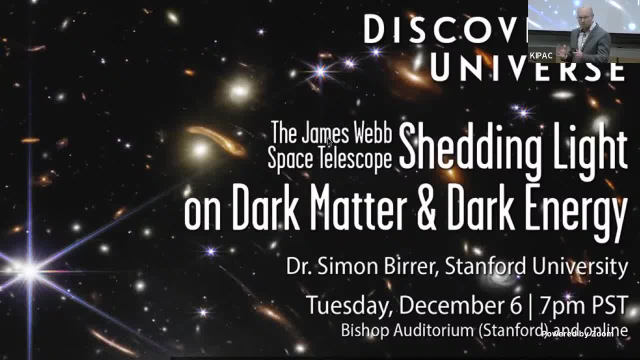 in short, they stand for. i don't know and i don't know, but i would, during this talks, i go through what we actually know about it, where we stand right now, why we are struggling, and i'll going to showcase a few experiments we are conducting with the jwst that helps us further guide in a direction of our understanding. 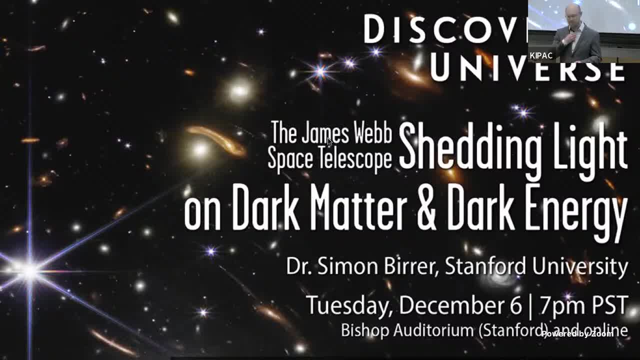 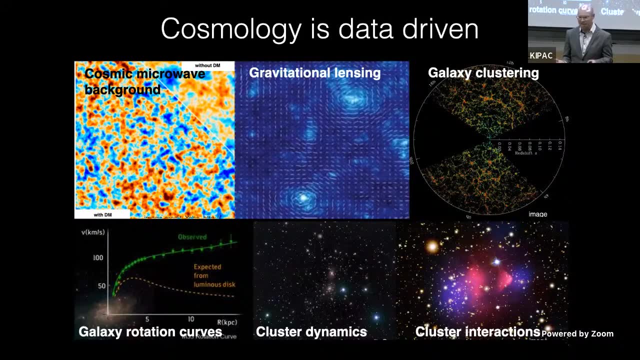 you're getting a bit of sound echo. you're getting a bit of sound echo. the reason i can stay here in front of you and be semi-confident talking about our universe is not because we have great thoughts necessary about the universe, but it's because there are decades-long tedious experiments that we measured and mapped out the 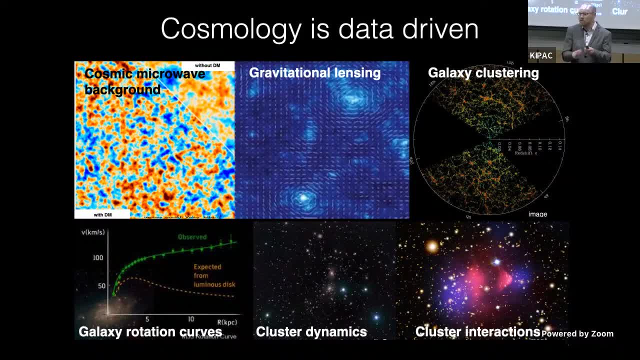 universe that helps us guide of where we are in the universe and that's why i can give this lecture here, telling us- or i'm certainly not fully convinced of what i'm saying is true, but i have a good background and story to tell you from that data. so cosmology, this is what 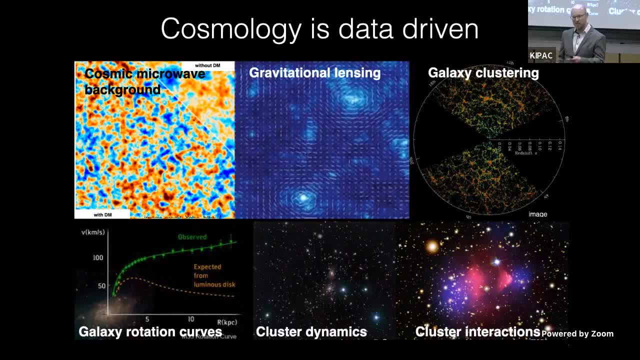 it is a physics discipline and empirical disciplines about the largest scales about the universe. it's not about our planets, it's not about our solar system. it's about what galaxies, uh do, how. it's how the largest scales in the universe that we can span and can see and visualize. 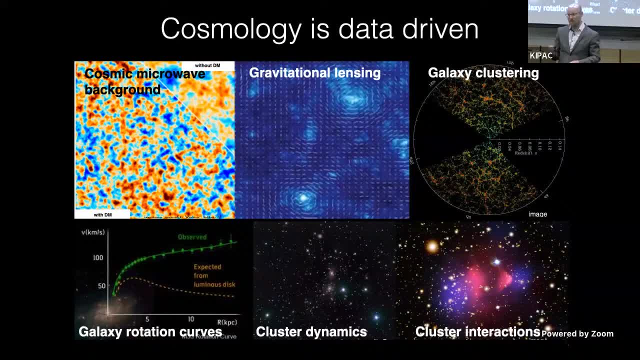 that is cosmology, and this is a data-driven uh subject, and what you see here is a set of images from data that we've collected over the last few decades that spans from galaxy rotation curves of individual galaxies to the dynamics of clusters of several hundreds of galaxies, how they 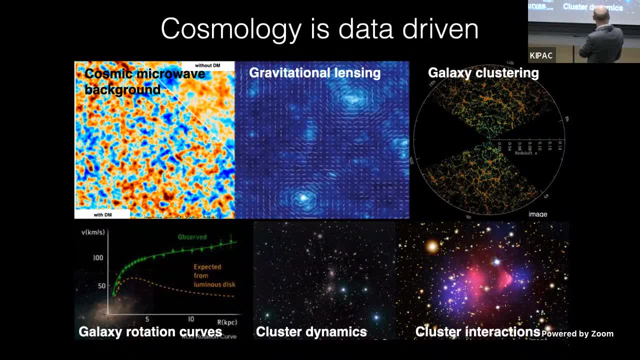 interact and how they flow through each other, to how clusters uh collide and what the gas is doing, for example. but then we can go even further out and take a bigger picture, say like how do galaxies cluster in the universe? and we see here like kind of like a spider web of galaxies. 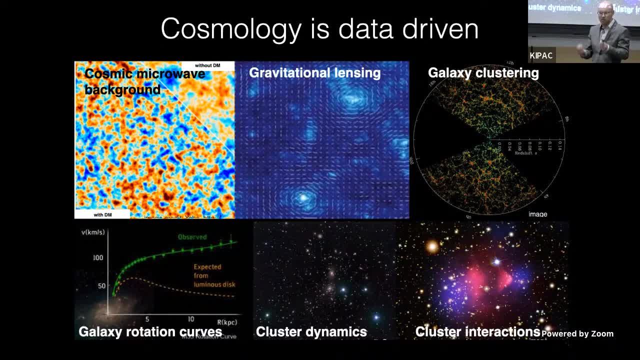 how they are clumped, how granular the structure we find to see in the universe. two, and this is what i'm going to talk a bit later: light is being bent and we can see this shearing and distortion effects in the universe on the very largest scales and we can map the matter: distribution of the universe over a large 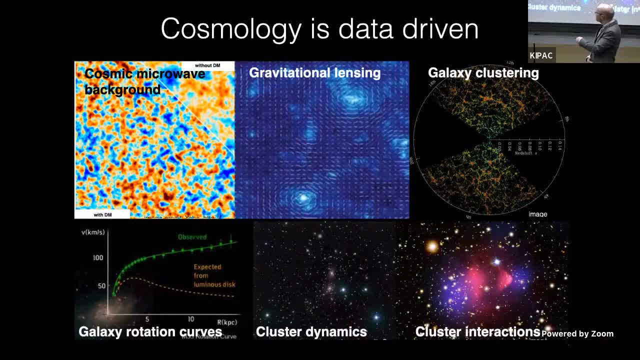 scales and epochs. and, last but not least, the cosmic microwave background, the afterglow of the big bang, the radiation of a hot plasma that has been emitted billions of years ago and that reaches us now rather cold, as a background noise. and all these observations together, and even more that i'm going to show. 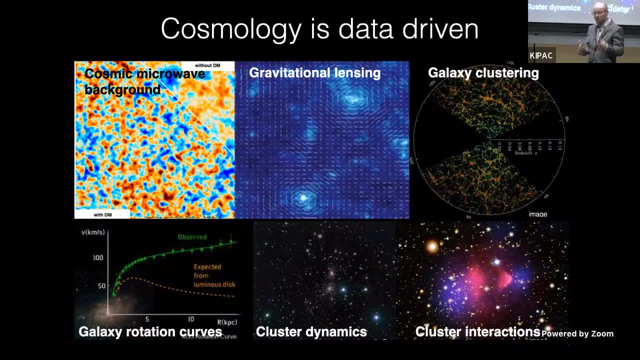 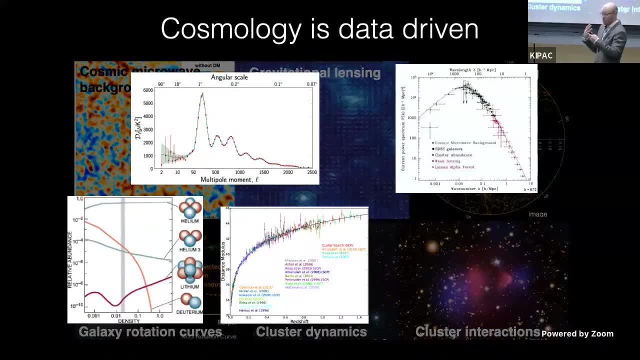 leads us to a rather consistent picture of how we think the universe has evolved through cosmic time. and what i show you here is not the pretty picture of the visualization of the data, but it's actually what we compare of that data with our models. and so, just as an example here, 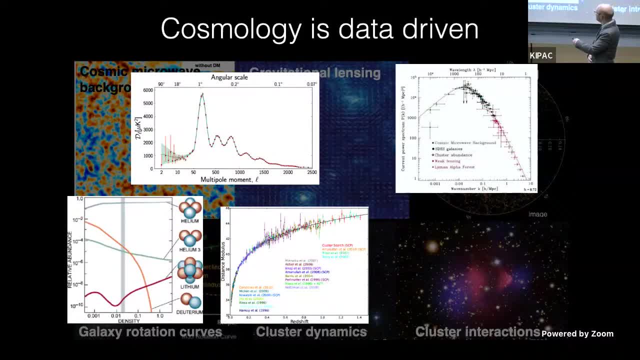 this is the cosmic microwave background in a space that is not really important, but the data points here describes the statistics of the patterns that we see imprinted, and this line going through the middle is a model, and so we have at least one model that describes that data. 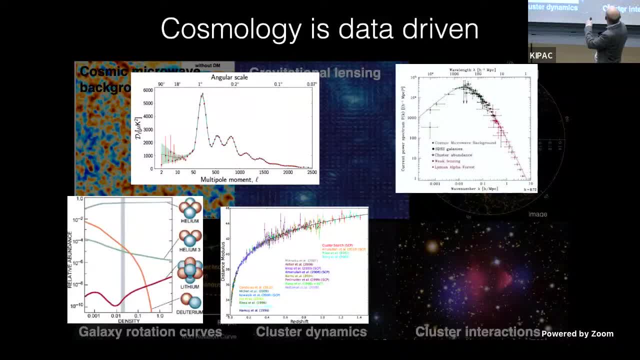 remarkably well, and so for other observations of galaxy clusters, and here a line through is a model expands- i come to that later- and the black line fluid and this is a model- and it's always the same model- that describes all this data together and this is a remarkable success. 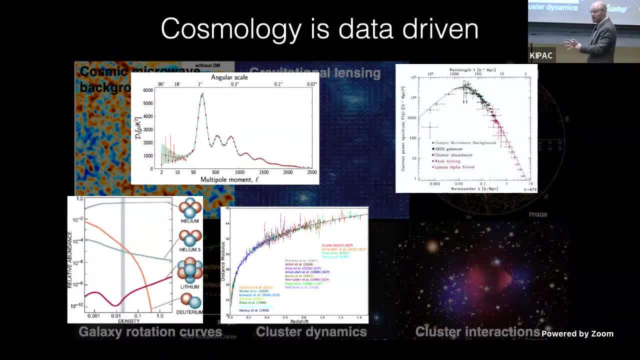 of cosmology, that we have the ability to describe the data. so we have at least one model that is excellent in describing this data that we have collected. that doesn't mean this is the correct one, but we at least have come to the point where we have the data which уч candlesнять moonlight huge. 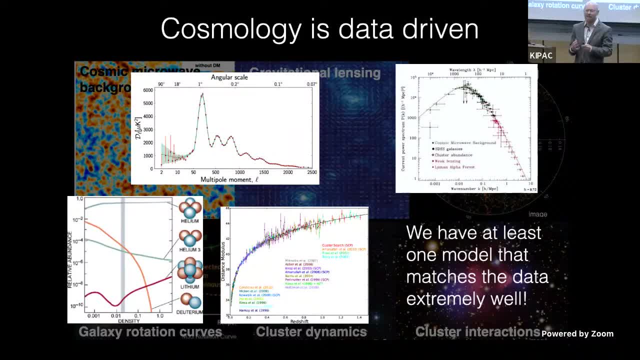 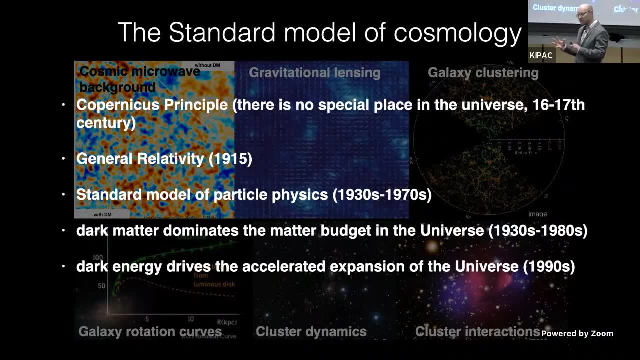 have such a model, and what does this model entail? and here the struggle starts. the first- and this is, i feel, the most fundamental, but it's often for forgotten a bit- is the copernicus principle: there is no special place in the universe, whether it's here on earth and solar system, our milky way, nor everywhere. so wherever we look and wherever, 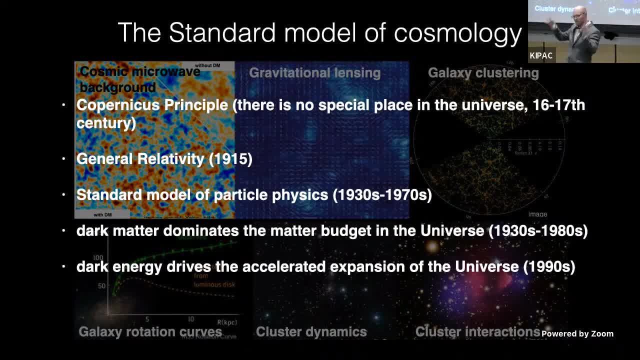 we see things happening. they're self-similar. there's nothing more important why we are here or somewhere else in the universe. that's the copernicus principle, and i put here also that this comes from 16th, 17th century. the second pillar is general relativity, our current 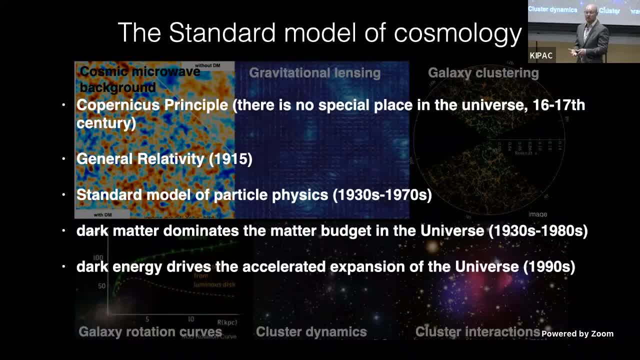 theory of gravity, how gravity works in a universe on the largest, two very small scales. as we stand here and getting uh hold on on the ground, the third pillar, not so much as a price, the standard model of particle physics, that's what we are made of uh. this has been effectively uh completed to that level and in about the 1970s. 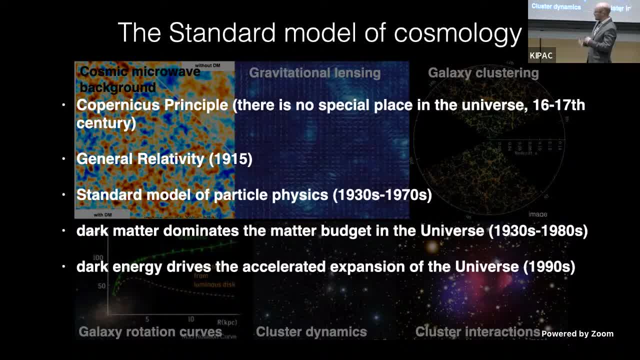 to the stand we are now, and so- and this is how particles, how the stars, shine, is very well described within this model. so we wish we were complete with these pillars, but no, there's this thing that we call dark matter, which dominates the entire matter. budget in the universe. 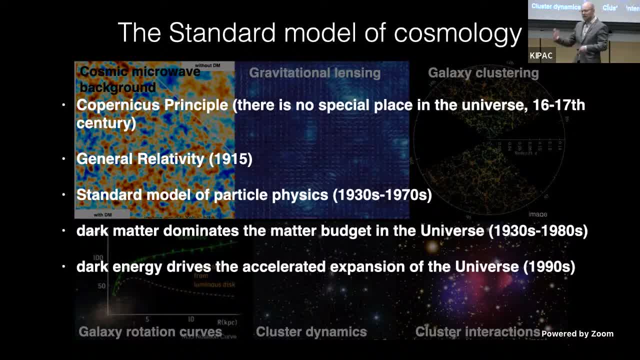 first sign came around in the 30s, and it got more and more accepted around the 1980s, when the term may have appeared more frequently in textbooks. let's speak that way. and then, last but not least, dark energy, which is a placeholder that describes the accelerated expansion in the universe, and only 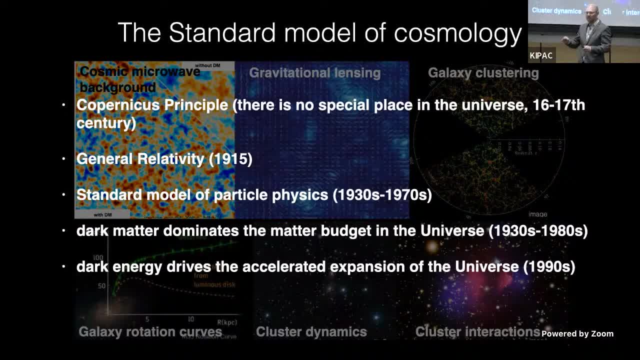 detailed observations in the 90s have indicated in the really early 2000s they've nailed it. we need this, additional components to it, and the reason i talk about dark matter and dark energy is not because it's some fancy terms, it's actually we. we need something to describe this wealth of data. and when we now look at the 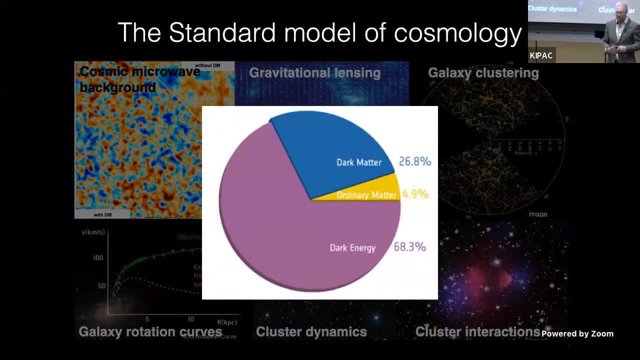 composition of the universe. uh, we can make a pie charge and this is what currently we think our best guess what the universe is made of right now is is 4.9 or 5 ish percent is the ordinary matter that we know that are described by the universe and the universe is made of right now. 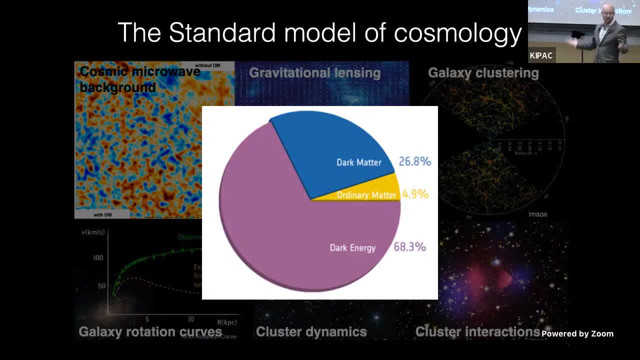 the standard model of particle physics. here, what, what we are all made of about five times more- is in the form of what we call dark matter, which is unknown. it's transparent. we don't see it, we don't taste it, we don't smell it, but we know it interacts gravitationally to. 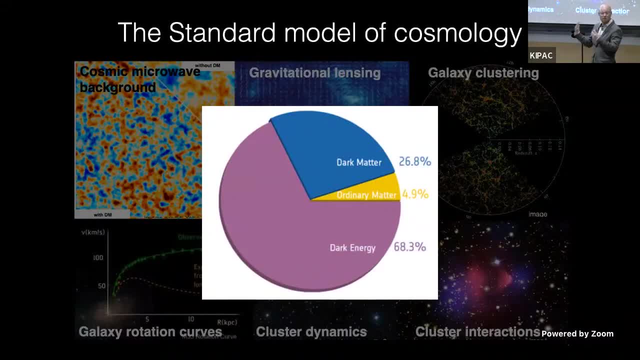 make up the universe, as to be able to describe the universe as we see it, and then this very large component is what we call dark matter, and dark matter is a very large component of the universe: dark energy, which is responsible for the accelerated expansion of the universe. 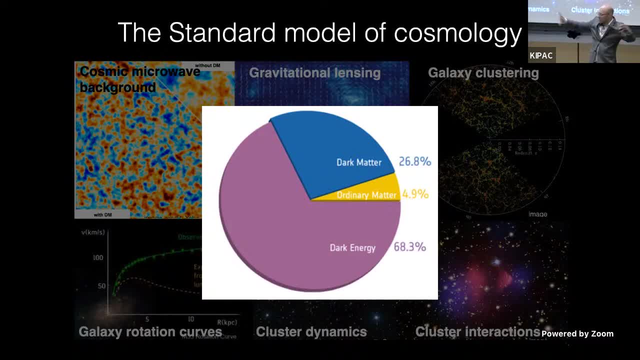 a negative pressure that pulls uh objects or galaxies away from each other and, over the long terms, leads to an accelerated uh expansion of the universe. and so, if i look on this, um, still, after years, almost a decade that i'm in this field, since i started my phd, i still think like that. 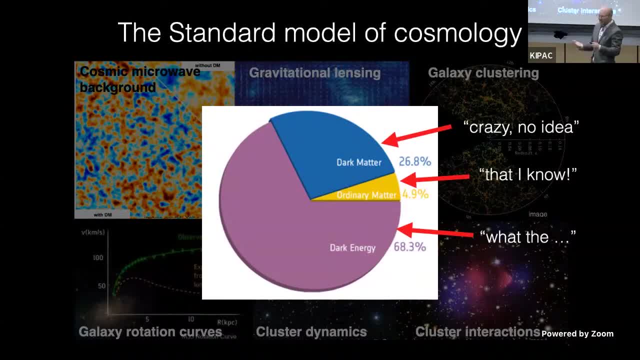 that thing, i know i'm kind of like familiar and some people even know it better- the particle physics that people are working on, solid state physics, etc. then dark matter- crazy, no idea. well, there are some ideas and i value all these ideas and some are actually quite nice ideas, but we don't really know whether 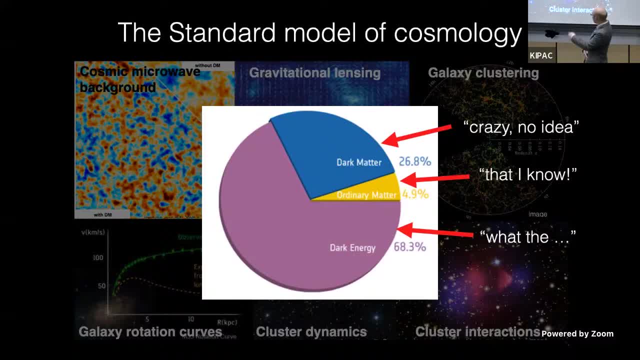 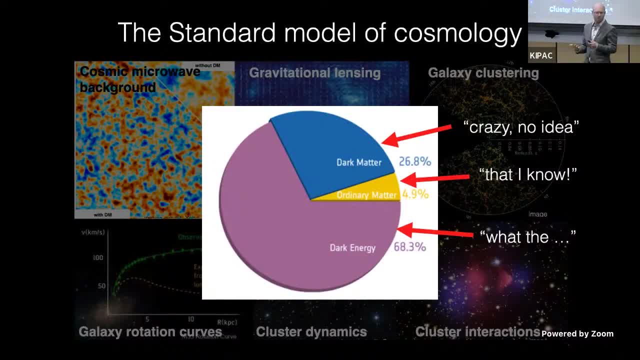 or may not be, but which one is the right one, we don't know. and before going now a bit deeper into the dark matter and dark energy story, this seemingly small part is actually what we can see in the universe right now: the galaxies and every data that i showed you effectively relied on. 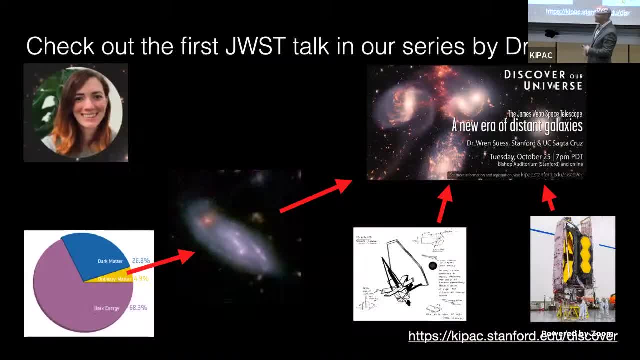 something that we see and observe, and i would like to highlight here the talk by dr ren sis, who gave the first public lecture in the jwst series about the distant galaxies, where she describes, yeah, what this portion is made of, these beautiful galaxies are made of, and she also lays out a bit 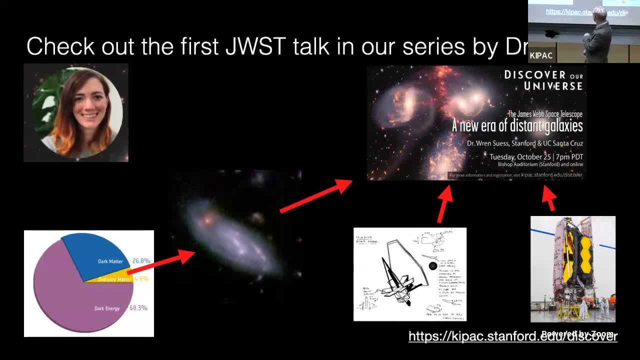 a story in the history about the jwst, how it's being built, launched and what amazing capabilities they have. so i invite you very much, go and watch it. if you're on youtube, you see, on the same channel, this lecture being present there and, without further ado, let me dive a bit into the first part. 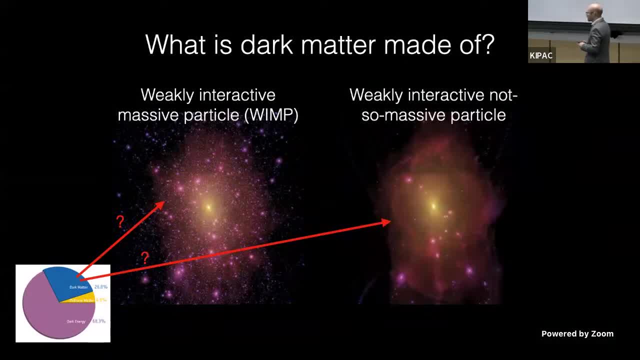 of dark matter, even though we don't know what it is. we can hypothesize what it is and we can run it in a computer to see what will it predict? what emerge, what structure merge, and we can put this in our computers and what happens is that, over time, 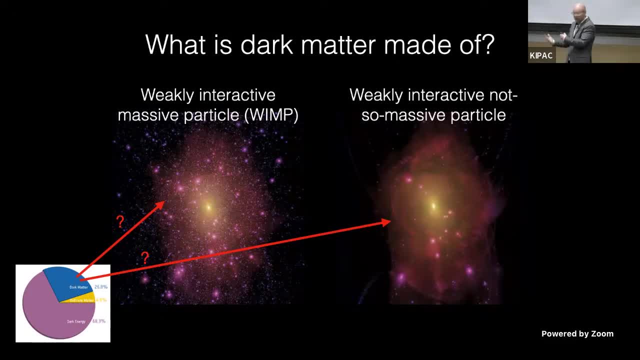 when gravity, we let gravity do its, it's, it's thing, gr. basically, we see such structure emerged of collapsed structure bound together that is slightly fragmented. so gravity is a attractive force, and so where there's more matter, it attracts even more and and so and it leads to something like: a visual structure, and then it's even more fiber, but then it's even more and then it's even more like aSparkle infrastructure that is falling forward in and causing many different contrasts. and homes, farms, where undisificación, oh, head relationship, mental Soup or gravitas have bends over there. all of that and that goes on, and so far. 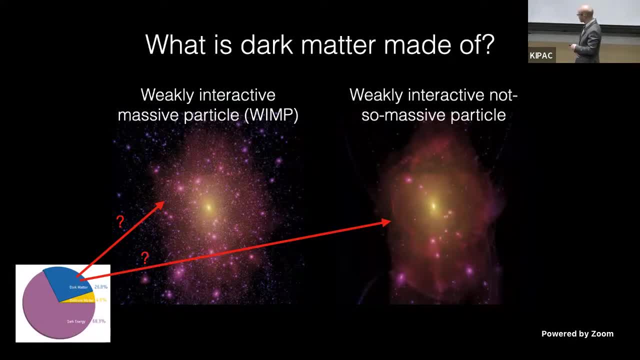 of structure together, what we call a halo. what we don't know is. but here we can either say dark matter is of this kind of weakly interactive massive particle, which is here on my right, or weakly interactive but not so massive particle that damps a bit the structure on the smallest. 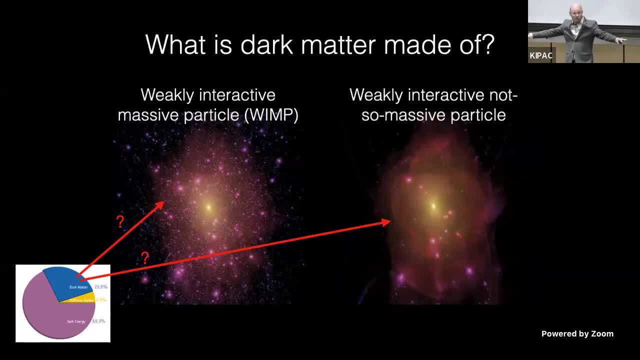 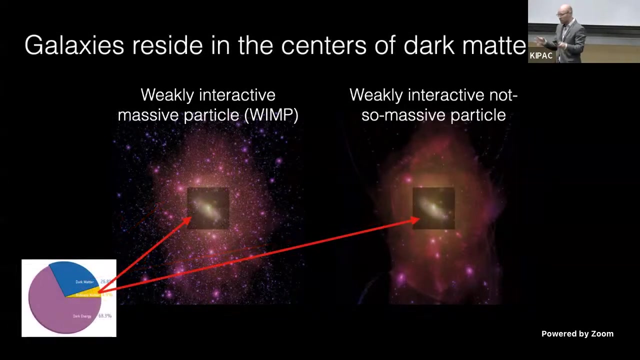 scale. so we let it first like rinse away like water before we let this little wave scroll back and gravity uh pulls things together. so there are two hypotheses likely. none of them is exactly the truth, but there are two uh models that we have. what we know exists is in the very center of this. 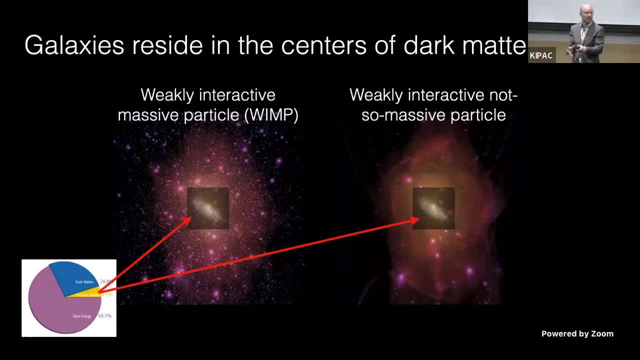 collapsed dark matter structure, resides the galaxies, resides a milky way, resides the galaxy that's seen, we see in the very early universe and basically every galaxy we see around us. and we need this massive dark matter structure around it such that even galaxy can form. we need this potential way of attracting force such that gas can cool down within there. 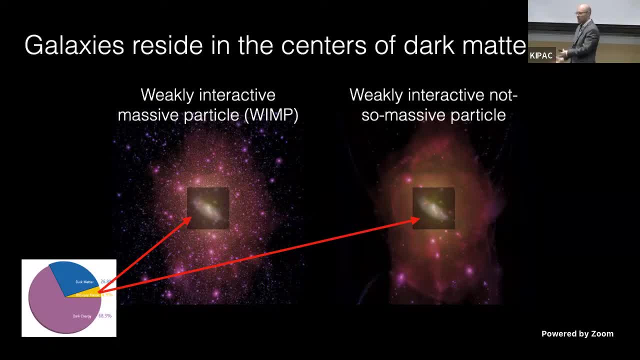 and form the stars. so, without dark matter, no galaxies. it sounds contrary, but in that sense it's required to form the structure we see. so can be in both of these scenarios, as an example, what we also know, and this is interesting- this has been, these models have been. 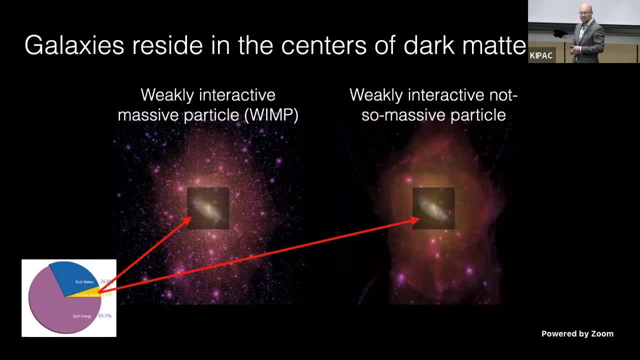 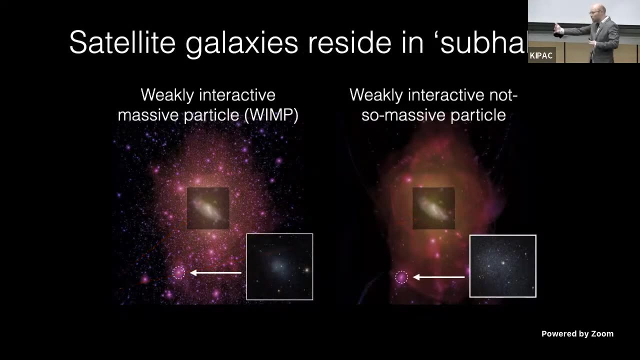 around since, like the early 2000s, by then we haven't seen very small galaxies, but we predict that there is a lot of clumps here, or potentially a lot of clumps around us, and indeed then in the early 2000s, with surveys that monitor diligently the skies, 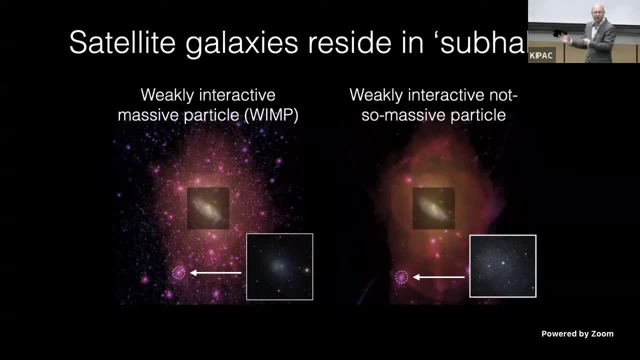 we discovered this ultra faint. we call them dwarf galaxy, so companion galaxies around our milky way, and we know they they reside into some matter structure that is dark, so dark matter, and so we can assign these little galaxies to this small structure residing around the bigger ones. and this 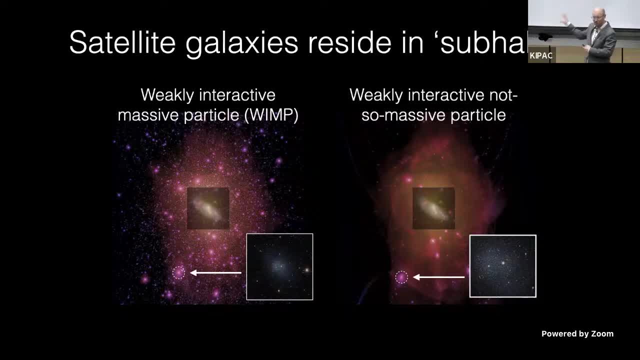 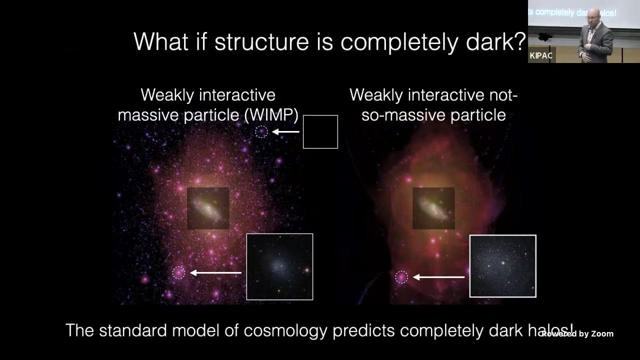 is a remarkable prediction has been made before. we actually saw and searched systematically for these very faint, very tediously to find very good, well hidden in the sky objects. so they match for both. but then we start counting. here it's like: well, what this dark matter model predicts is very small clumps that are depleted of stars. there's nothing in there. 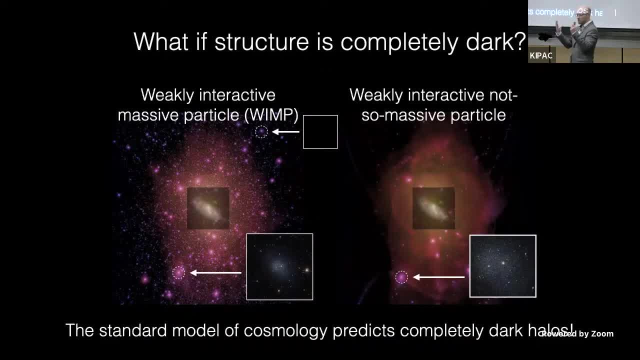 except dark matter or nothing that we can see by eye, that stars would would shine, and this is a fundamental prediction of our current model of cosmology, where i show you the nice lines going through there, which we don't know whether it's true, but we have predictions of what may be out. 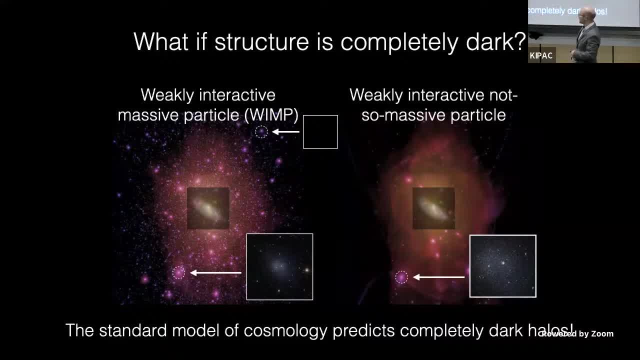 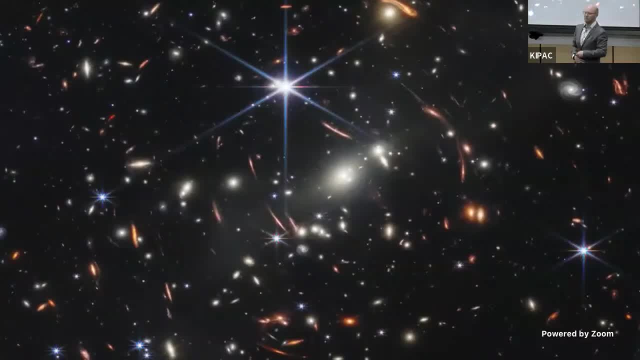 there, but we don't know whether or not it's. it's being present, and this lets me now to the james webb space telescope, and this is the first picture that has been released by by nasa. it's not the first. fiction has been taken by uh. 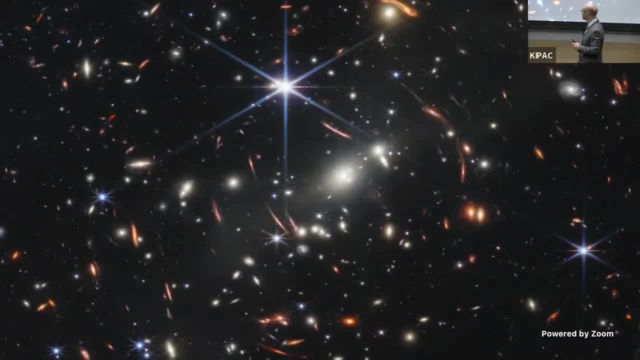 that amazing telescope, but the first picture that's been released and what you see. our first question: what? what do you see here? shout it out if you're in the audience- galaxies, stars, gravitational lensing arcs, many thing- and if you're in chat, put it in what you see, and there's a lot going on. this is i could stay or i stare of it. 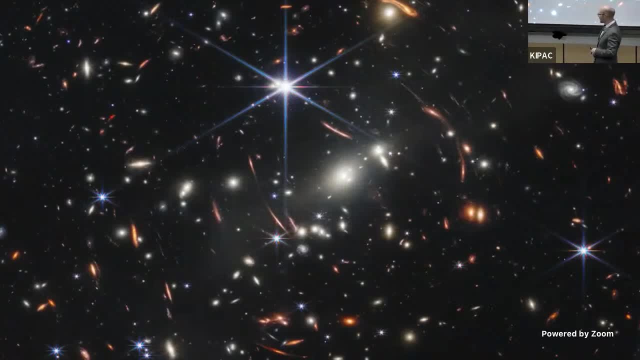 too long, i think. but that's also what drives to some degree my excitement for this field are such images. but they have so much information in there, and what, just to give you a little glance here? what you see here, this light yellow blob, is a massive galaxy. 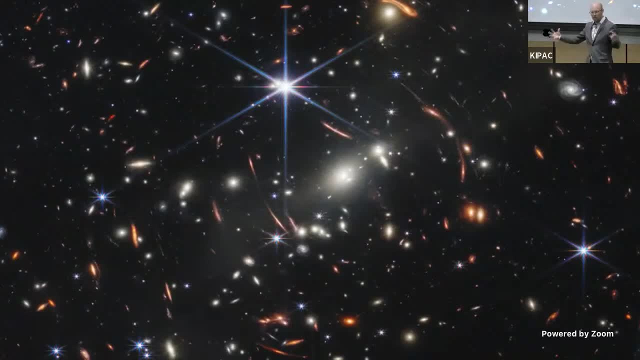 that is about a hundred times more massive than our milky way. it is in the center of a massive cluster assemble of other galaxies that are in in yellow, and this form one of the most matter accumulating objects, so to speak, in the universe. and when there is matter, mass gravity bends light. 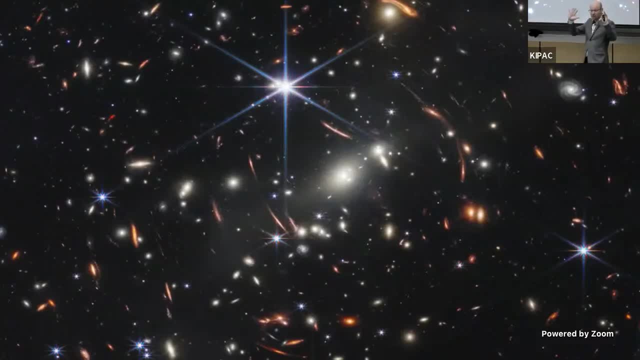 and so if there's something behind it, it gets bent around and we call it a lens, as if you have a lenses or you can take a wine glass and use it as a lens, a glass, a refractor, and it bends around objects behind. and these are these highly distorted images, and we know, we knew of them. 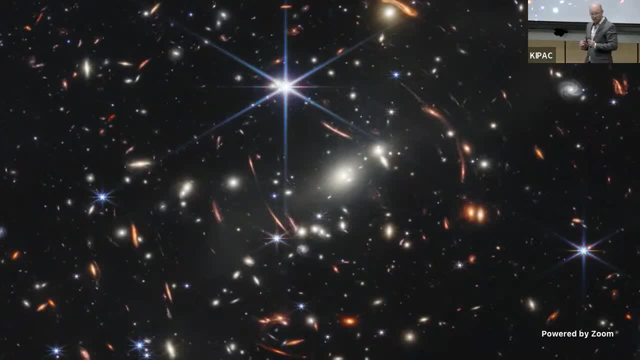 so that was not a new surprise from jwst. but jwst is so deep and so precise and when i personally looked in this image the first time, i thought, like you may or may not see these little stripes here and there, everywhere they were not. 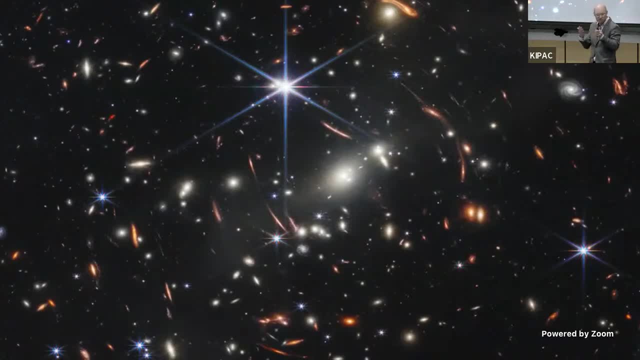 not visible before jwst and when i saw it on the screen i felt like my screen is dirty and i washed it and yes, it was dirty, but this was still there and it just showcased how much information is in the universe to be extracted if we come with 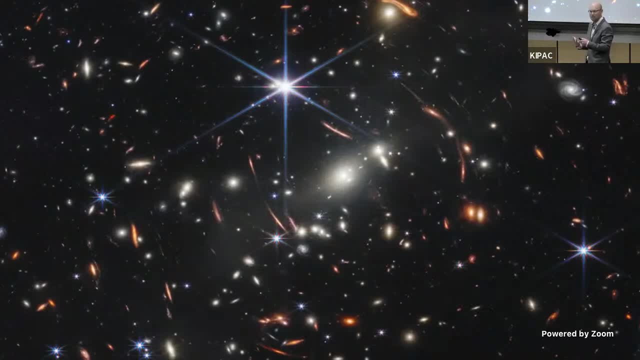 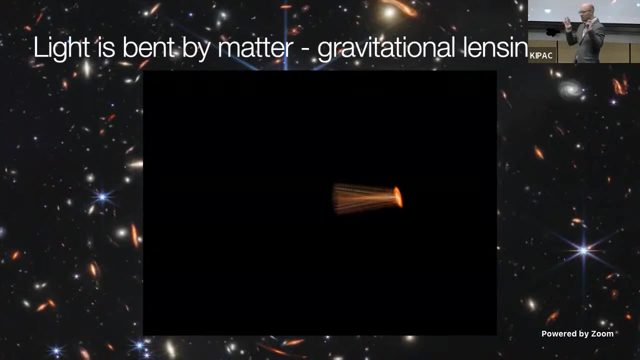 a telescope, an instrument that can really take this information to us, and jwst is such an amazing instrument that can do. speaking of gravitational lensing, here a small animation of a galaxy that emits lights in different directions, and it on the way to us, or through the universe. it gets bent around and then, depending on when we're aligned, on the 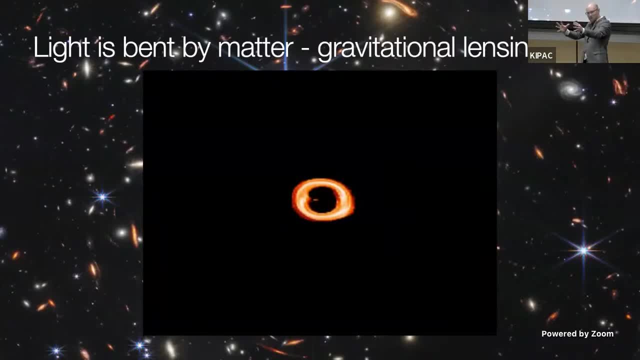 sight line that something big, a massive, is in between. we see it so highly distorted and this object here we call an einstein ring. so when you see multiple images of the same sources as a ring form, when the matter is more or less spherical, being bent to us and this phenomena can be used, 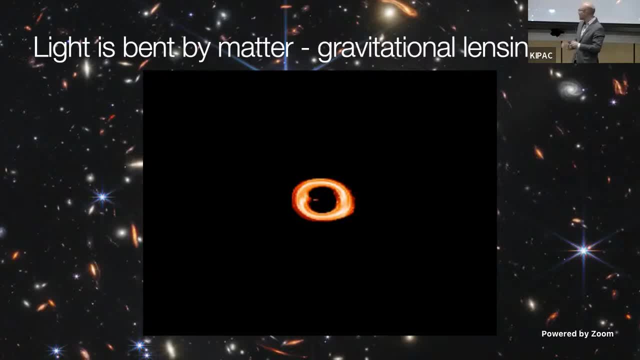 to study dark matter. no matter what the matter is, it bends light, no matter whether it's in stars, in gas or in some spurious stark matter. whatever it bends light and so we can reconstruct and see, know where it is, how much it is, how granular, how clumpy it is. and that's what the one aspect of the 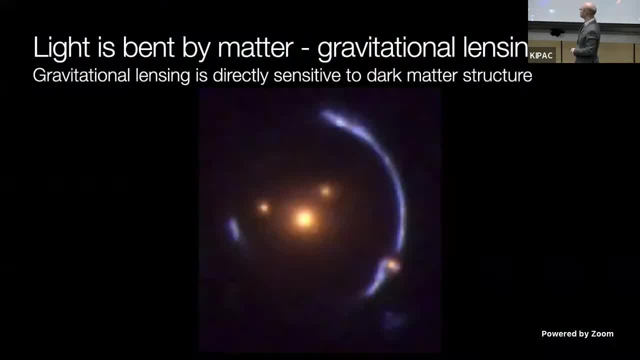 what the james webb space telescope is going to do. so here is an example from the hubble space telescope of such a phenomena, of a arc, some massive galaxy that does most of the lensing and what you see here is this little companion galaxy that does a secondary bending here. 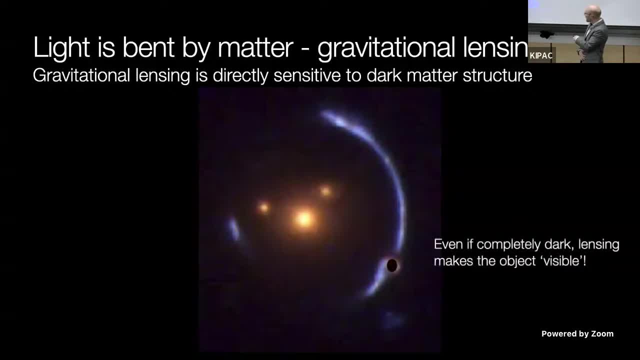 and you see, even if you were, if i wear your black out and if this thing was coming be completely dark- no stars- we would still, by just looking at what it does to the background, could pretty confidently say how much matter should be here. that makes this distortion and that 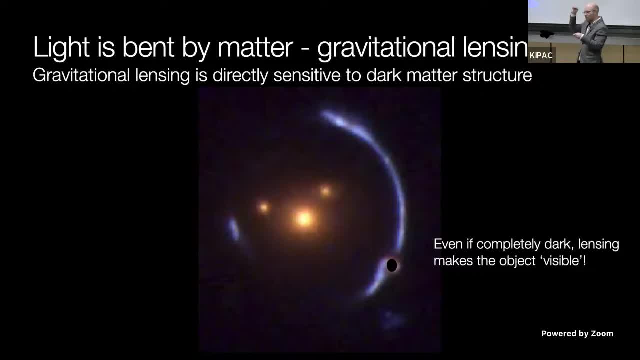 game. as we see here, this is very massive. we play further down in the range of mass, further down in how much it distorts, down to a pixel, down to a tenth of a pixel or even below, and see what are the small scale distortions are present, and that's one project. um, i'm involved with jwst, that i'm. 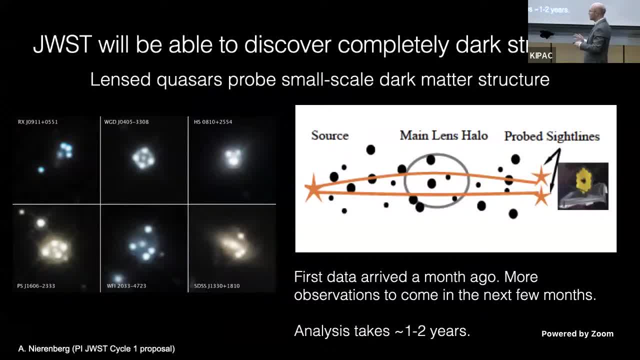 particularly excited about and the way we do it. in brief, so here um these are quadruply imaged quasars, so four images of the same source, and that source is an accreting supermassive black hole. and, as if this would be fancy enough, these four images. 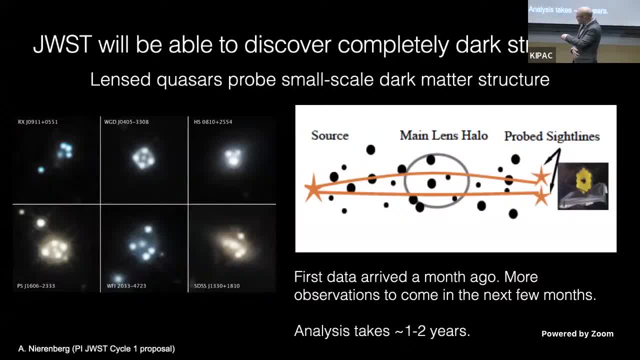 provide us with an expect, or we have an expectation of how the brightness between these images are, depending through what lensing they come to us. so we see one flux a bit more and the other image a bit less, and while this light is traveling to us, it may intervene with a lot of potentially dark. 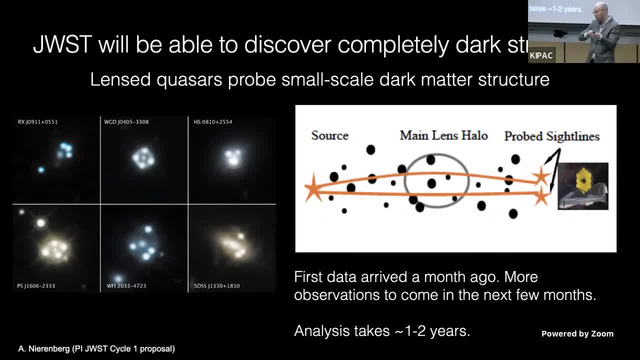 structure along the way and depending on how many of, depending on where they are and how cuspy or corey or fluffy they are, it exhibits a difference in the brightness and if, and the james webb space telescope can measure these fluxes to an incredible precise level that we cannot achieve before. 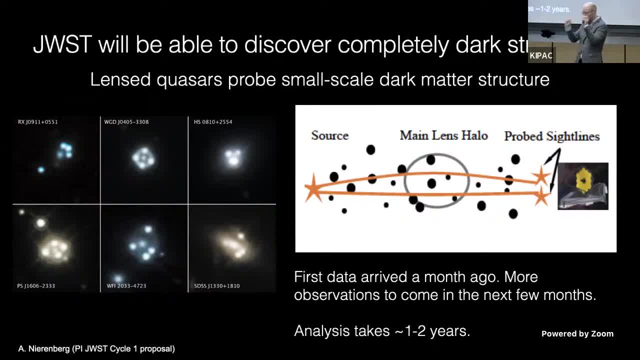 and we are able to measure very small scale distortion of these flux ratios and we can do the statistics and tell us what type of dark matter or is consistent and what type of dark matter is not consistent with the observations we have. and here this first data arrived a month ago. we are very excited. 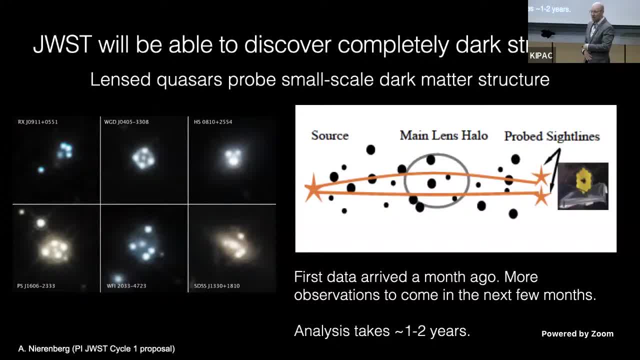 and more observation within the next few months, and we all have to learn that data products the analysis and this takes about one to two years to just run that analysis that we have now set up before the plan planned before jwst was launched and now we have a lot of work to do. 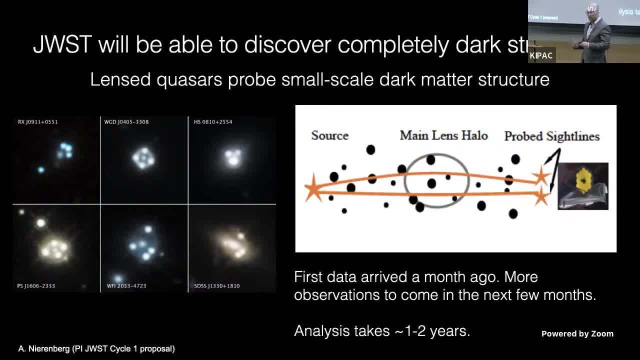 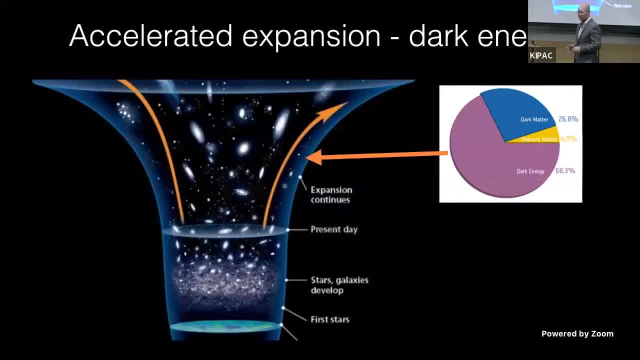 so that's one of uh, dark matter work, one project that jwst is i'm personally excited about. let's switch gears to the accelerating universe, or dark energy, the placeholder that we use to describe this phenomenon. so here we are, present day, around here, and in this kinematics, the acceleration. 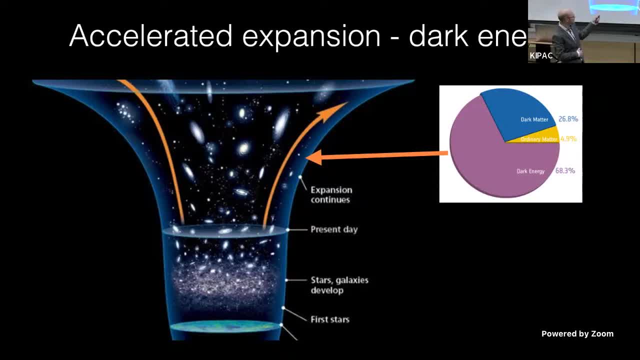 has just started this year is a protect projection of how our current best model projects, of what's going to happen and, if you're interested, what are the scenario of how our universe ends. i highly recommend you the public lecture that's by katie mack that is also on the youtube channel of kaipac. 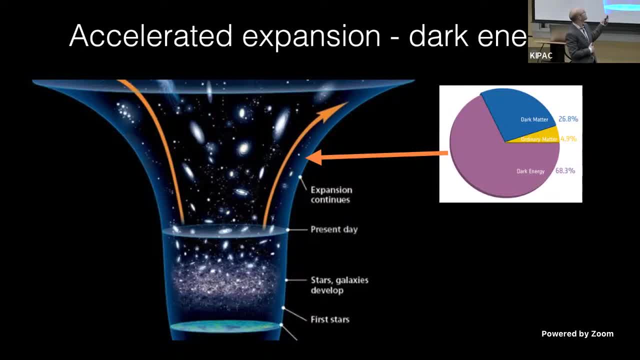 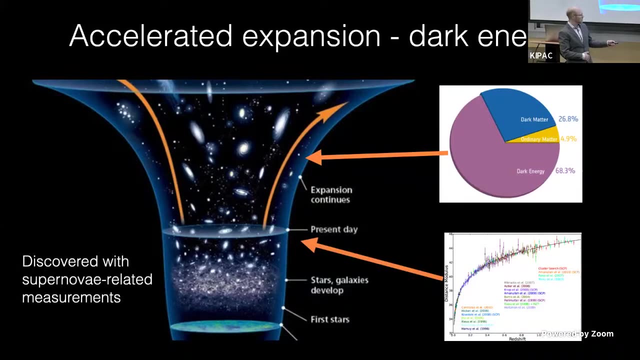 that goes into the details of what may or may not happen at the end of the universe. and again here, when we looked where we got this information about how the universe really expands. we have data, and this is one of these graphs where we looked at supernovae at different distances. 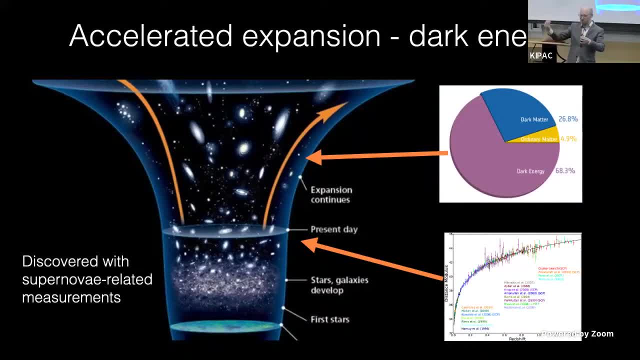 or at different redshifts where we called. and there's also something that ren dr seuss talked in in her lecture: the further away objects are, the universe is expanding and with it the photons when they travel, and so something that's further away has, when it's being emitted, has traveled through. 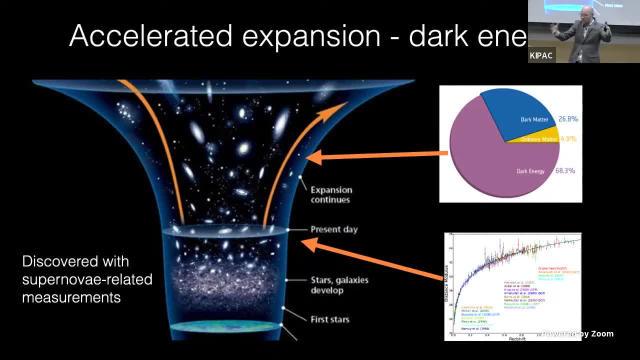 the universe and the photons have expanded, and the photons have expanded and the photons have expanded with it, and so we see it red shifted, and what this curve, briefly, is a diagram of how bright these star explosions are at different, uh, redshifts, of how the universe has spread and this has led. 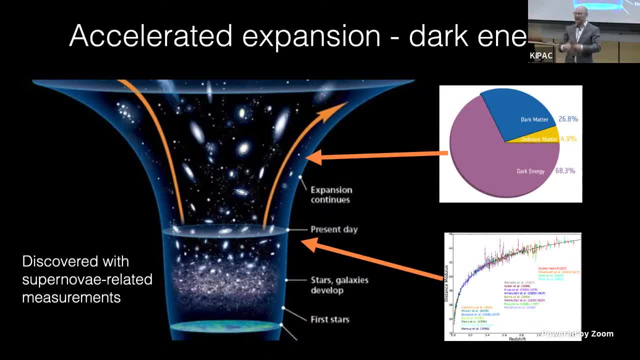 to the conclusion that the universe needs to be accelerated to explain this data, and even more and more accelerated as time comes closer to the present day, and then we can project it even more. and this was in the late 90s, so very recently. so, but now the question: okay, we have established. 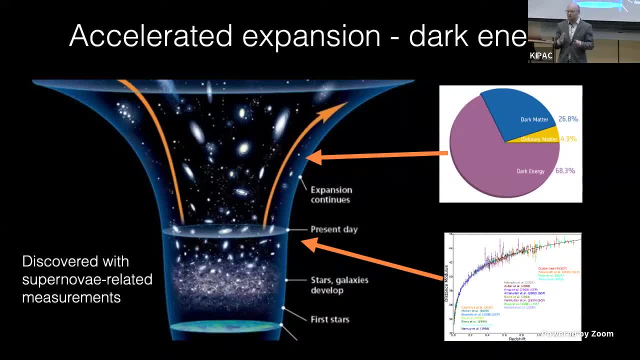 it accelerates. we don't really know why, um, but the question is how much it really accelerates, and that's a harder question than we may think. it's easier to say that something accelerates. it's easier something- the dynamic part- than actually saying how much is the current. 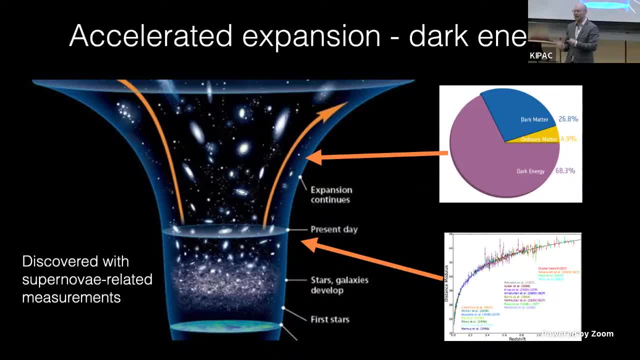 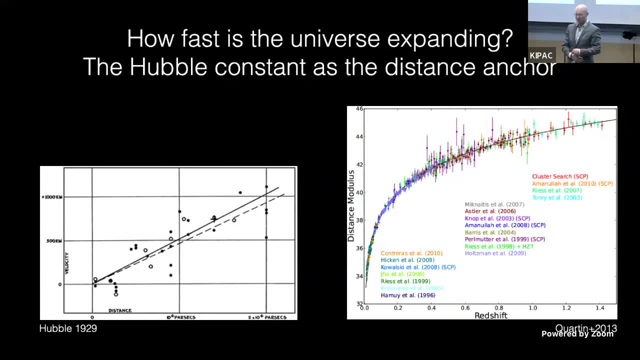 acceleration rate of the universe. very simple question, a very hard answer answer, And so one of the first studies that went into that to look for how fast is the universe actually expanding today is Edwin Hubble, among others. So he got a bit too much credit for that work, I would say. 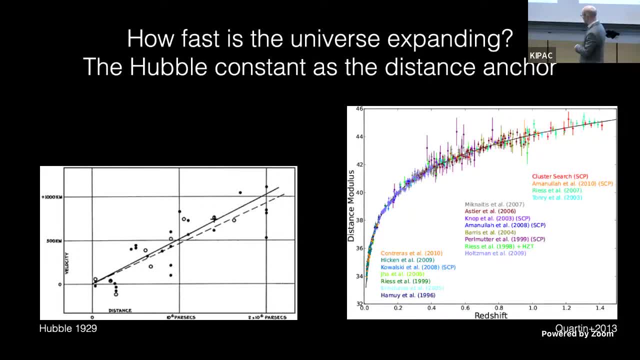 But here his diagram from 1929, where he puts here on the x-axis, distances in these units of parsecs doesn't really matter what, it is just further away and we are here And here velocity. so how much recess velocity these objects go away from us. 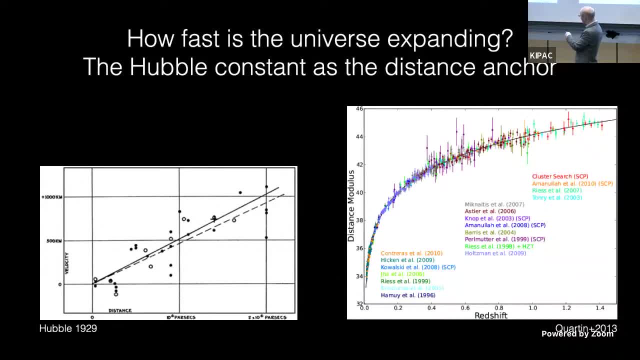 And you can put these different galaxies. these are data points or galaxies. you can put them on the plot and what you can do is put a line through it and say: the steepness of this line is this Hubble constant. That's basically it. 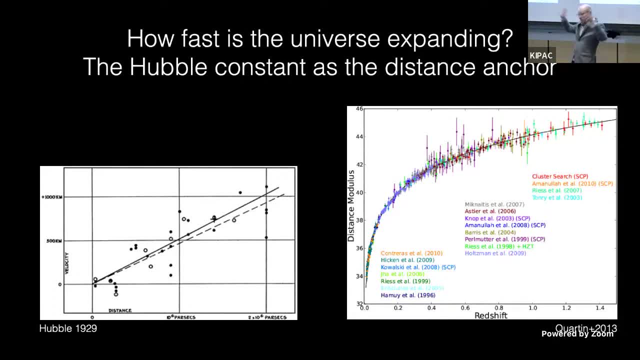 So if something is further away, it's recessing, going faster away from us, And the question is how fast? And for the very trained eye view the units are even wrong On this graph And the number here is like: okay, in one parsec it goes about 500 kilometers per second. 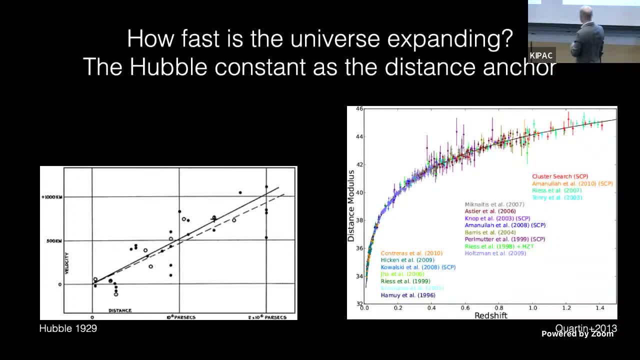 away. This was then Almost 100 years later. these diagrams are now being made with supernovae, And these are quite modest. They don't write distances here. They write this thing called distance modulus, modulo, something that we don't know, or we. 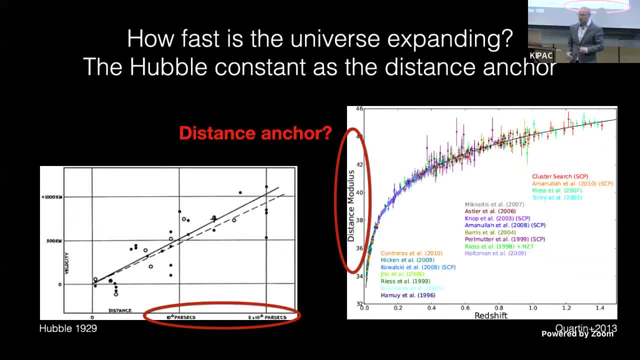 don't have calibrated, And so the question here is really the distance anchor, where to come, the absolute distance, How far is Andromeda galaxy away? How far is the Large Magellanic Cloud away? How far is the next star? And these are not trivial, actually very hard questions. 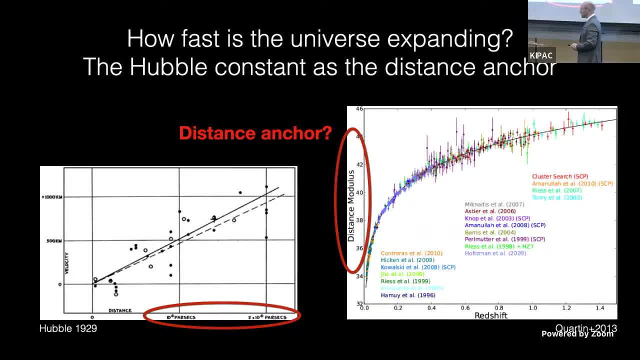 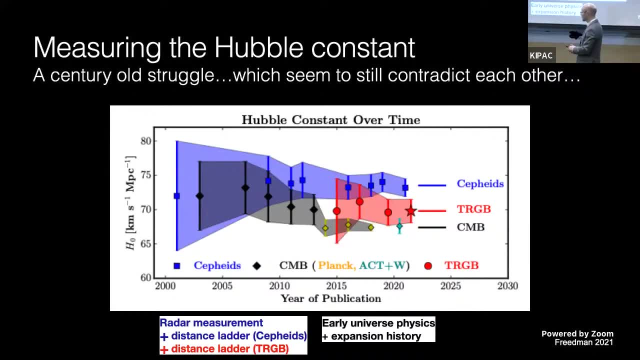 And we're still fighting with it. And if we go through the history of recent measurements of this Hubble constant of the current expansion rate of the universe, Here It dates back to about the year 2000.. This graph could have made back to 1929.. 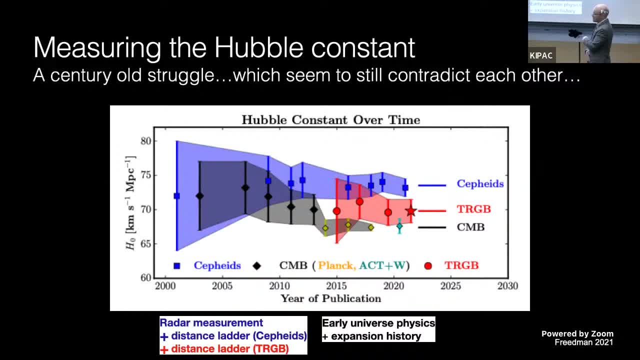 And just the numbers here. they're around 70. And on Hubble's diagram was a number around 500.. So through the roof somewhere, And you just see how things are being still struggled. And, interestingly, over the last about 20 years these measurements got ever more precise. 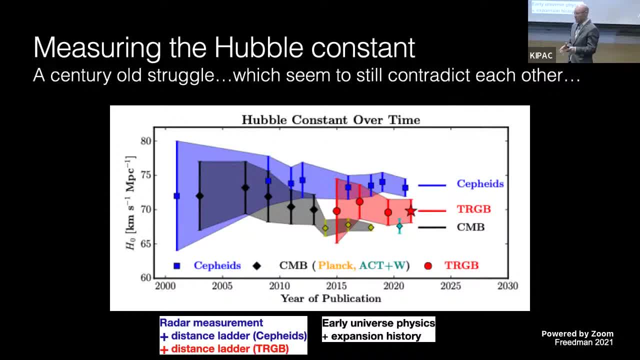 with different techniques And some of them tend to more and more Or not agree with each other, And that leads to a mystery. So an example here is what is here under CMB, the cosmic microwave background, When we assume how the universe has evolved in the very early dense plasma, how plasma 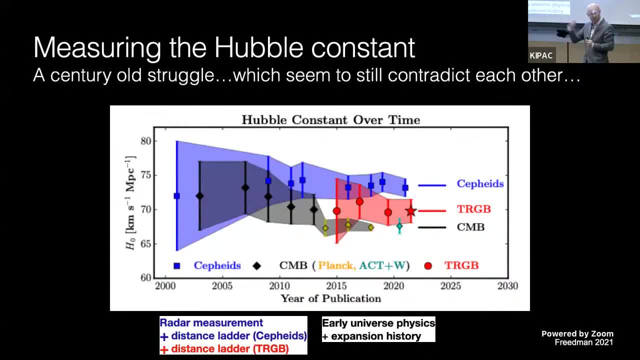 waves evolve. This is a relatively simple physics. If we put it into, we get an inferred answer that is around 67 right now- Really small error bars, Yeah. And then we have other measurements, which we call the local measurements, And I'll come to that how they're being done here, with C-feed, variable stars or what is. 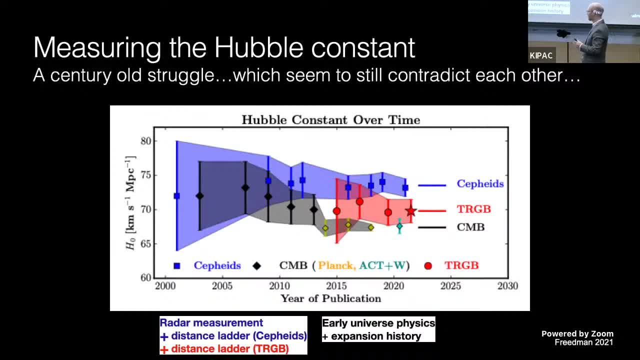 known here as TRGB, tip of the red giant branch hold for two minutes. They tend to be higher And this may or may not indicate that what I told you in the very first slide, that I'm very confident to describe the universe. 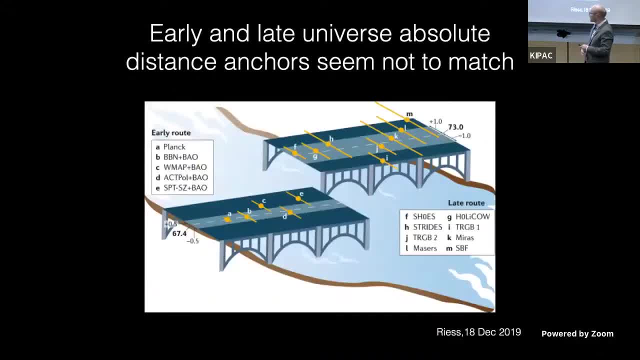 I may be not so confident to describe the universe, Because there's some indication that something does not really match. And if this is true, that this doesn't really match, it also would imply that the story that I told you- that these black lines fit through everything- doesn't work that way. 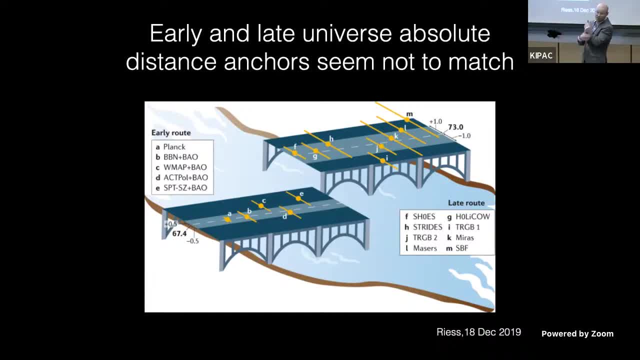 And so that we need at least a different component or throw everything away and rebuild it from scratch in different ways. And so, from an experimental physicist, this is exciting to probe and test ever more precise, to see where do our current understanding break, and that helps us guide of where we. 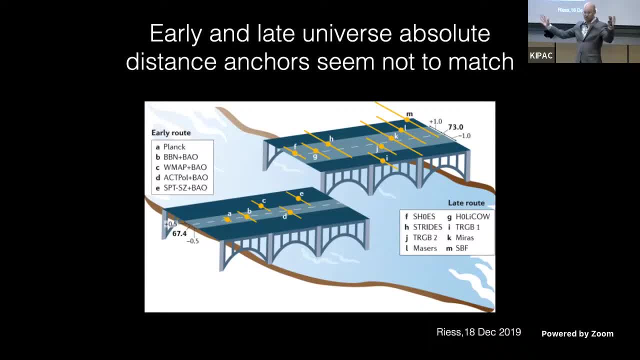 can put our faults In if we are too divergent between experiments and theoretician. But hold a second. So it could be new physics. But it could also be that some of the measurements are not as precise as we think they are, And this is a term we colloquially use, a systematics, which is basically mean we are overconfident. 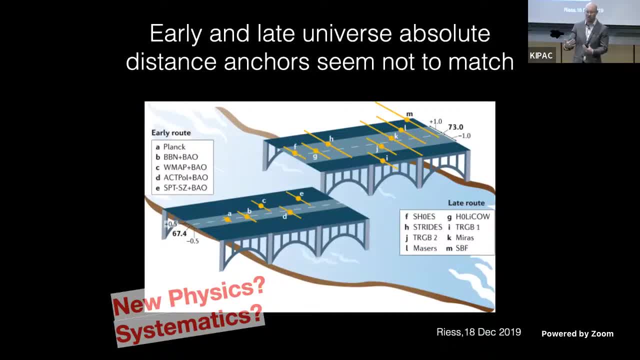 in our statement we have forgotten to include certain or we have not ignored that we actually making some assumptions that may not be. They may be good, but not good enough for the specific statement that we're making, And so we're always at the edge of finding new things, learning about the universe. that 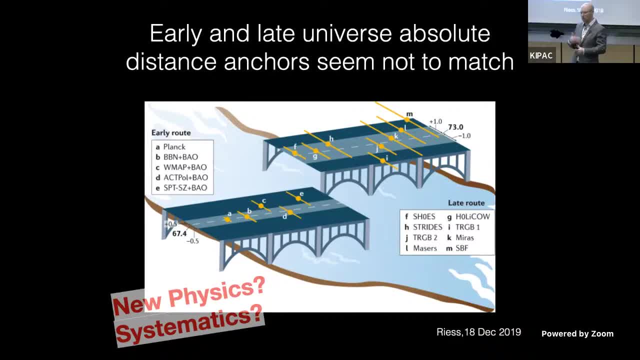 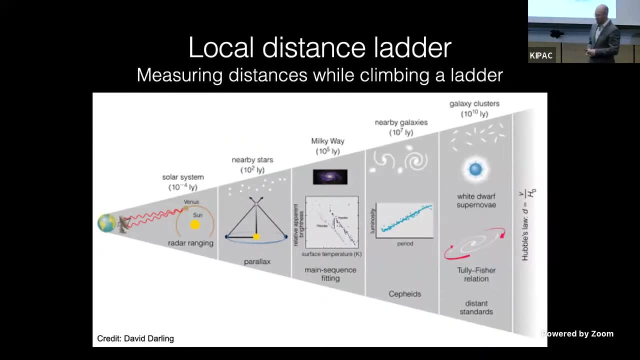 sometimes we're going maybe a bit over it And so going. this is tedious work to go into. are the stated uncertainties as good as they should be? So the distance ladder I. So what are these measurements made of? and that leads them to the 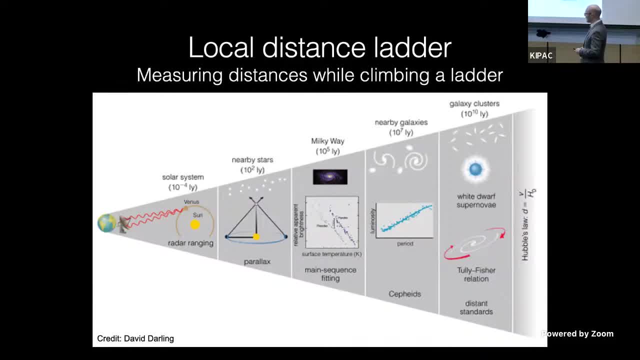 To the James Webb Space Telescope again. So when we measure distances, one what we can do. we can very well measure time. clocks are extremely precise. that's the thing, the state of the art, What we can also do. we can send radar signal from our earth, bounce it on Venus, for example. 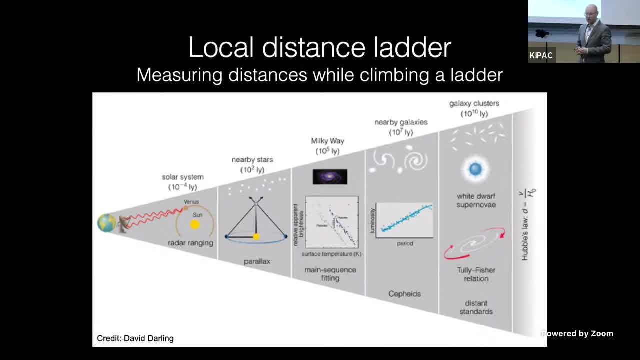 and it comes back to our dish, for example the Stanford dish here, and we can click the time, how long it takes, and we measure this distance remarkably precise, to something like a few centimeters. We can measure the distances in the solar system with such a radar observation. 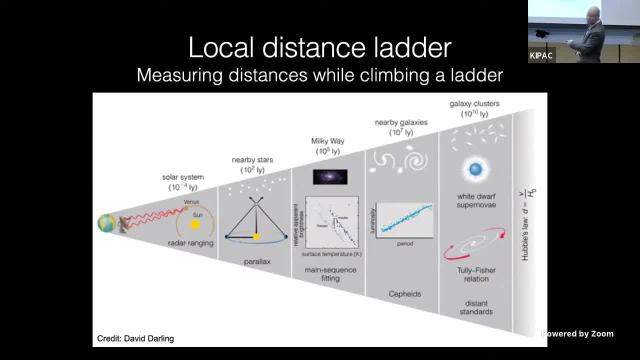 What we can't do is send this radar signal to stars away or even galaxies that we wish that's not coming back in the lifetime and will not measure into signal that's too weak. I wish it would be that way, And so what we need to, as inter mediatory, call liberator of how we do it. 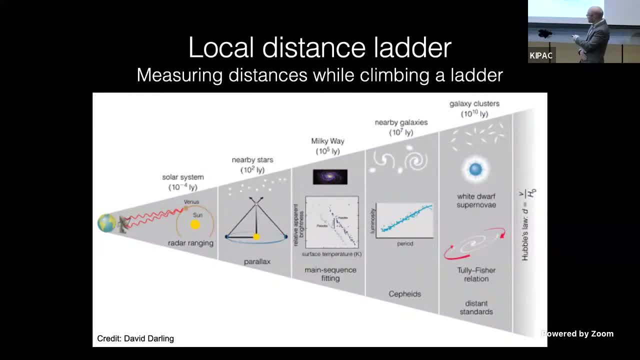 And one way to do is is what's called the parallax method. We can use the fact that The earth And everything else in our solar system is actually rotating around the sun, and if something is above us and we're moving on the left and on the right, it changes the angle on the sky. 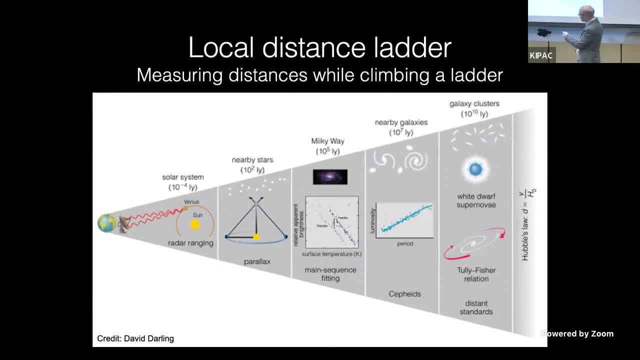 and this is the parallax method, and so when we know this distance, we can get geometry to the stars, and amazing progress have been made, for example, by the Gaia satellite and a lot of very precise techniques that measure these angles very, very precisely. So that's the next step. 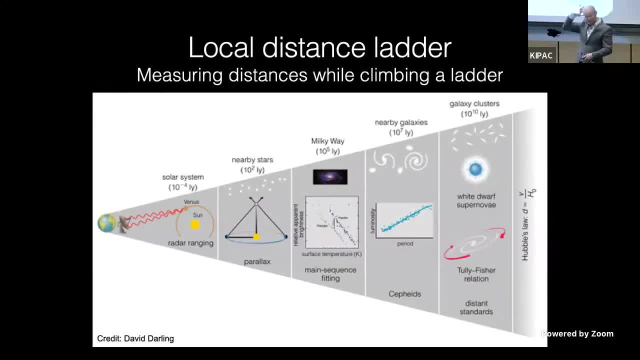 But it's still not the next galaxy, It's not the galaxy on the other side of the universe that we barely can see far away. So we need other, more luminous sources intermediary, And so we can use different techniques, such as, for example, see feed variable stars that. 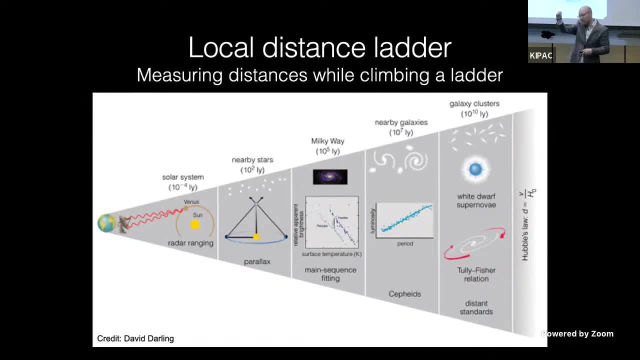 we can measure some of them with parallax, See how bright they are, and if they're like four times dimmer further away, we know it's like twice as far away. So and then go step by step out, And if we want to go very far out, we need to have something very bright and something. 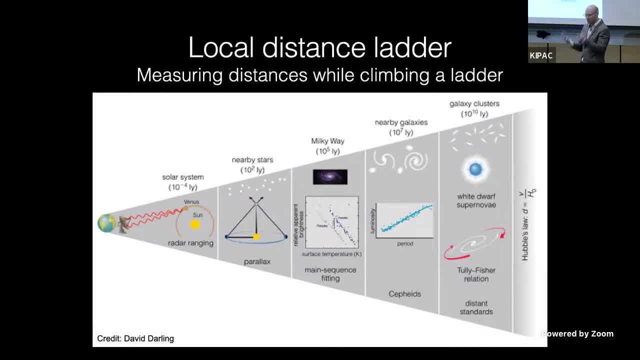 very bright is something that explodes, for example, like a star supernovae, And so we can use then the more localish supernova where we can still see sea feeds in there, to calibrate how bright a certain intrinsic luminosity is of that supernova and then learn. 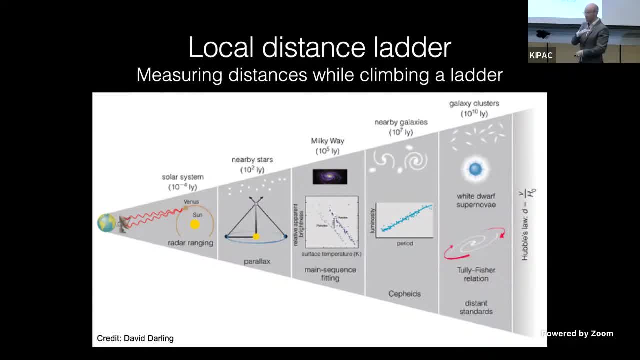 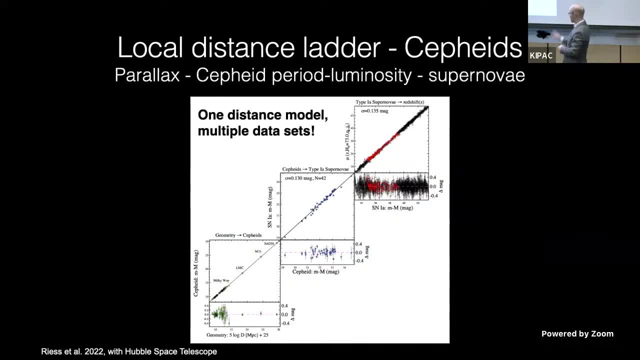 about- and you see already like this is a long story and I abbreviate it like a lot- and so recent measurements and here come through some data point that there was the one of the lines that gives a very precise measurement of the Hubble constant. This is a study with the Hubble Space Telescope went through such a thing and this line here. 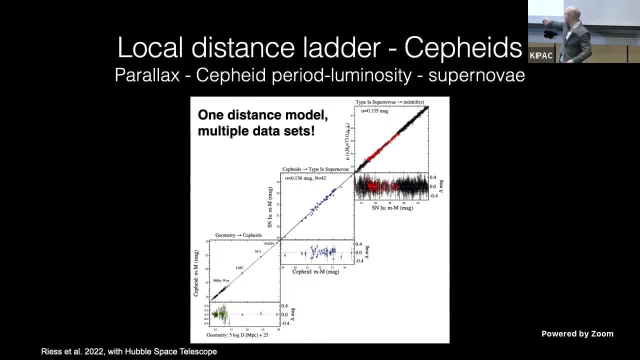 is a joint fit of distances throughout, you know, a very large part of the, or the local universe, where we, with different techniques, aligned with each other, and so this involves parallax. I mentioned that, so this is the first rung, so to speak, in this ladder. so when, when we 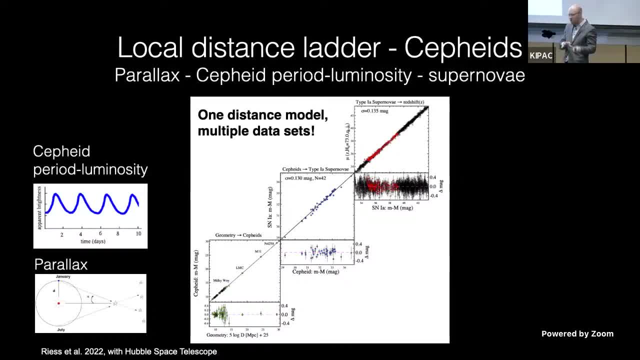 walk up. the next step is the sea feed periodic period, luminosity. so it's a star that kind of like has a frequency at how bright it is and what period it has. and you, if you say they're self-similar everywhere, you can calibrate and say like, okay, this was so bright, so this. 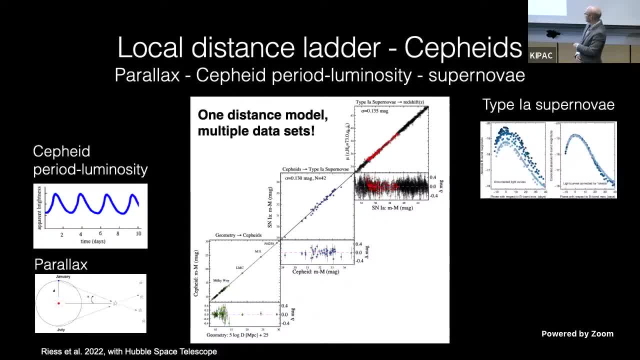 has to be further away. these are the sea feed and then the last rung is the type 1a supernova. as you may Or may not see here on this plot, they're not all the same but they have some similar relation that you can put them on the same plots and stretch them and squeeze them and 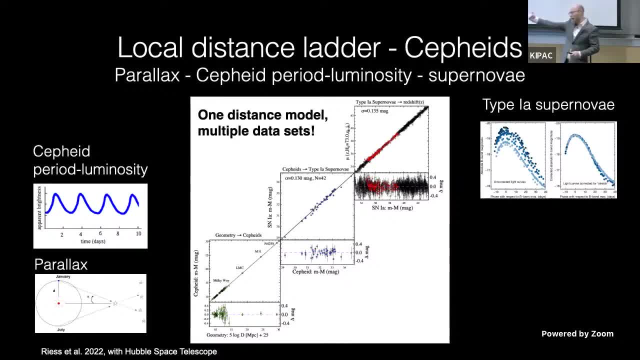 then you can use them as calibrators. so this is a way to go out to the universe where we can really measure the expansion rate very accurately. so here again, new physics or systematics when we go through this. this is a very precise measurement. a lot went in there, but there. 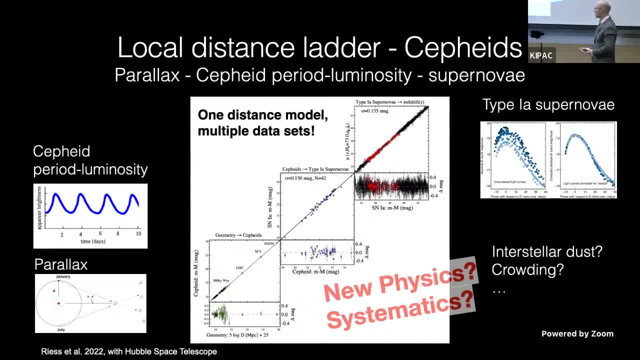 may also be some uncertainty. Is there some dust in there that we haven't accounted for? is there some crowding effects? do we really measure the same thing that we want? are we slightly offset in between? do and we understand what the sea feeds are? questions over questions that hundreds of people spend. 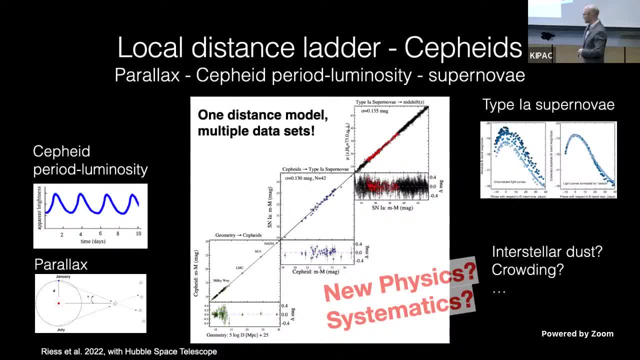 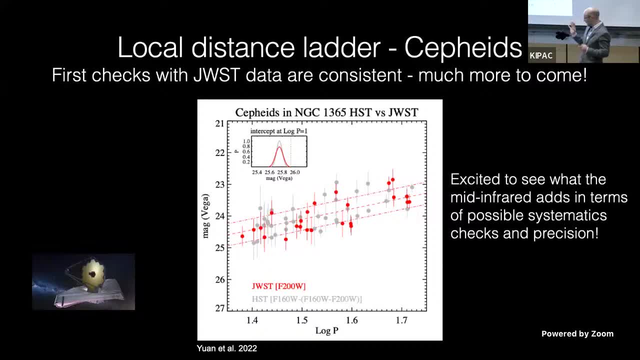 their daily life, sometimes nightly life, on to make sure that this is accurate- and this is the first publication that came out that I saw from JWST about that matter. and here it's not about all a new measurement more precise, or disagreement, No, this is just to show that in the safe wavelength- wavelength with a different telescope- we 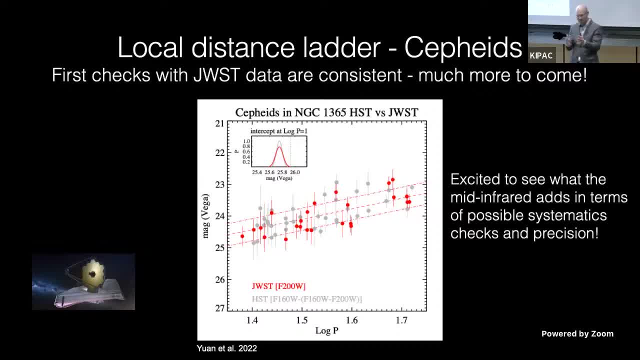 get the same answer. And this is just the first step. when you then go forward and say, like we now use the new techniques, the new capabilities, that to make sure that, under the same capabilities as before, we get the same answer, And that's just showcase that's current state. 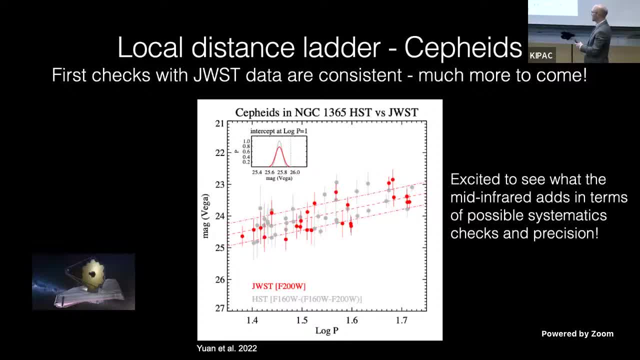 Just right now, Right now of what the James Webb Space Telescope is doing with the seafood science- and a lot is in progress here- And I'm excited to see when we push to the far infrared and whether we see either some differences in this analysis or whether it actually makes it more robust and gives another. 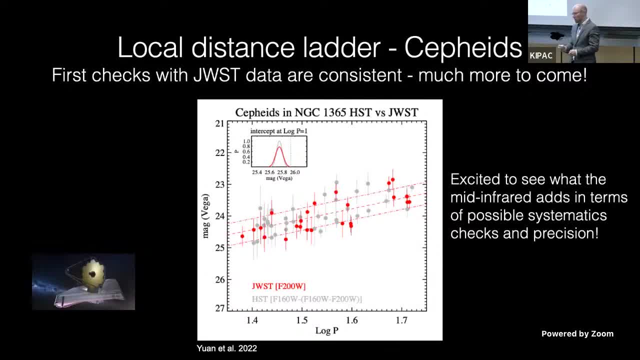 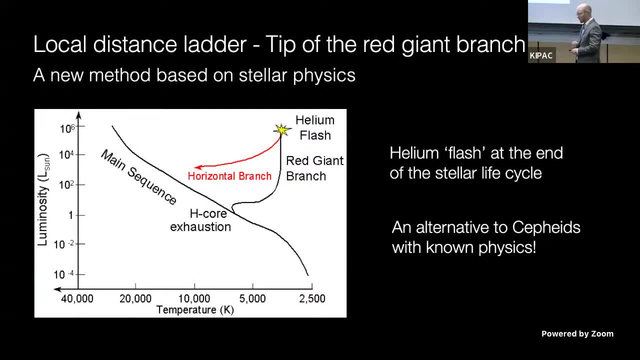 pillars like: yes, it's true. What I'm more excited about personally is a different technique, using stellar physics to measure cosmology, And here we talking about the tip of the red giant branch. In very short, a star is somewhere on the main sequence that is defined by its its 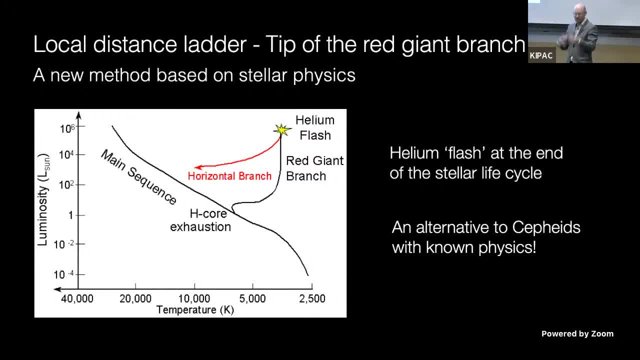 mass and its temperature. it burns hydrogen mostly, as our son does, And when the hydrogen fuel is used up, it construct until it starts the helium burning And at one point it creates this helium flash. And this is a specific moment Where we understand physically what's going on. 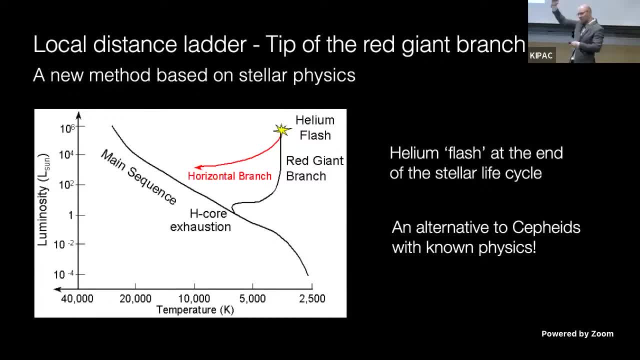 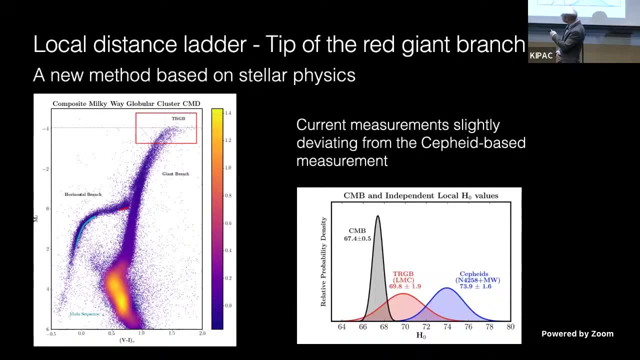 And that leads to a certain calibrate there, if you see stars right at the tip And we can know the difference in distance, for example, in how bright they are, And so- and this is an alternative method, And here's an example, some measurements of brightness of stars where you can basically 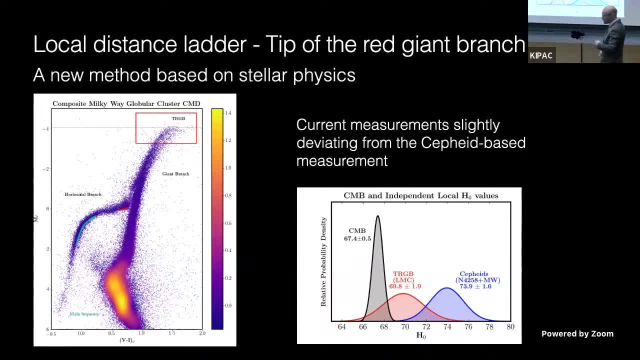 see where this tip is And this method currently used with the Hubble Space Telescope. If there's some measurement in between, it could be high and discrepant. It could be in agreement with the what we call the late, the early universe physics. 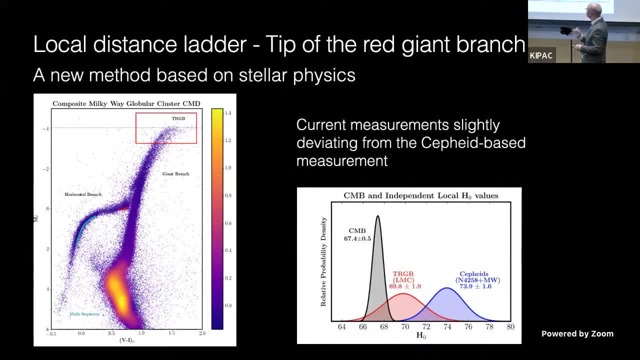 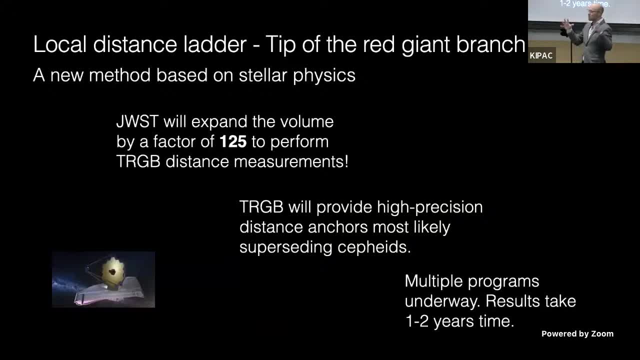 We don't really know. But what JWST is doing is it collects about 125 times more volume where we can do this measurement And if we have done all the programs, this is really the ability to settle the debate, Settling meaning either one or the other way. 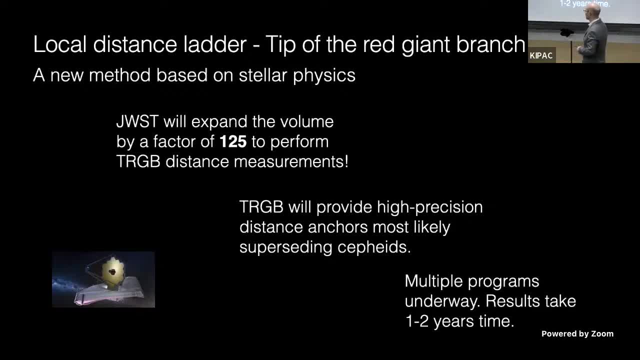 And if we have done all the programs, this is really the ability to settle the debate, And if we have done all the programs, this is really the ability to settle the debate. Do we need new physics, or is it systematically driven? And so that's very exciting for me and many others. 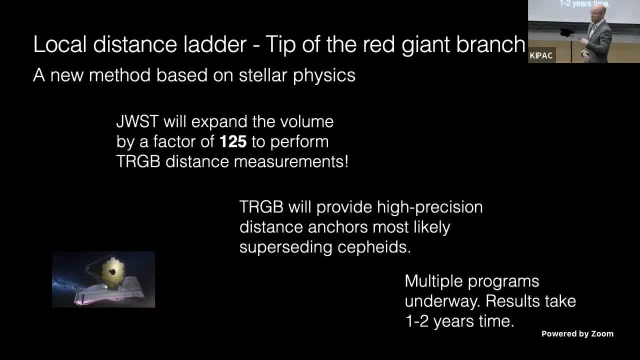 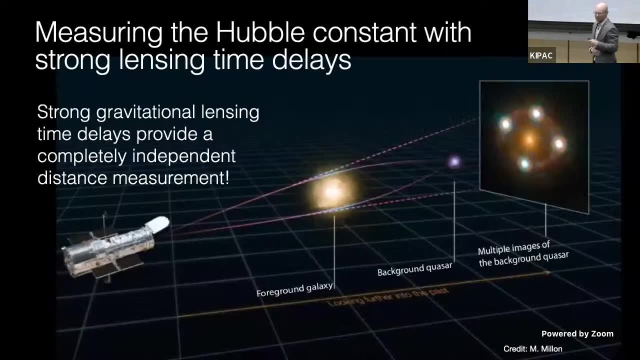 And again it takes time. Multiple projects are on their way, but it was just in the beginning, learning the experiment and going step by step towards it. So, and in the last few minutes, it is another measurement that I'm very excited about with. 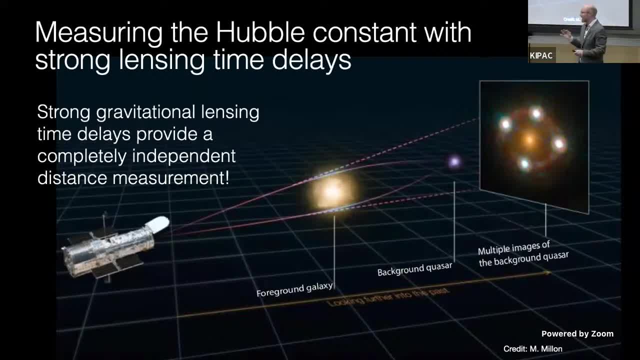 again strong gravitational lensing, measuring the Hubble constant, And be using the technique called time delay cosmography. So what we measure here with quadrupole lens, quasar, these images, it's the same source in the background. We're not just 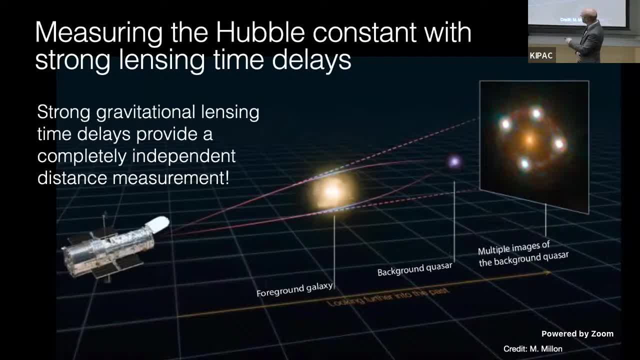 seeing them multiple times. but the light path, the light travel time is different between the different images, And so if we can measure that relative light travel time between that image and that image, we can get a depth information of how far away these objects are If they're closer to. 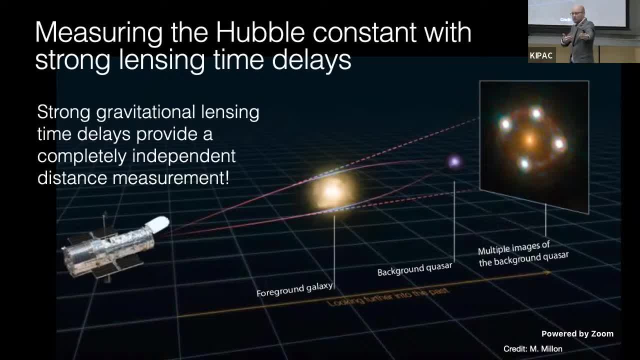 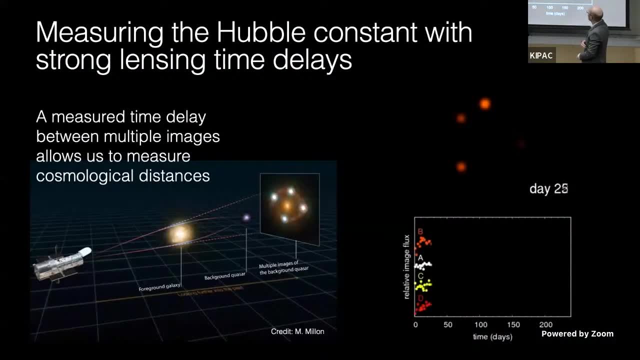 us the light travel time is shorter, The further away of us they're longer. So we get a one-step measurement of distances right away, And this is exciting. And so here, for example, these quasars flicker, And so we can adjust the flickering to each other, And we have also experts here in the 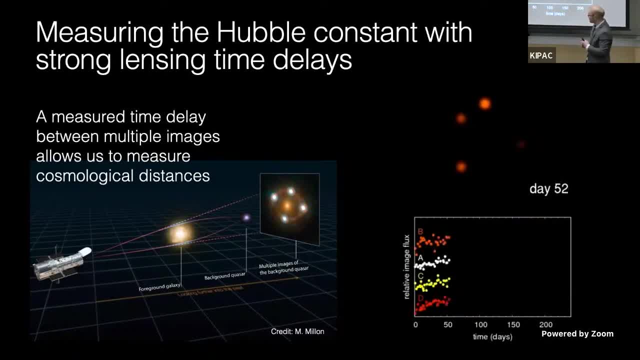 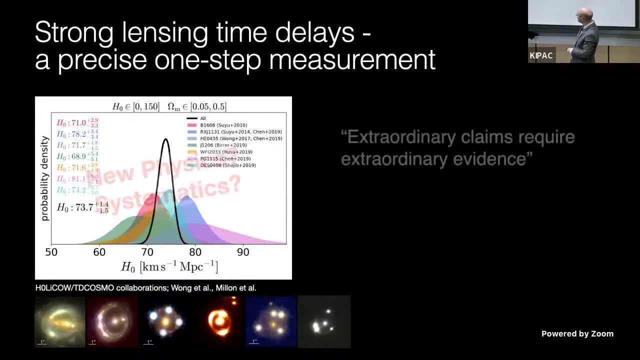 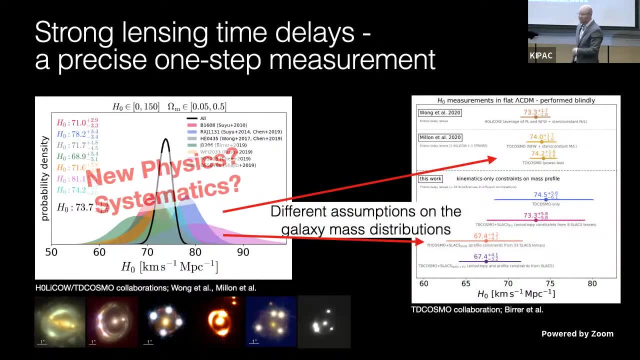 audience that do that very well and very precise. And here again we have a precise measurement. It seems to be high, But again, extraordinary claims require extraordinary evidence And depends on how you do. it depends on how you run the assumptions. you may or may not find the same answer. So we're really opening the box again. 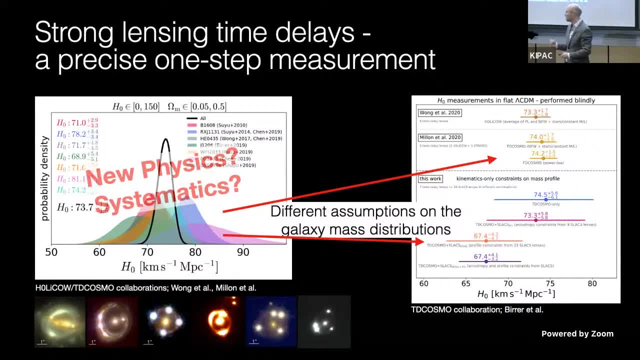 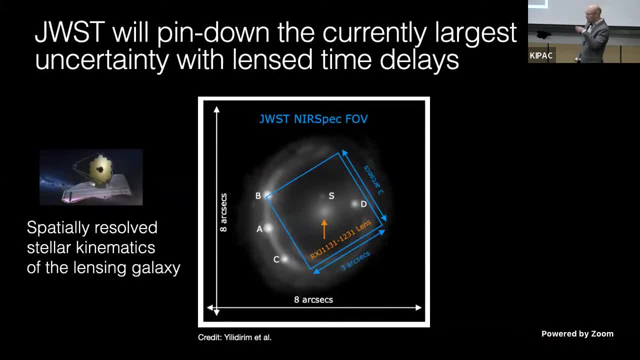 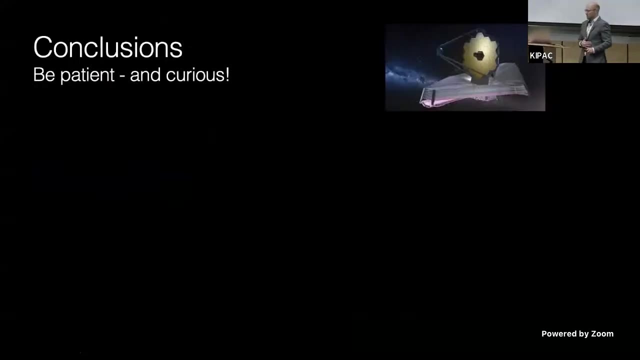 and again and again. And there JWST is very impressive, where we can do spatially resolved studies of such deflector galaxies But where we currently have not so much knowledge about that to really anchor down and show are our methods robust enough. And this is just the beginning of the studies. And with that I want 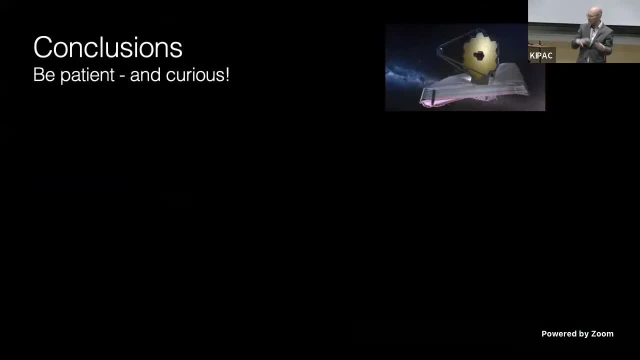 to conclude, I showed you a bit about dark matter, dark energy, where we are right now, the open questions. I showcased you just a few examples of what's going on right now. And conclusion here: be patient and curious. JLT is the most complex instrument that's been flown to space, which required us a lot to learn about that instrument. 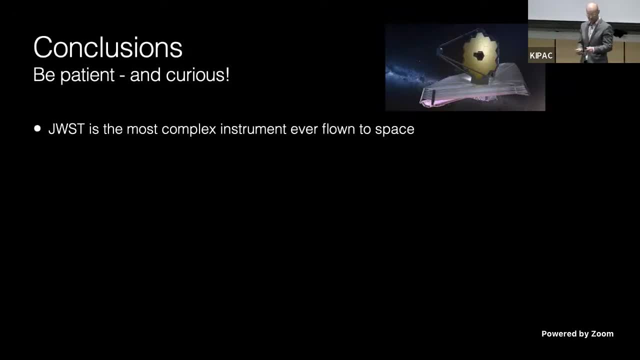 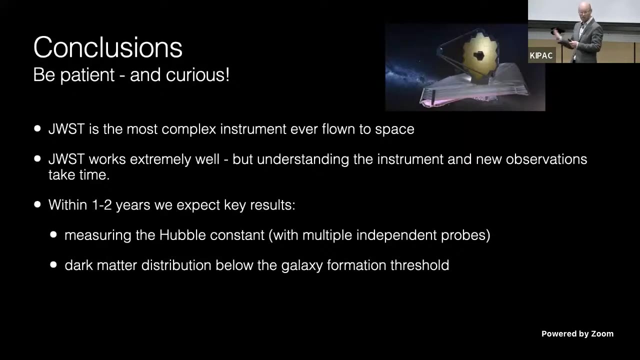 before we can really trust what's going on, And that's just takes time And it works extremely well, But understanding the instrument takes just time. I I'm within the one or two years. I highlighted a few studies of dark matter and dark energy that hopefully change a bit our view on this. 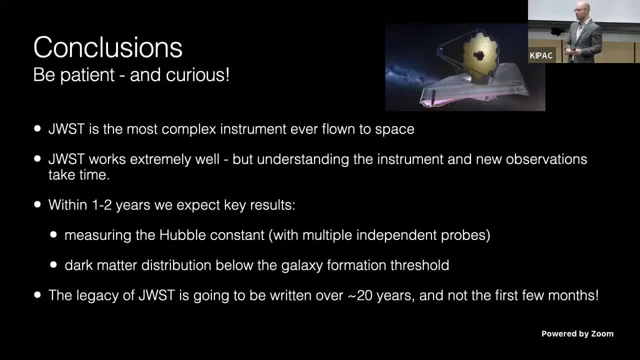 and the legacy of JWT will be decided not in this next few months. it's an instrument, it's out there for 20 years and it's our imagination how we use it to change our perception or a view of the universe. and with that i say thank you very much for your attention. i'm looking forward for your questions. 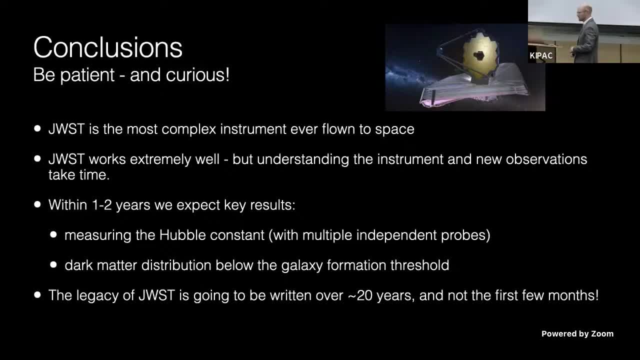 wow, that was a very amazing talk. thank you, simon. it feels one of those talks where you've learned so much, yet there's, uh, even more questions coming up. so i'm sure there are a lot of questions from the audience, but we can start to take in-person questions, so feel free to. 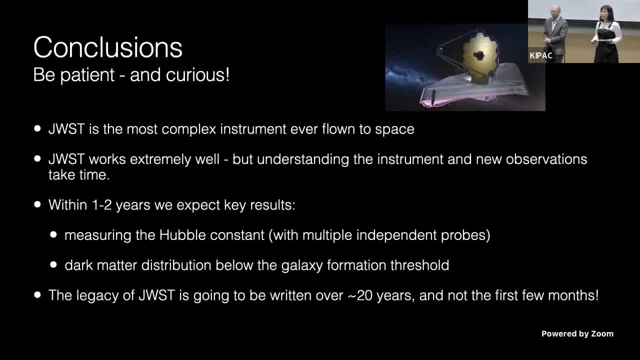 you? yes, great, thank you. um, i'm gonna just quickly repeat it for our zoom audience. um, so the question was: uh, do you think the universe is finite or infinite? and how does it tie to the entire paradigm that you were just talking about? um, yes, so the pernicus principle states that there's 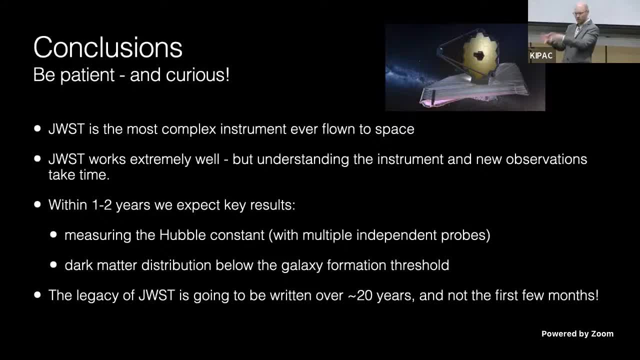 no place in the universe that is more preferred than other, and if you take that to the extreme, as soon as you have finite, you need somewhere- boundaries, and as soon you have a boundaries, you're somewhere in the middle of it, and so the principle that there's no special place requires you directly. 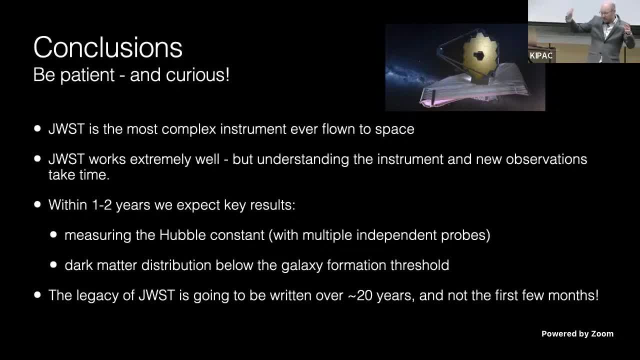 to not have boundaries. we don't see everywhere, so we only get light, information that travels to us, and so our accessible universe is finite of what influences us here. the story that we were written, the history of the earth, of our solar system, is finite of what it could interact with. but there's no border, and there's so in that sense. 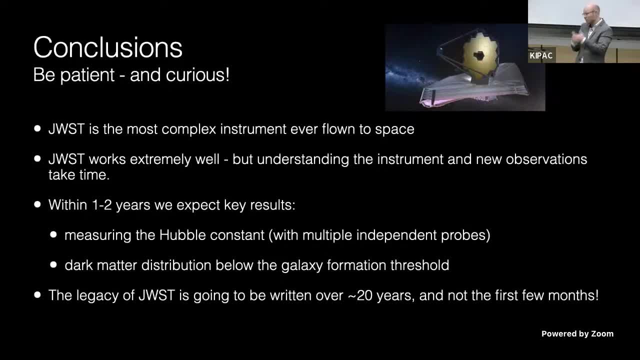 it's infinite. um, yeah, and that is part of the cosmological picture that is over and over, uh, confirmed by data. regardless of where we look, we see the same thing and no boundaries. great, there is actually an online question from tyler also asking about, uh, you know, space, uh and uh, the universe, of course. so are things really moving? 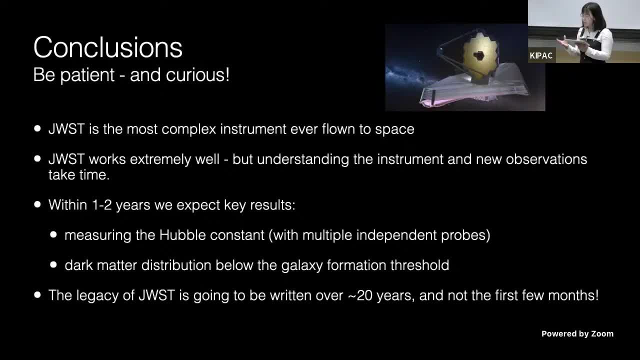 through space or are they just appearing to be moving just because the space itself is expending? and if the space is expending itself, what is it expending into? yeah, i must say i'm always struggling with it the way i imagine. i'm always struggling with it the way i imagine. i'm always struggling with it the way i. 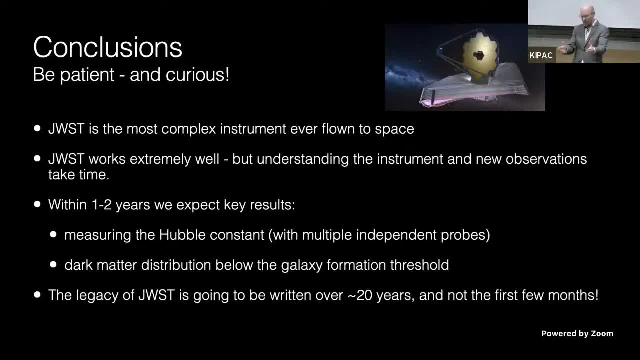 imagine it for me is: if you think of a grid that you lay out that never ends, you always can put in another line in your grid again, comes back to there's no center of that grid and now you can say, like you squeeze all the grid points slightly more away from each other. this means if you go, 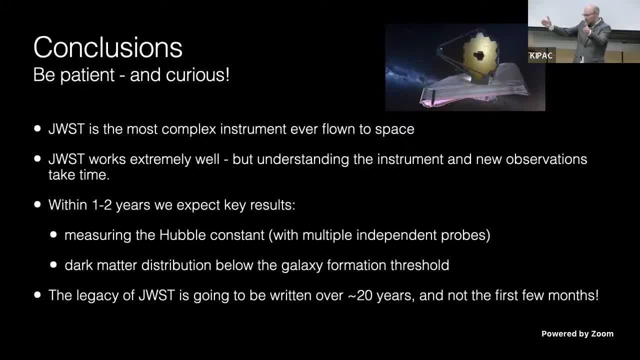 the first grid point one step away, the second one needs to go two steps away, such that the second and the third one is also going apart from each other and in that sense it doesn't expand somewhere else. it's an infinite grid that just expands itself and constructs, so it's in itself that it expands. 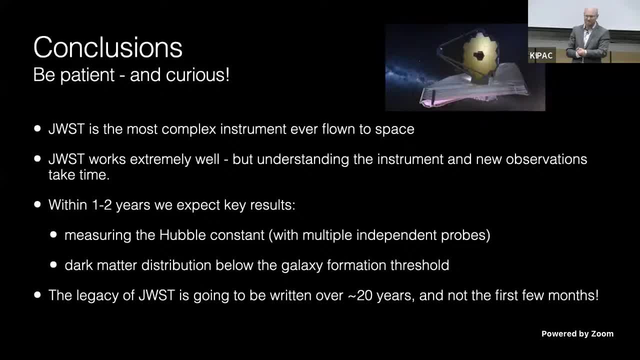 thank you over there. well, the honest answer is: we don't know. the best answer it can give is: it most likely does as well, well as everywhere else. it's a great. a lot of people do that, in fact, and the problem is they haven't found anything. they've built better and better detectors, and they're well designed. they. 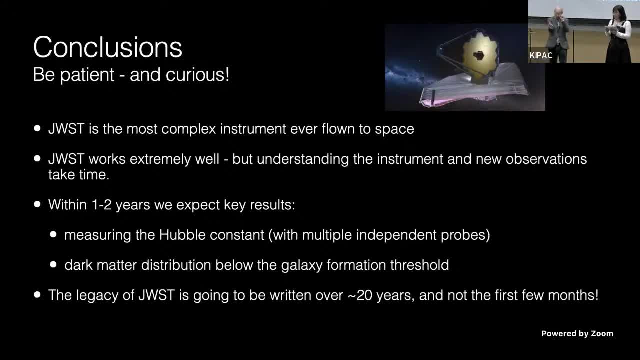 measure incredibly well anything that may come and give a bit of recoil to, to atoms, but if it's not interacting with the thing that we can control and measure out of devices, then we don't see it, and so in that sense it's a multi-pronged problem or a multidisciplinary problem. dark matter. 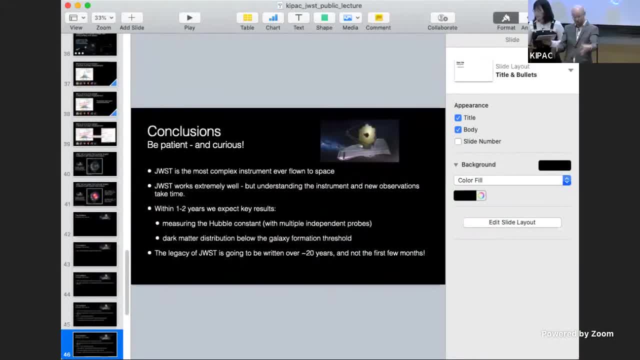 there are particle physics, that physicists that work on the ground- here there's a lot of people actually are kypac- that design these detectors of seeing it and what we are doing here at space. we use space itself as a laboratory to see whether we can learn through the gravitational physics. 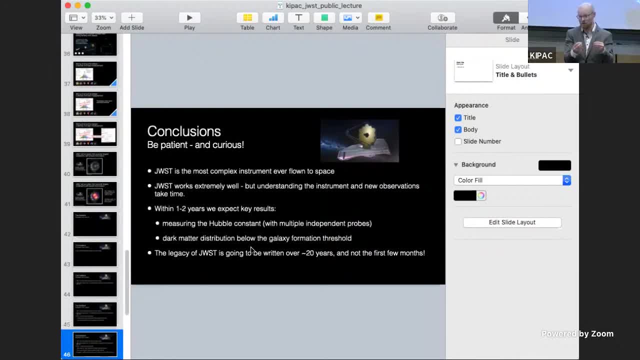 how we can learn through the gravitational physics, how we can learn through the gravitational, how it imprints in our cosmology, of whether we can learn something about the, the microphysics we call the fundamental principle behind it. great um question here. um so if we have dark matter, 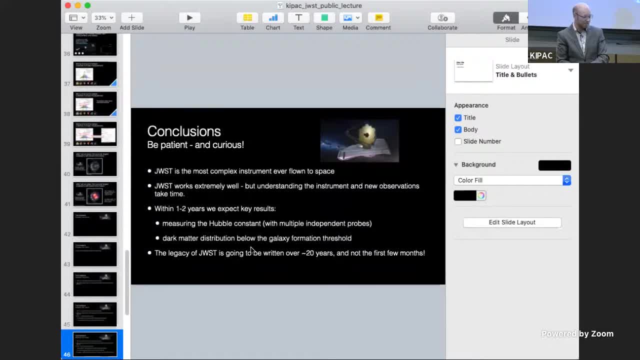 out there but none here, and we have the speed of light. we assume it's constant here. is it safe to assume that the speed of light is constant over there? the data we're getting, assuming the speed of light is constant over there, represents something meaningful. so the speed of light, this is one of them. can you also repeat the question please? 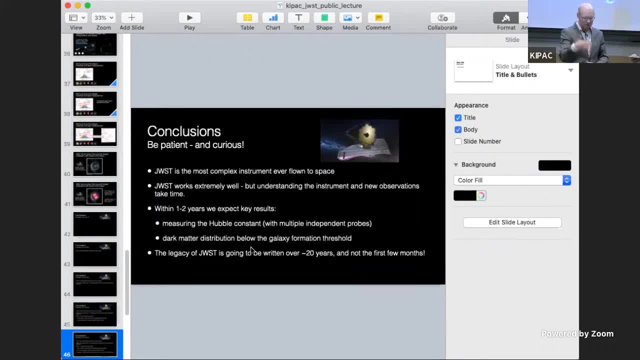 okay, so the the question was, um, whether we can assume that the speed of light is constant everywhere, when sometimes maybe dark matter is some, maybe over there, but not here. um, so, experimentally, the speed of light is so well tested that actually now the definition of what length is. 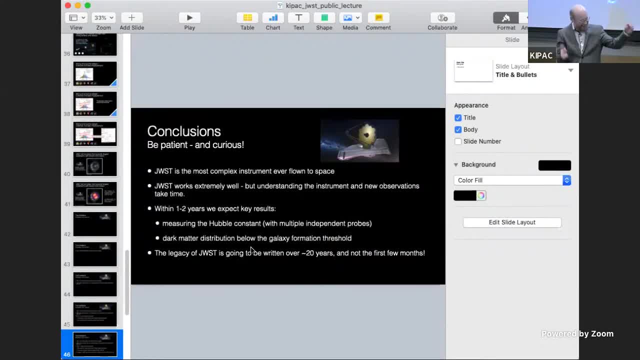 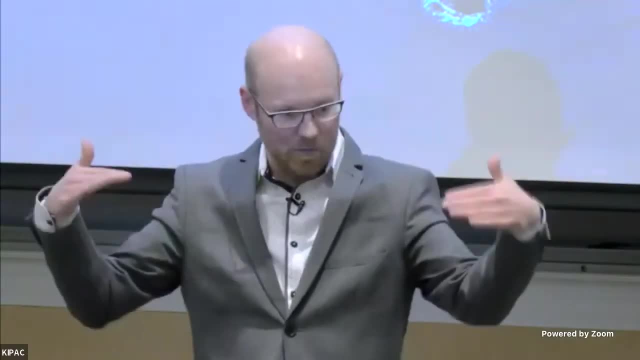 is is tied to it, so we cannot change, uh, the speed of light. by definition it sounds, it's effectively. it just shows that experimentalists can measure time so well and have lasers that reflect or can interferometry. that's basically locally how it's been done. the measure is so precise and it 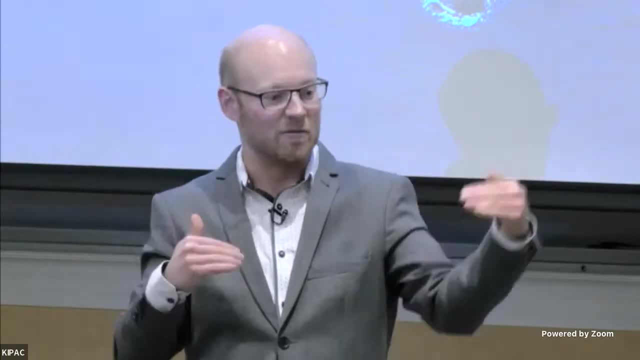 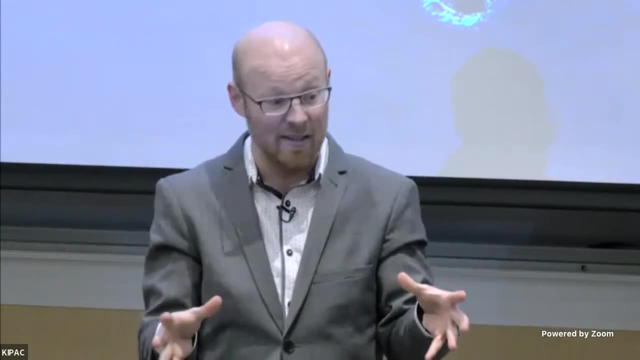 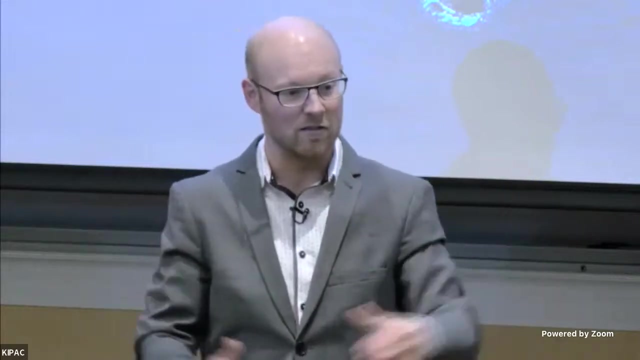 has always been confirmed that they came to the conclusion we're actually fixing length scales to, to the clock. that only works for us, experimentally on Earth or on our solar system. that definition we cannot use on cosmological scales, and so we have to extrapolate and rely on general relativity. 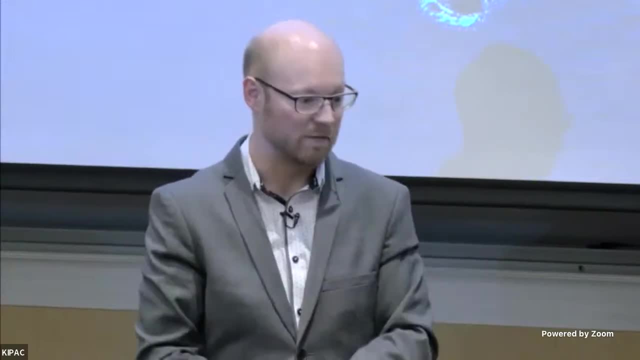 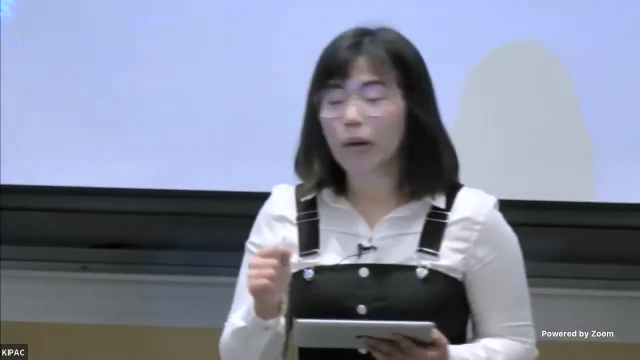 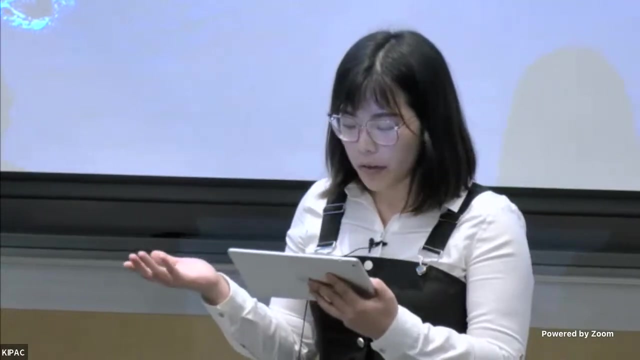 to give us the relationship between matter and length. great, okay, so one. um, we'll take more in person questions, don't worry. um, actually I wanted to switch gear a little bit. um, also, there are questions from online asking, especially especially this one from Phil, asking what, uh, phenomenon or factors that might actually degrade. 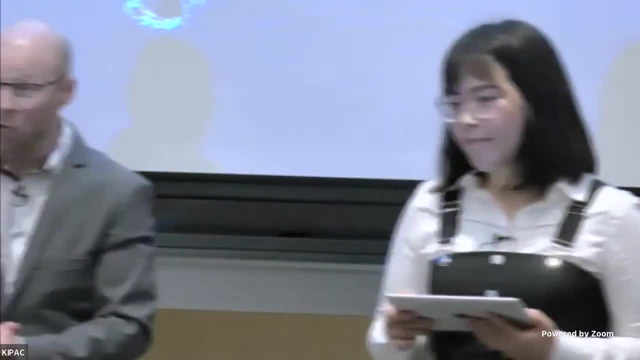 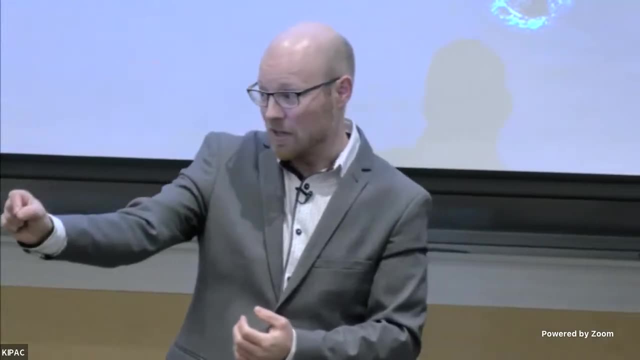 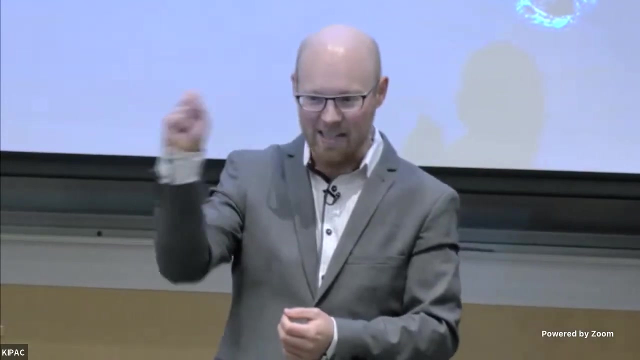 JFC accuracy over time, and one we've already seen: there was a micro meteorite hitting the telescope, one of the mirrors, and this was not expected. well, little objects are in space, that's expected- but how big and energetic it was that actually almost destroyed one mirror segment. and so- and this 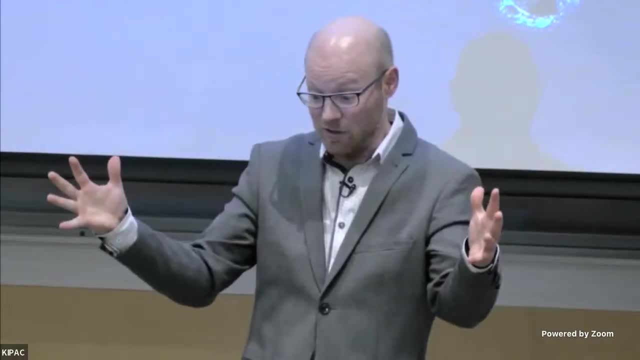 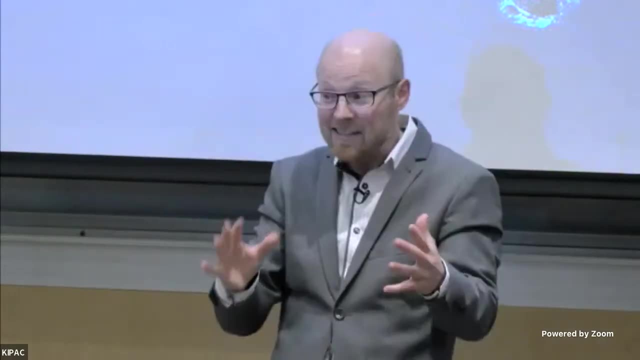 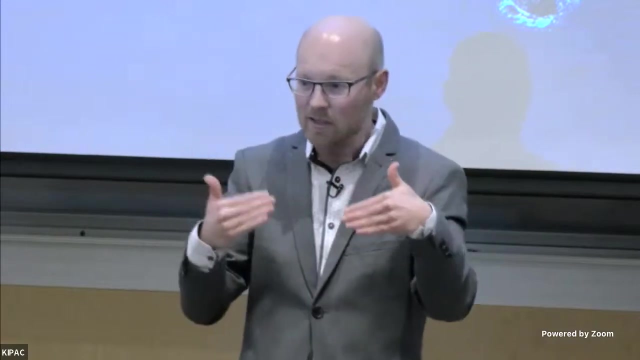 happened very early on, when when they open up the telescope, and so, oh, if this happens every month, we're learning out of mirror time. luckily didn't was a one-time event, fingers crossed- and so this will last. what will be great over time is some like mirror coating here on Earth we can repolish. 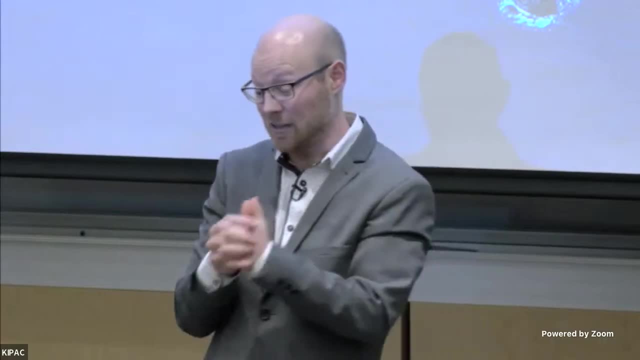 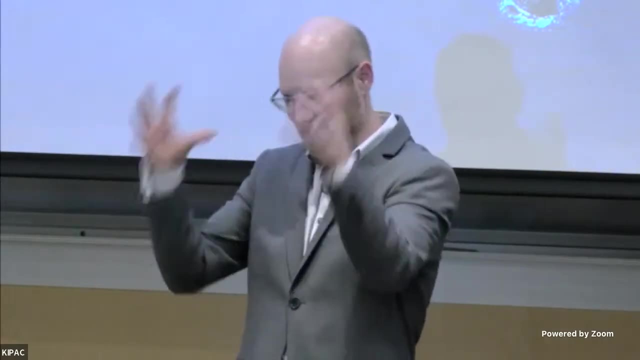 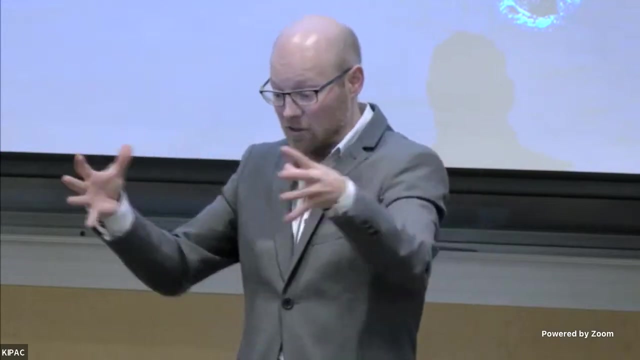 it. that doesn't happen on space, and what eventually dictates the lifetime of the telescope is the fuel. so we need external energy or ex energy that we send with the telescope to actually turn it, twist it and cool it, and once the energy is run off, it cannot stabilize on that orbit where it is and we cannot turn it anymore. and 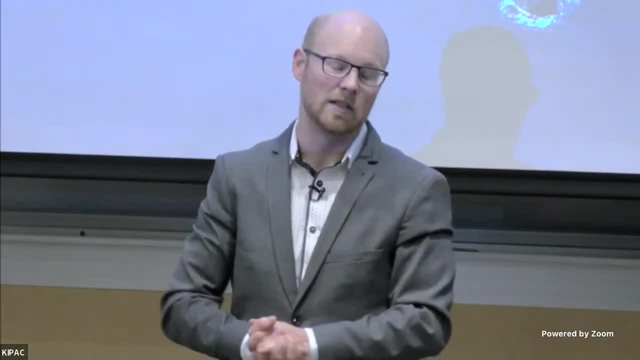 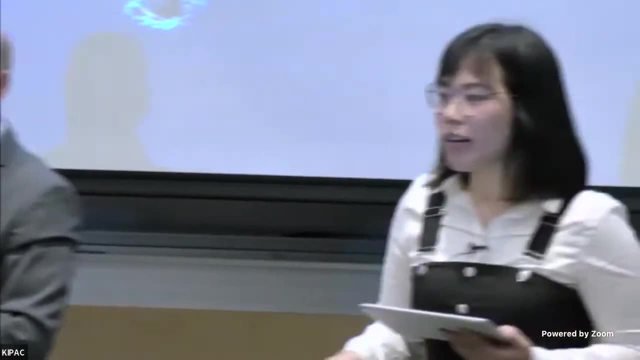 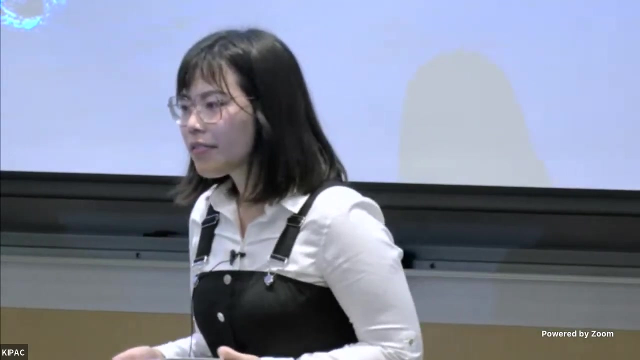 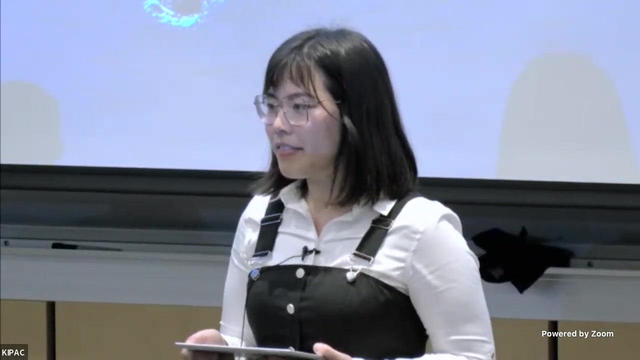 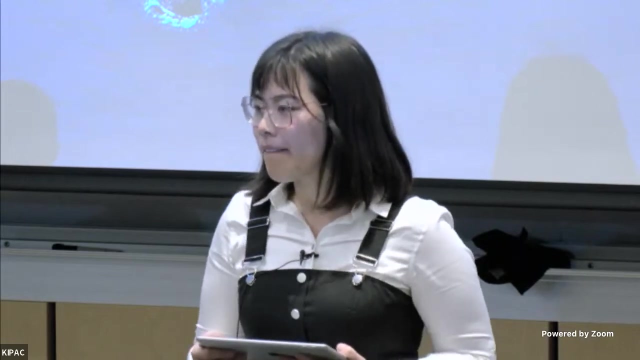 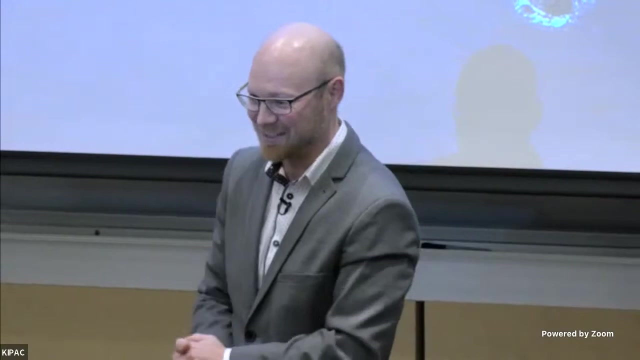 you will just go into outer space, and that's in about 20 years. well, we still got some time. things are not started yet. um, I saw a question over there from our- uh, probably youngest member of the audience. so wonderful question. the question was from one of our, if not the youngest, audience member here in. 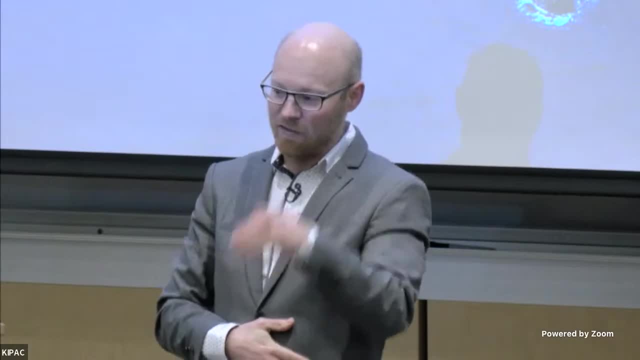 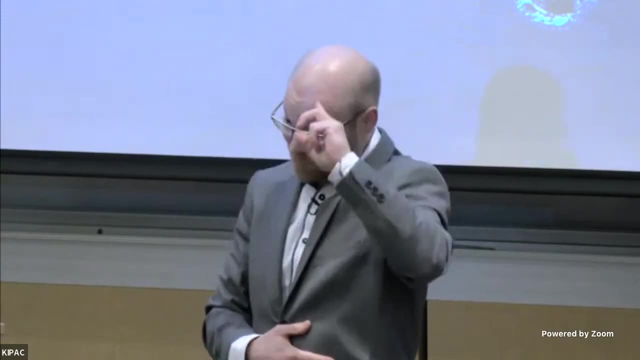 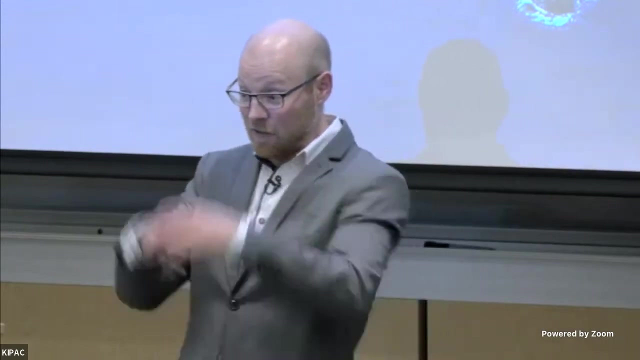 person is: if we look at the star further away, we expect the light of travel to us. so it's older. so and the question: if you, if you go, do it all the way and say like, hey, can we see the Big Bang if we go further and further away, and if the Big Ben itself would have emitted light that travels to? us. we would see it right now at and very close to the Big Bang. the universe was so dense that light could not escape. it just bounced back and bounced back. but then at one point universe became less dense, expanded, and at one point is these, photons did not bounce back anymore and start traveling freely. and that moment. 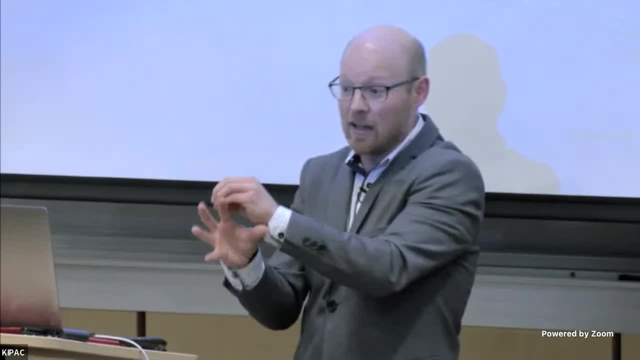 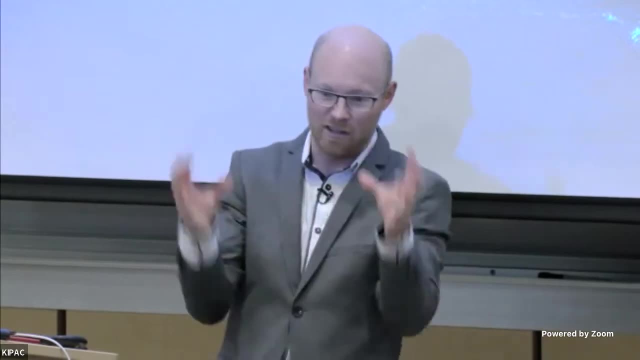 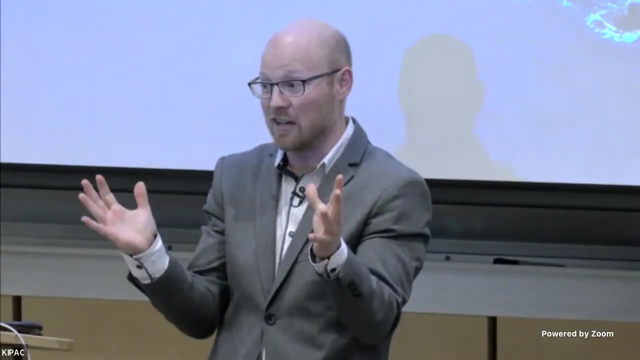 we can observe these photons we collect and these are known as the cosmic microwave background. it's the earliest picture of the universe we have a few hundred million years after the Big Bang, which is a relatively short time scale, and that is the picture that leads to why we call it cosmology, like we call it a big 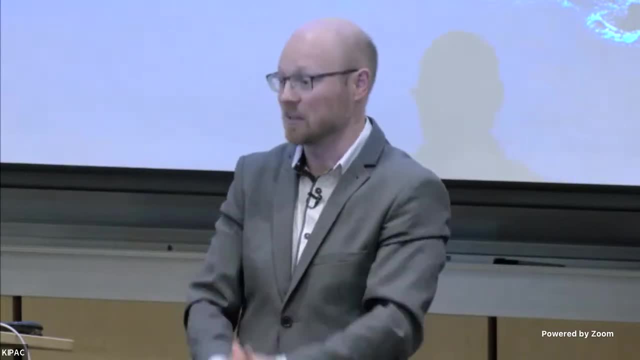 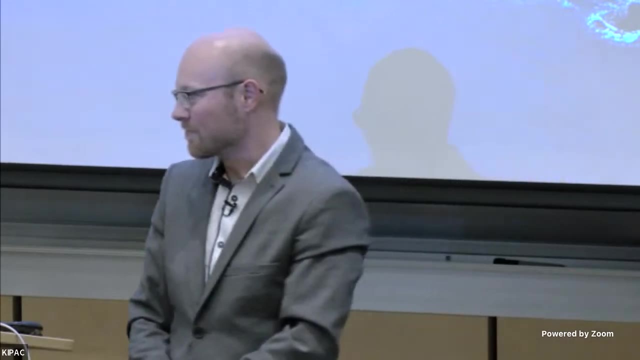 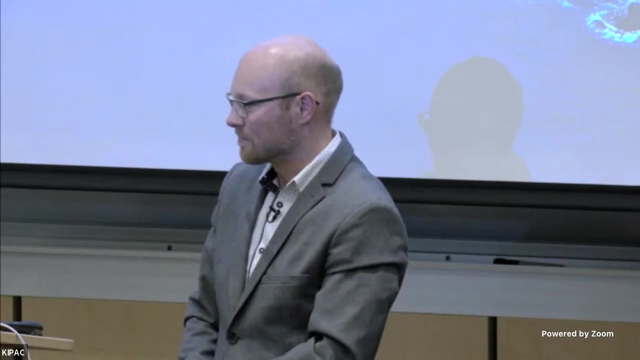 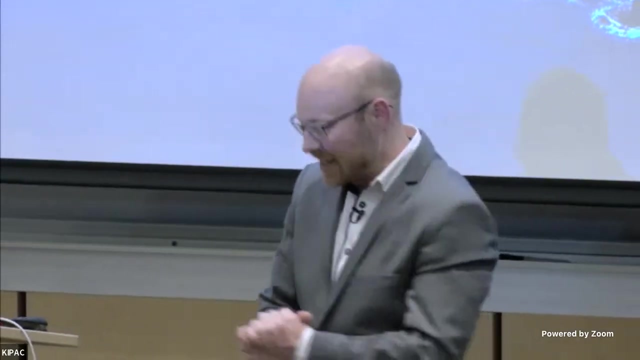 thing why we think the universe came from. basically one point, then expanded wonderful question, great over there. so yeah, why is the CMD in it? like? so essentially like noisy, like, why is this? uh, why did it vary so much? um it first this. it has a bit of okay. the question was why the, the cosmic microwave. 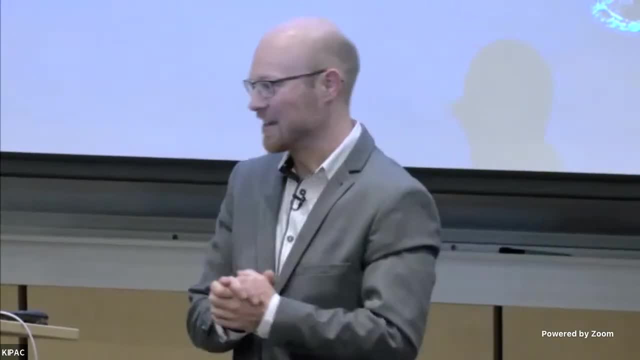 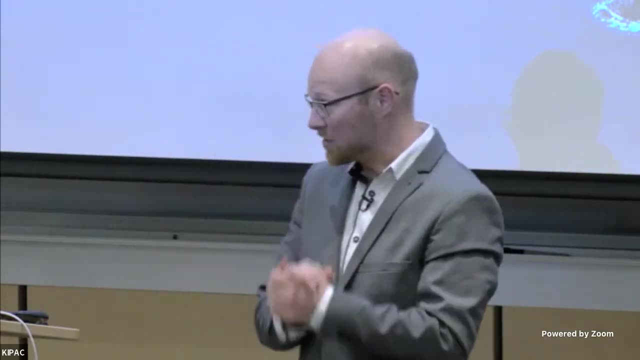 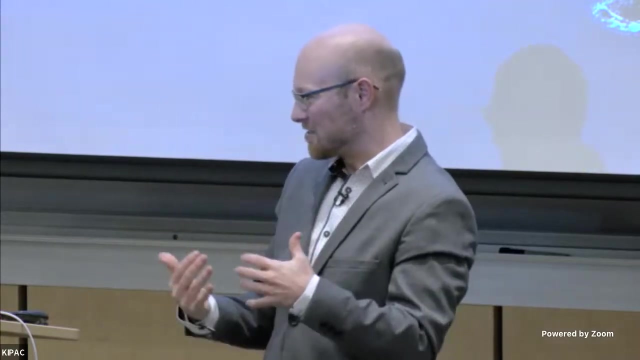 background image- this was one of the first top left images- is so noisy or wiggles so much um. so, first, it's not noise, it's actual signal that we see, and it's not so much it's the art or the, the, the person that makes the, the graphics that 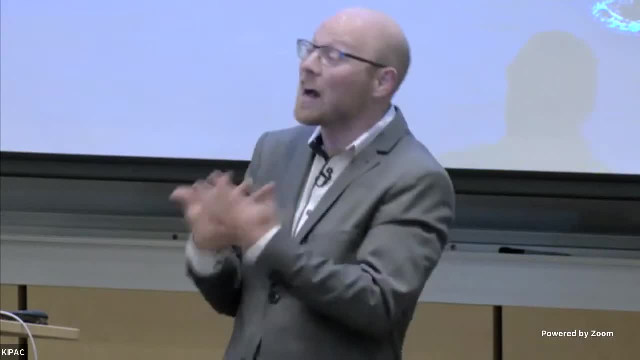 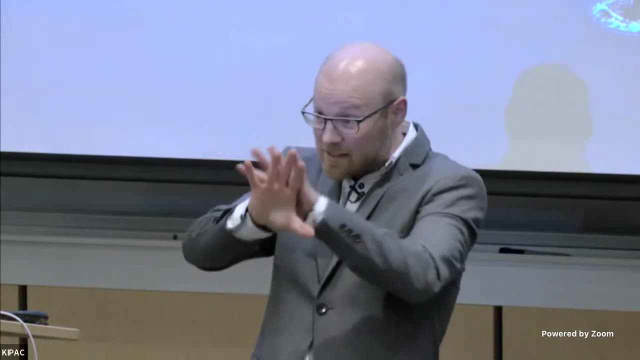 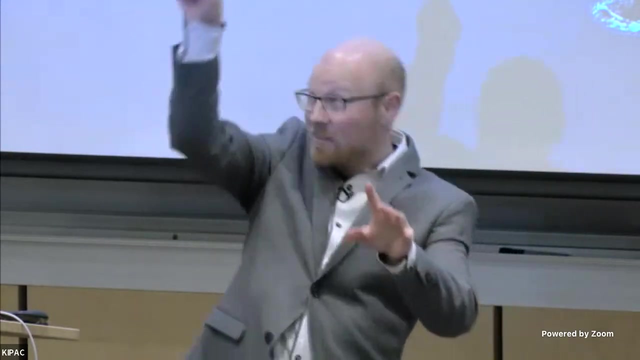 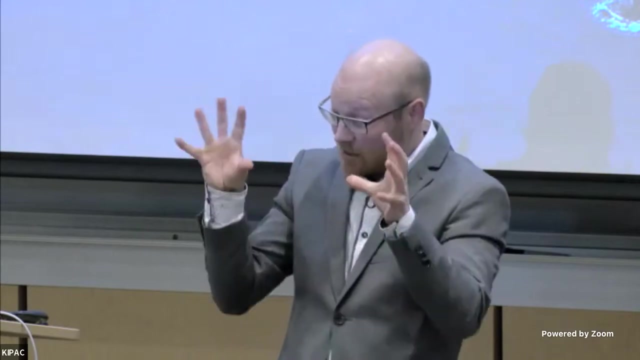 runs the signal. so this is one part in 10 000 difference between what you saw in red and in blue. so the universe was basically the same density and temperature, but just one part in 10 000, a bit more over there than than say, and like a degree next to each other and the signal. 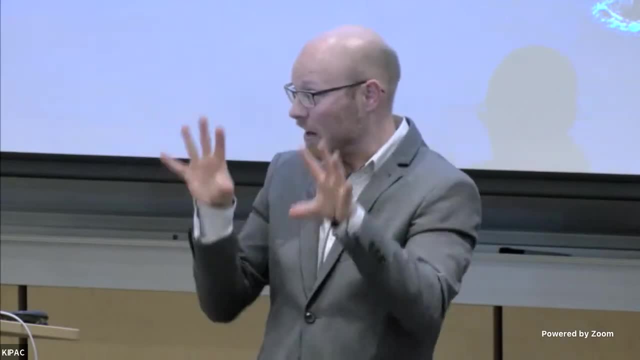 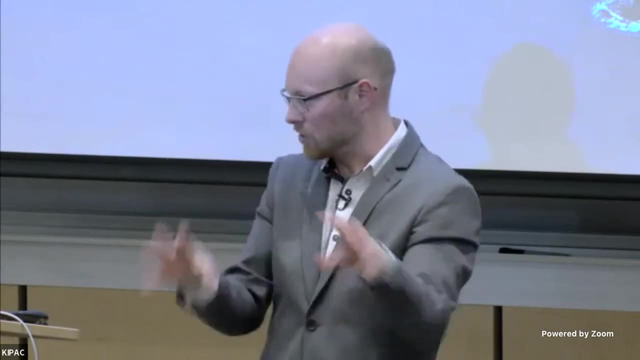 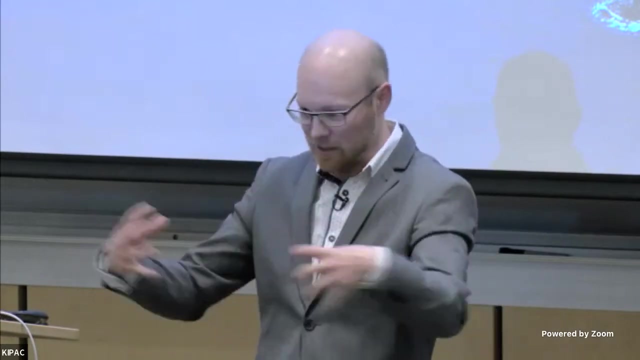 of this little differences are actually very crucial. so what happens there is? in the very early universe there were some density fluctuation. we don't know exactly where they came from. we assume it's quantum fluctuations in the where, your universe. that dictates uncertainty of where things actually happen. and once the 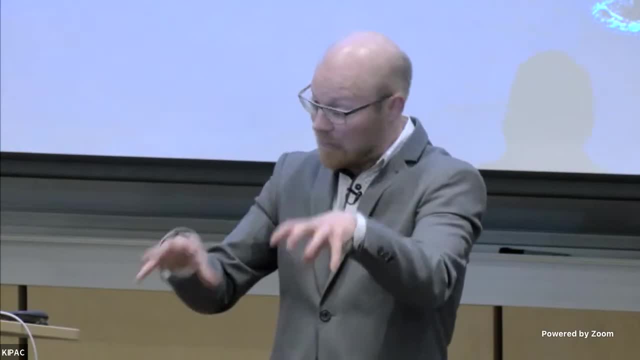 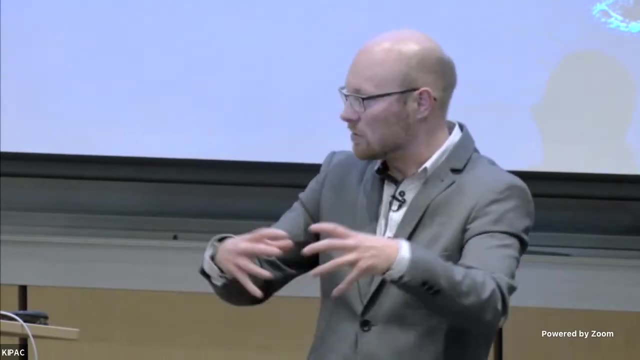 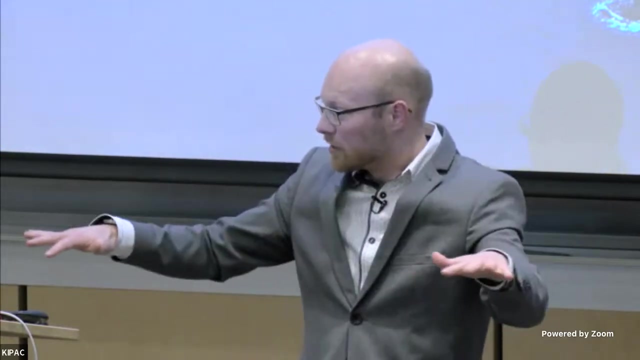 structure grow. they were imprinted and then what happened is that the plasma, the very energetic particles they travel in, or they have a sound speed, or things travel with a certain speed and if you let this structure evolve, this wiggles. they happen to be on certain scales on the sky. 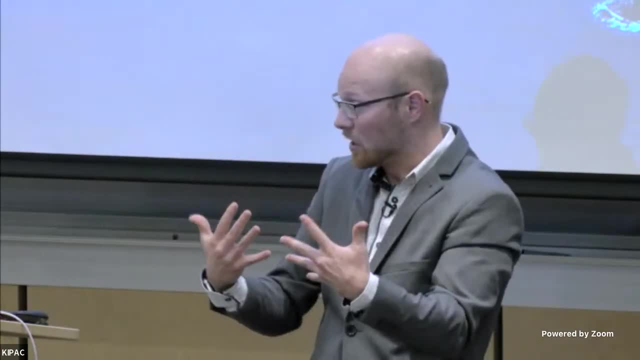 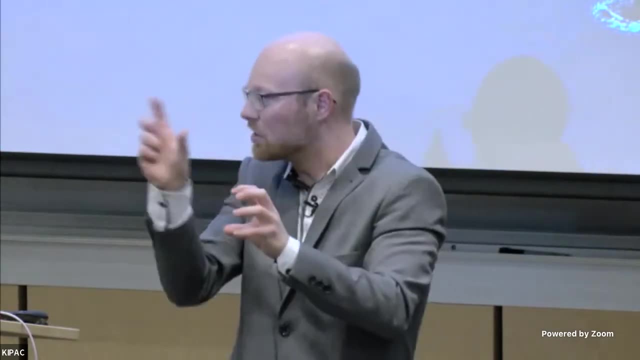 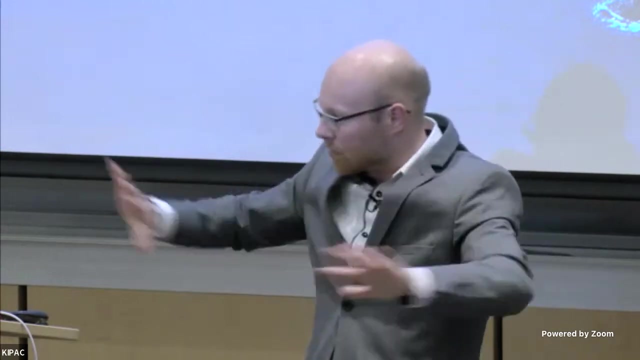 when the CMB. actually, we see it that the structure and these scales of how close a black and the red dots are from each other, which is about one degree, is according to that prediction of how this density fluctuations evolve and and go through that pressure is fluid, effectively plasma. 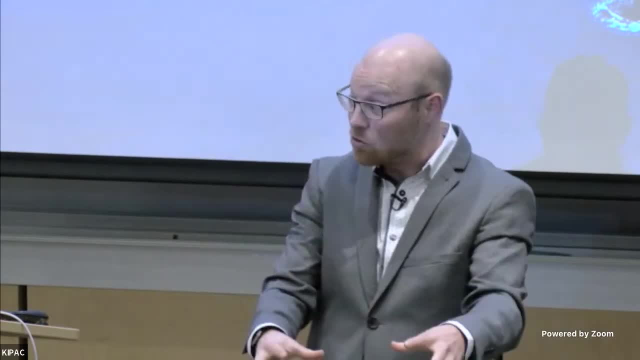 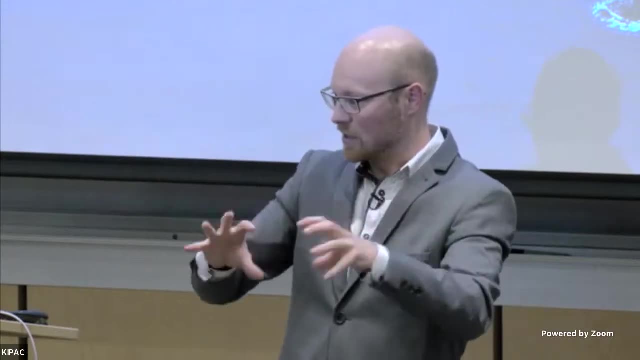 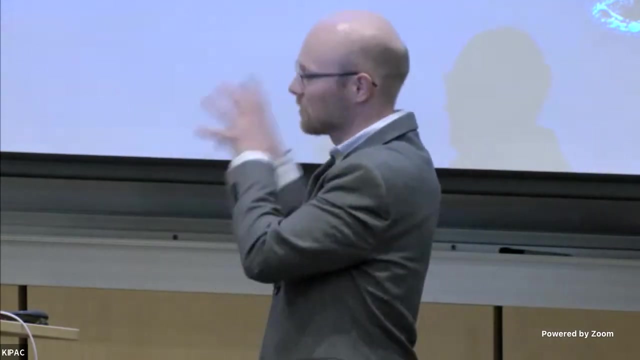 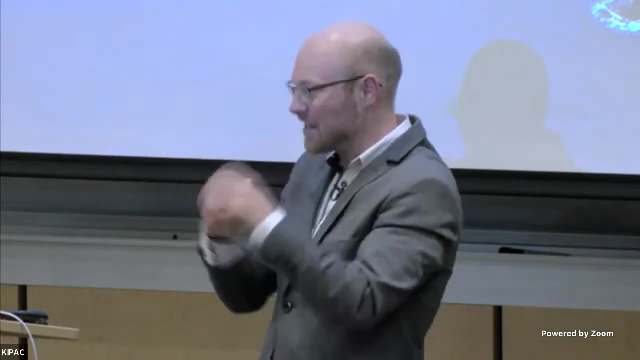 and so this ripples that you see there later grew into what we see as the galaxies, the cosmic web, the spider structure of these, and we can consistently trace the statistics of these fluctuations forward, and they are according to the expectation of where galaxies are around now. without this wiggles in it, there wouldn't be any life, there wouldn't be any structure, it would just. 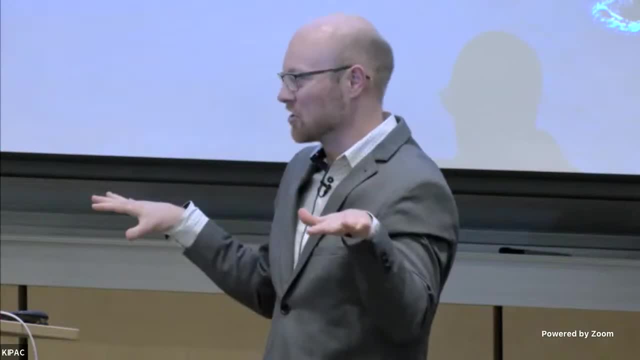 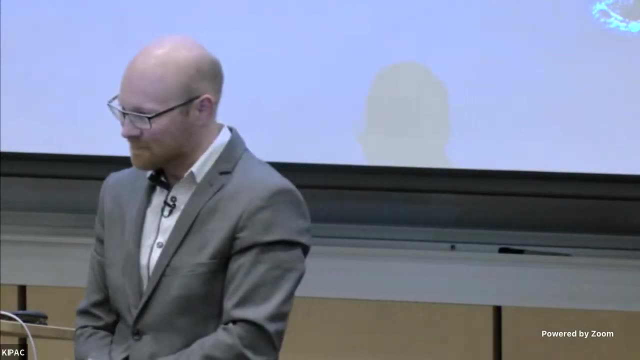 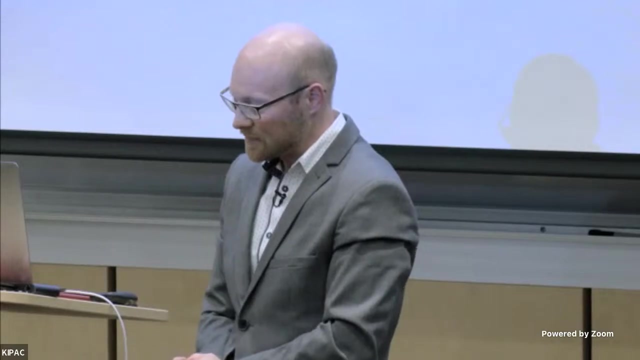 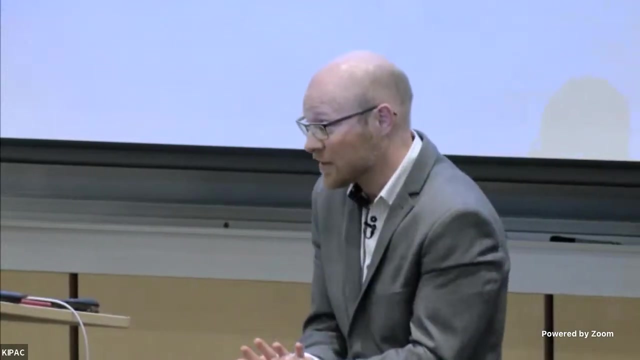 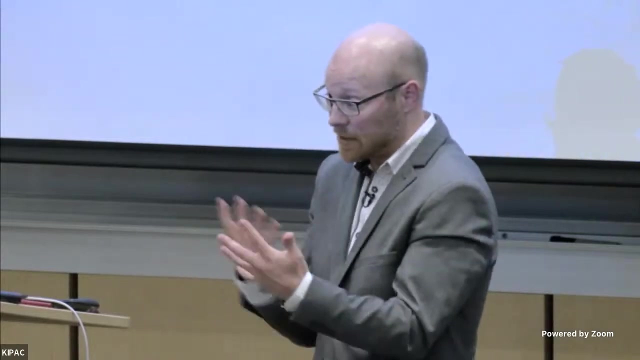 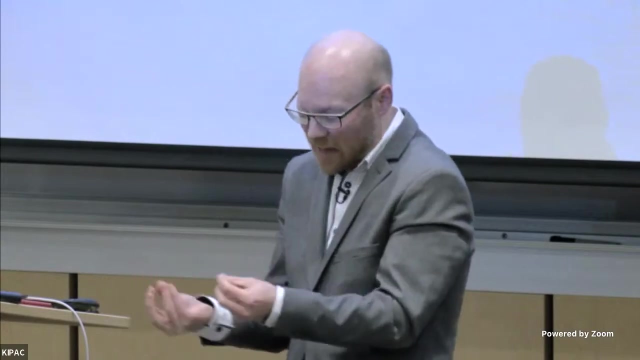 be boring flat. helium and hydrogen, nothing else great over there, um, and if we were to feel it with our hands, we could measure it and some and characterize it. the fact that we cannot measure it basically means that most likely I cannot feel it, so no one has felt it and measured when we can enhance. 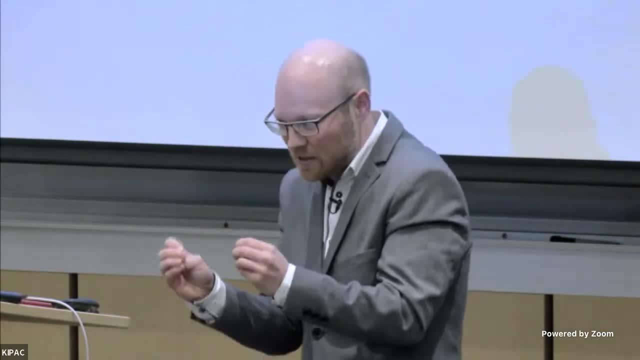 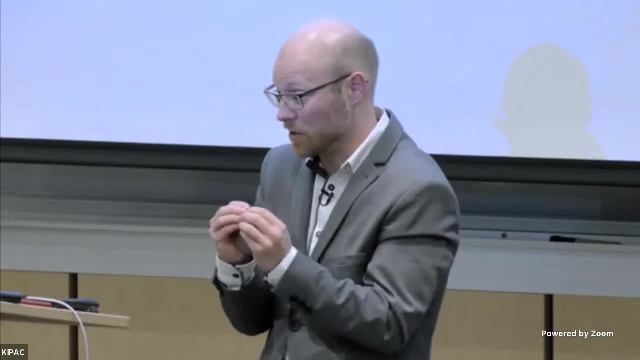 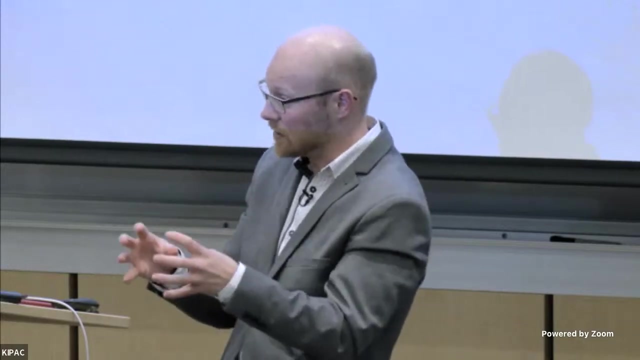 that feeling and be very, very precise and listen very careful of what's happening. we may find some hints of what it is, we may find it in one or the other way, but we have to be very, very careful and very precise. the nuances and that's basically the, the experiments that are being built on the ground. 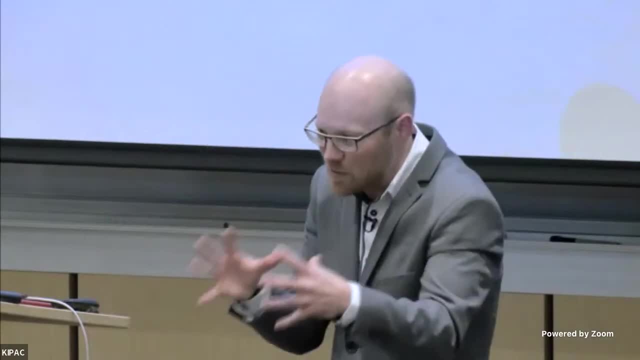 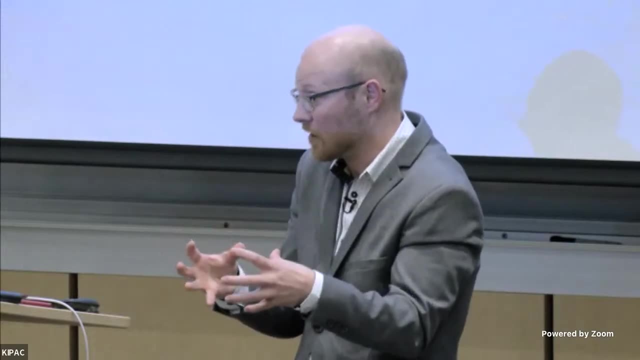 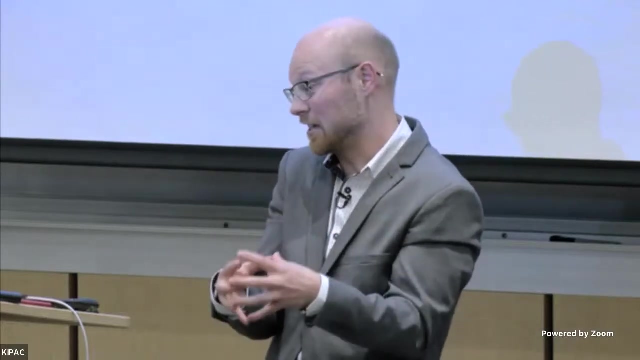 shielded from everything else and just listen basically to the sound of what a dark matter does something to that we didn't expect without it, And people are doing that very diligently for a long time ever- precise, And currently we only get. we just know what it is not. 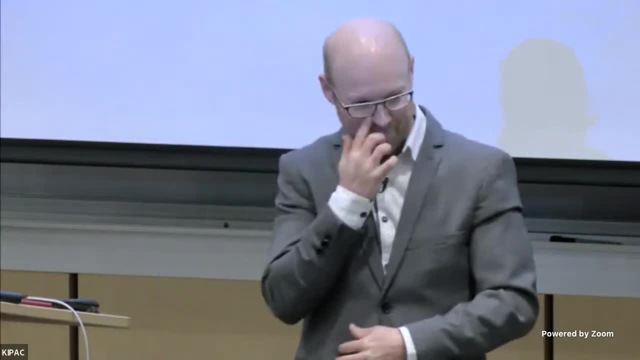 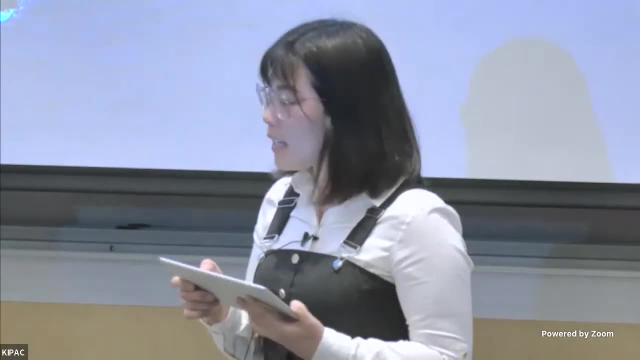 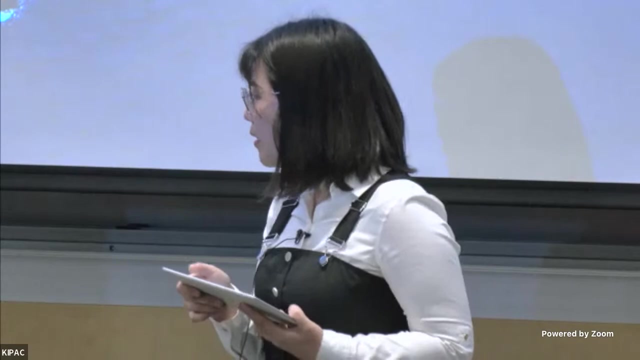 Yeah, There is a slightly technical question from our online audience, John, asking: is there a reason why JWST is unique for solving a lot of the questions that you have actually raised, For example, using the TRGB measurement, where you talked about the helium flash? 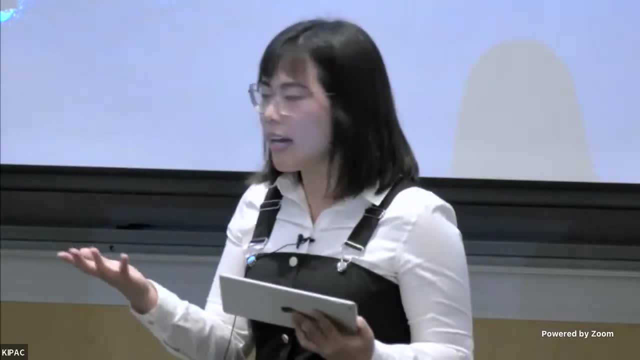 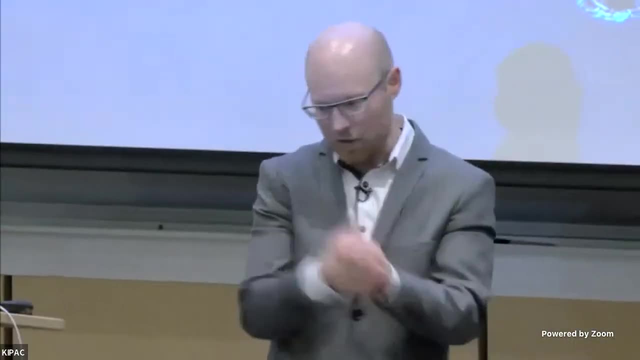 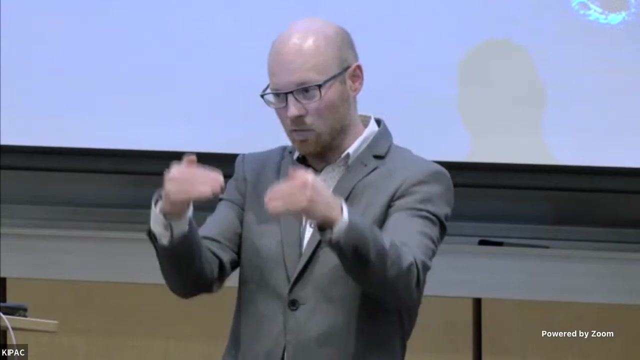 that's as part of the phase through stellar evolution. But why is JWST unique? And so the method has been used, in particular of the TRGB. so this method of measuring the Hubble constant, The currently available telescope, were just only good enough to give a measurement of that tip of. 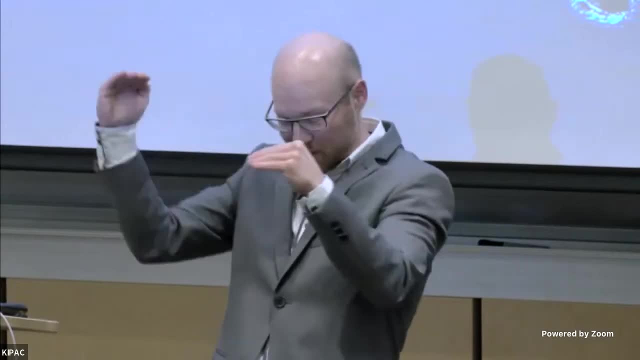 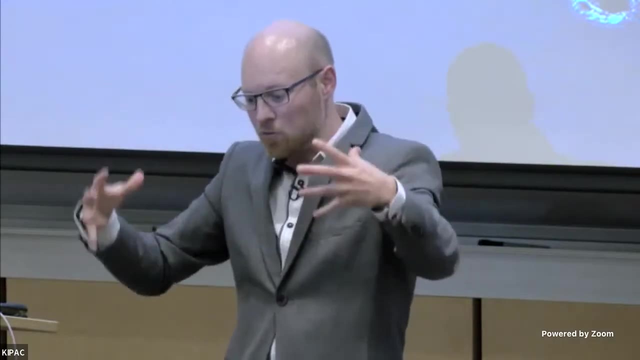 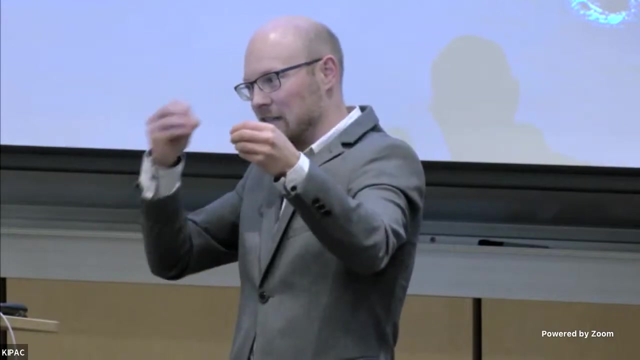 the red giant branch. so to find individual stars and measure where is the tip to a certain distance out in our universe- And there's just too few supernovas that went off- that leads to a good calibration And what the JWST does: it has the sensitivity to make that same measurement much further out. 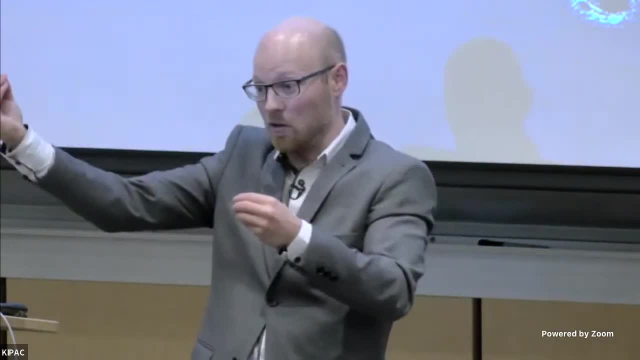 and in the same distance, And so it's just too few supernovas that went off. that leads to a good calibration. And what the JWST does- it has the sensitivity to make that same measurement much further out into where we have a lot more supernovas already went off that we have in our pockets from. 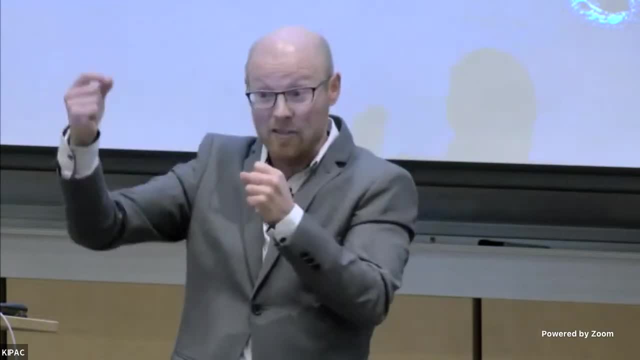 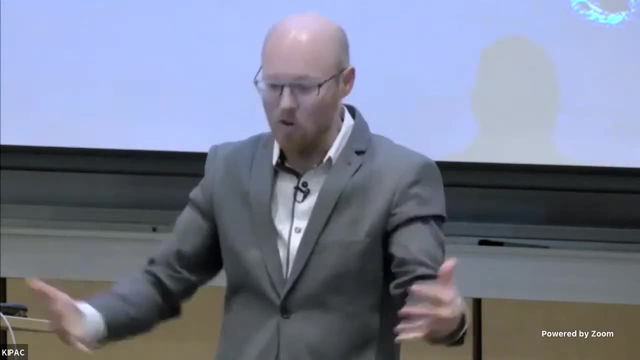 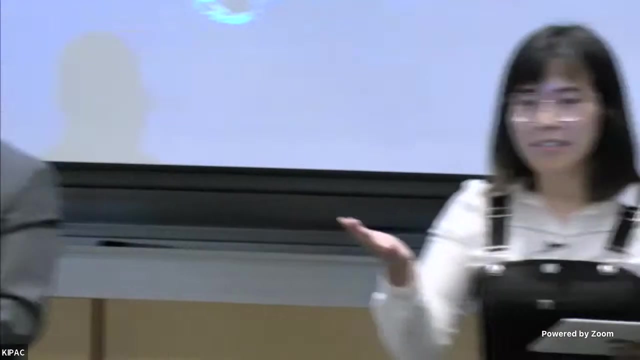 the last decades of observations and where we expect also many more to actually go off and observe. In that sense it opens up a much broader window in the sky. Great Well, I know we still have a lot of questions from the in-person audience, but Simon is not. 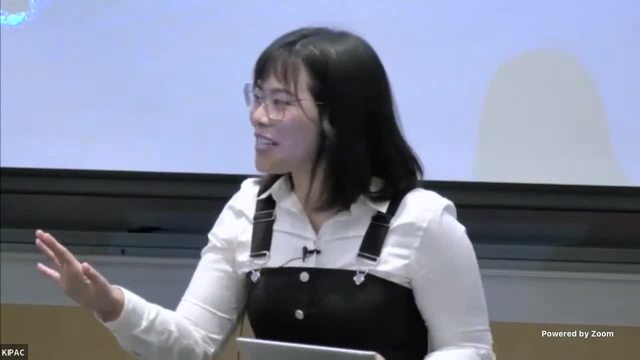 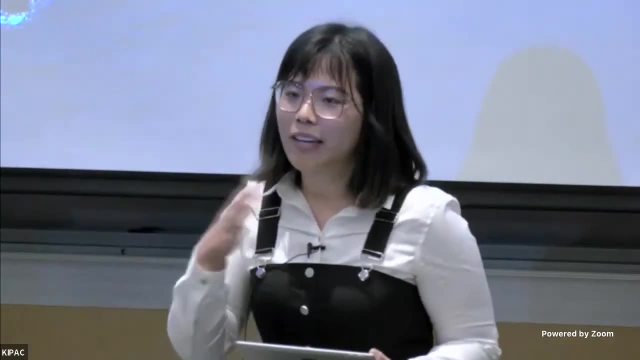 going home until he's answered all your questions, And also since this is well and certainly, your last week physically at Stanford, right, So we got a need to take full advantage of his presence, So let's thank Simon again. Thank you. 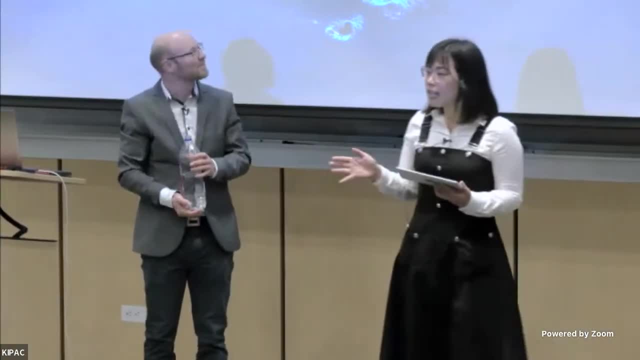 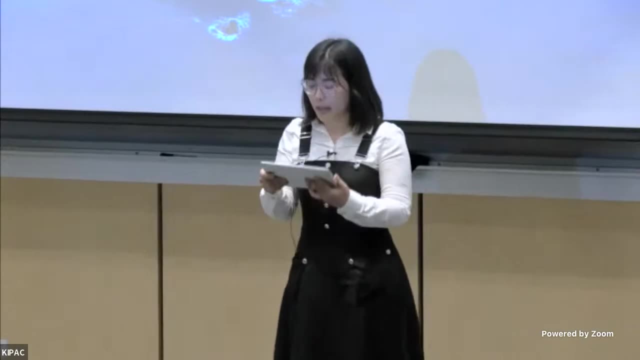 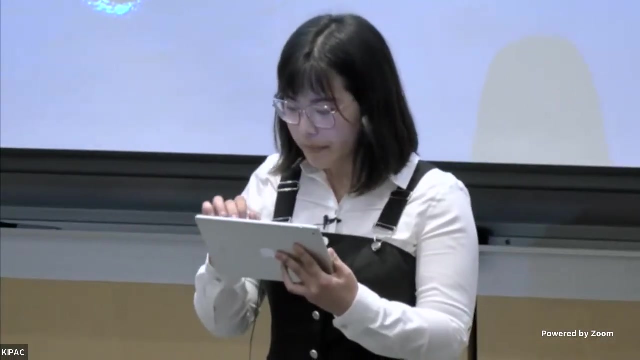 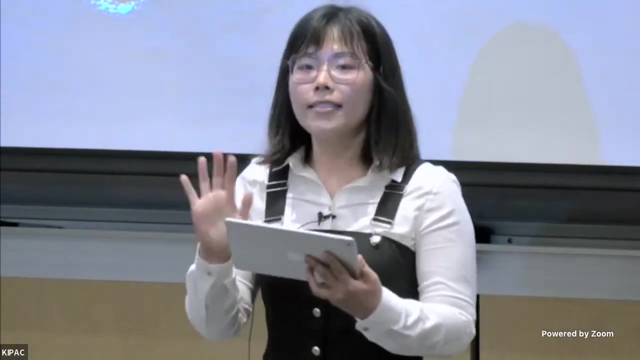 And before we wrap up, I would like to quickly just introduce a few ways to follow KIPAC. If you have enjoyed this lecture and wanted to also tune in for our future lectures, So let me just quickly start sharing screen. So we actually have a lot of different kinds of social medias, as all the other organizations. 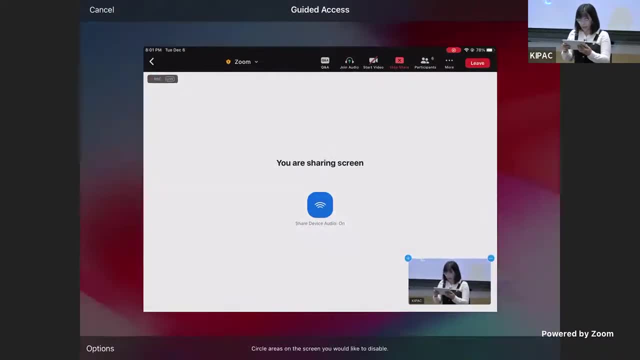 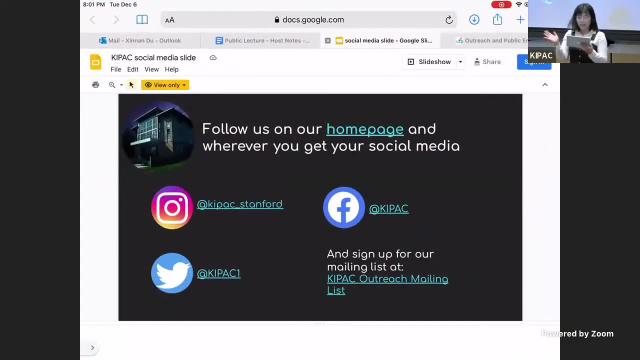 might do. For example, we have here Here Great. Okay, So you can see that we have all these social media platforms For an online audience. you can actually see the URL will, which will be dropped into the chat. These are the ways to follow us. 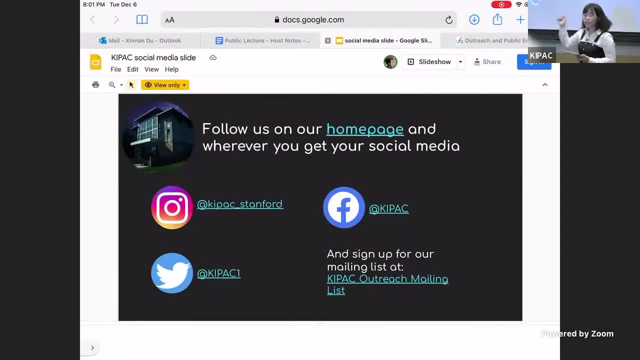 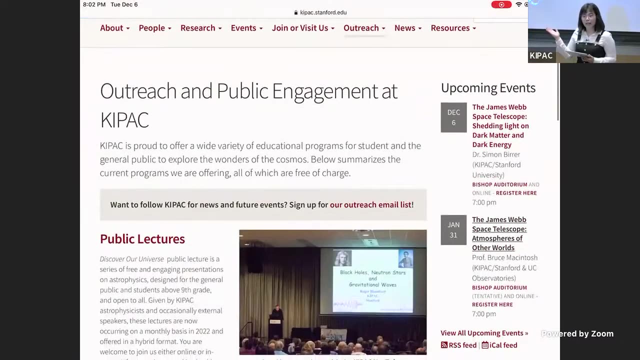 We have Facebook, Twitter and also Instagram, So all kinds of things, And especially if you're interested in hearing the third lecture in this series, I would also recommend That. And then you go on to our outreach page, which is simply also on the social media slide. that. 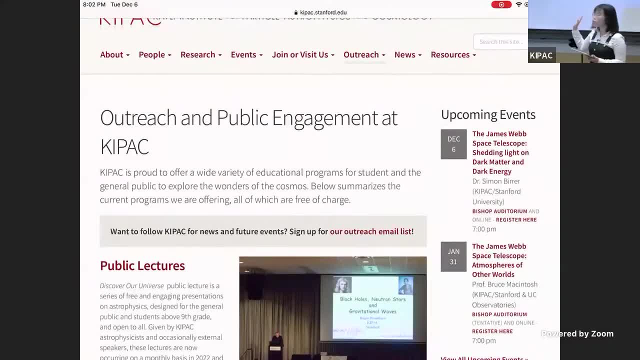 you have. So on the right you can see, we post all our upcoming lectures: This one that just happened And also the January 31st, where we will have Bruce Professor, Bruce McIntosh, who is an exoplanet expert, to talk about how JWST will help us better understand and characterize. 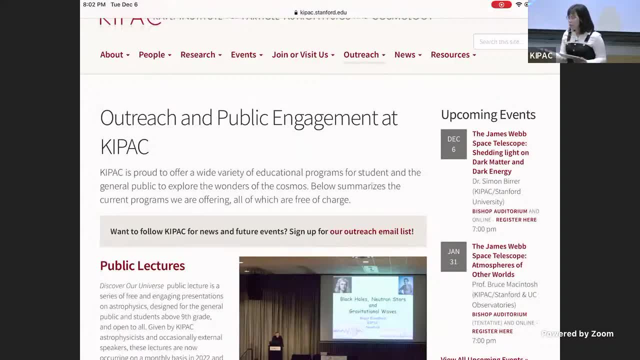 the atmospheres. Okay, So we're going to be talking about how JWST will help us better understand and characterize the atmospheres of all those planets That's orbiting other stars. So it's going to be slightly different from what we have already talked about, but it's.